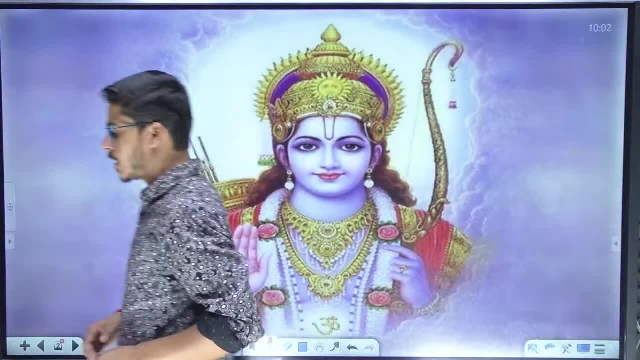 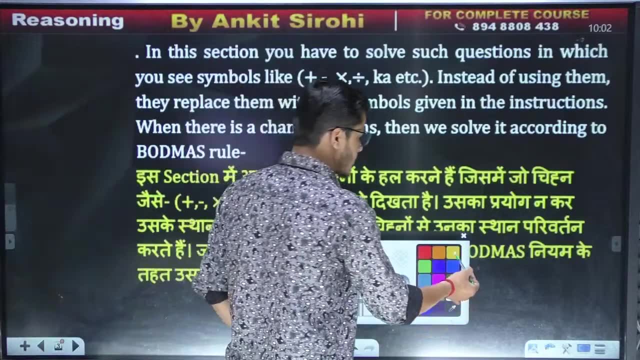 What will happen, dear friends? see, come quickly. Dear friends, first of all, let's go and understand about whom our chapter will be today, Which you must have seen, dear friends, and about whom it is. Here I will talk about mathematical operations. 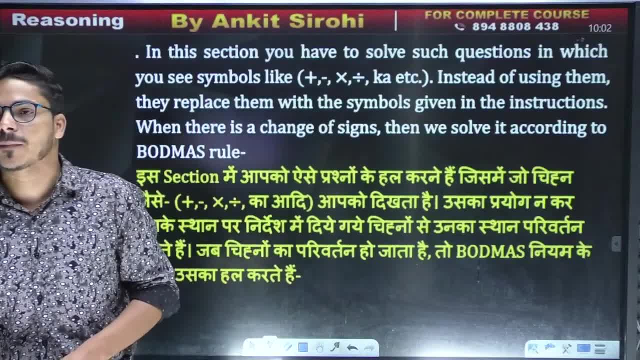 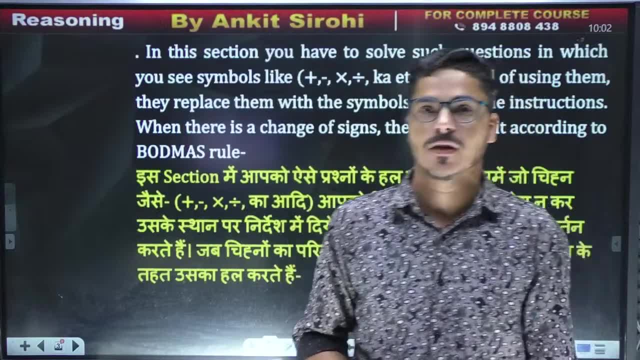 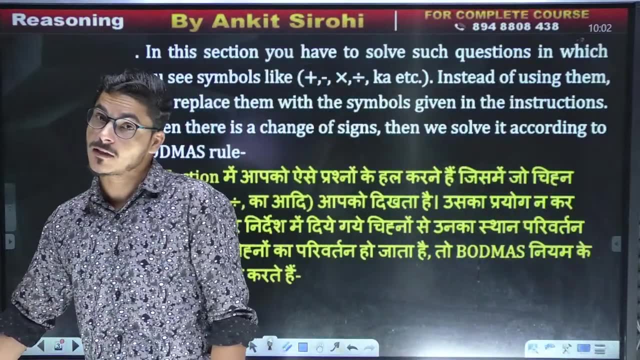 Dear friends, whose Mathematical operations, dear friends, Which we all know in the form of mathematical operations, It cannot be that the question is not asked in the exam from here. Okay, And dear friends, remember this, And if the question comes and you cannot do it, we will not let it happen. 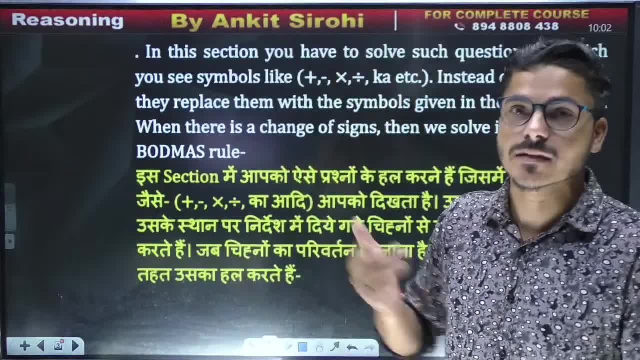 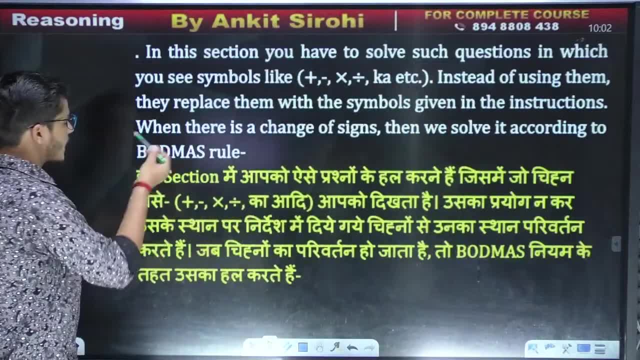 It cannot be that the question is not asked, And if the question is wrong, we will not let it happen, Okay? So, dear friends, come on, let's go very quickly. Dear friends, in a simple way, Brother, see what will happen here in the end. 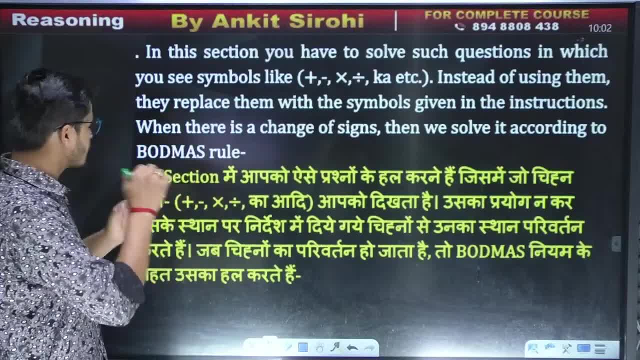 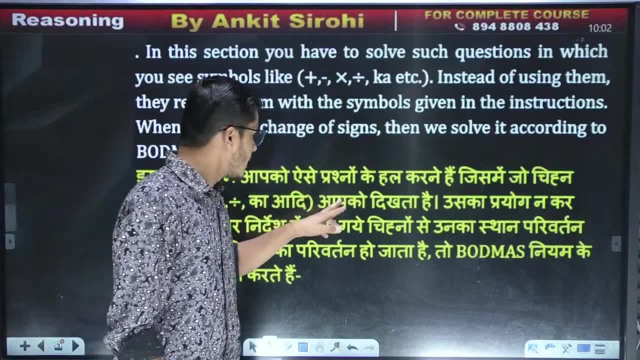 In this section you have to solve such questions In which, for example, the sign is plus, minus, equal part, etc. etc. etc. You can see, Its application is to change the position of the signs given in the instruction instead of it. 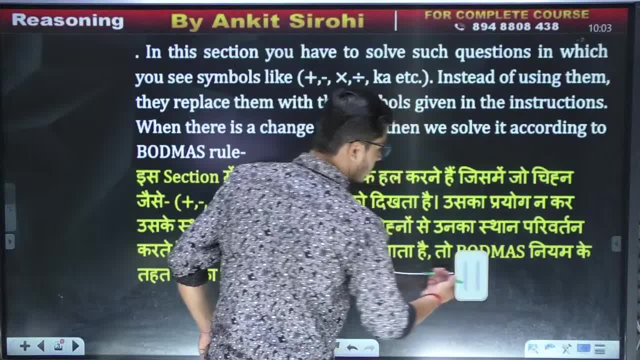 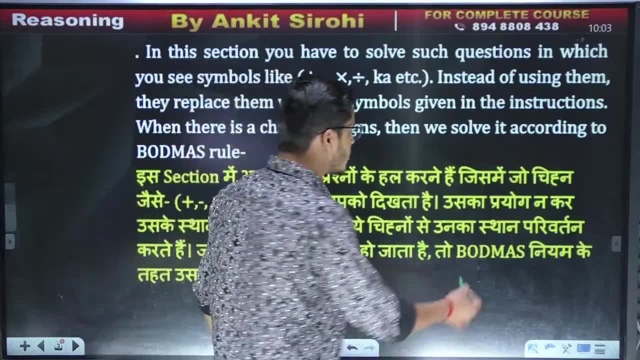 When the change of the sign is done, dear friends, we use the rule of boat mass If I talk about its Ramban. What will be the Ramban method, dear friends? First of all, that will be In which my dear brother knows, the boat mass. 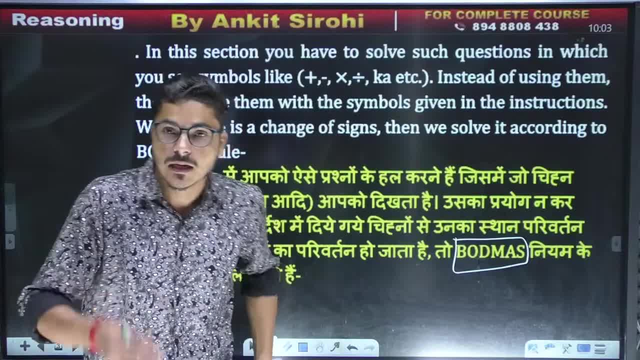 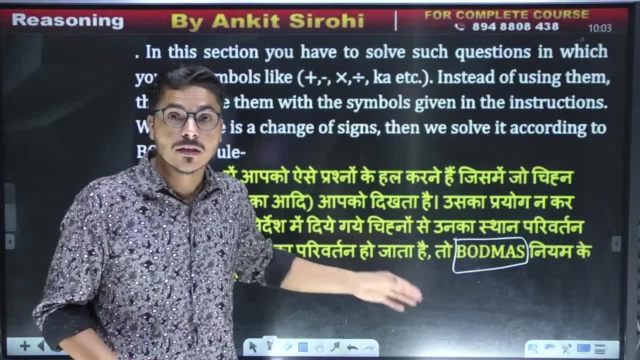 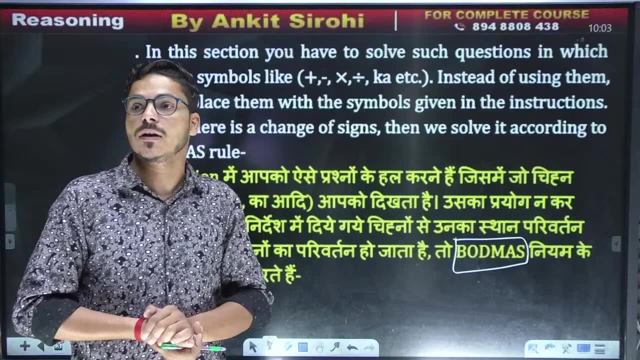 The boat mass rule that follows is the strongest Brahma master, Because, dear friends, there is nothing without it. Understand this. Without it, this chapter is like a bullet without a gun. Okay, It will remain only to be shown. And, dear friends, if anyone attacks, then you cannot run it while coming to your safety. 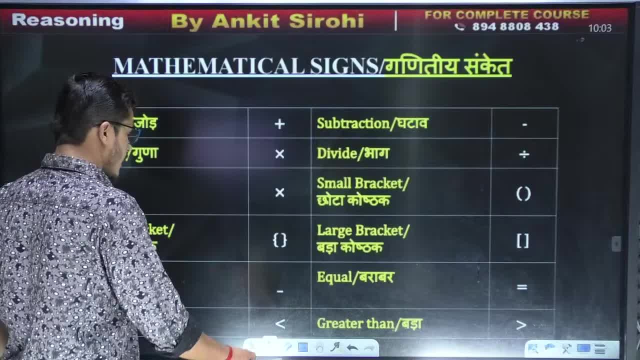 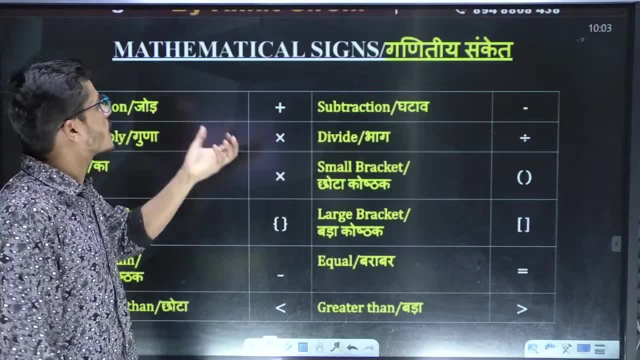 Let's go. So now here. first of all, let's know about the mathematical operation, Brother, after mathematical operation. See here Now, dear friends, there is a mathematical operation, We have mathematical signs. Mathematical, There are mathematical signs. 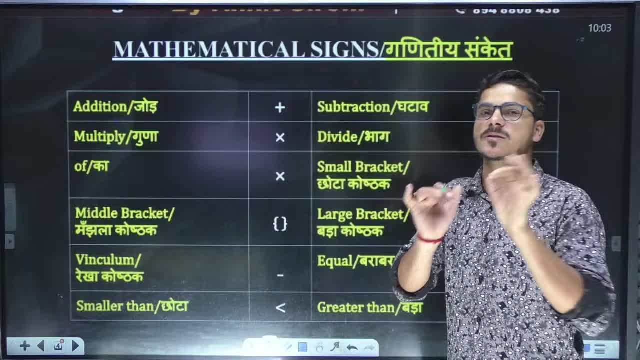 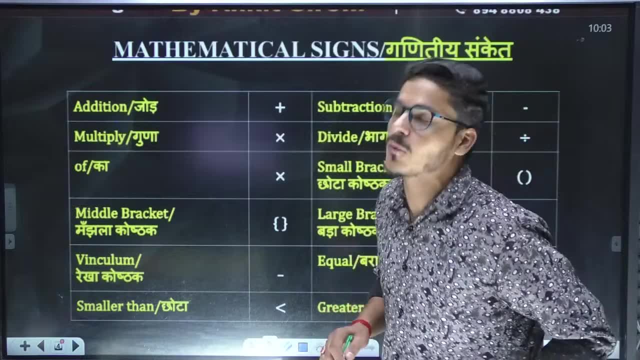 Absolutely, dear friends. Means Now see that you understand what I mean. Only here. first of all, everyone should know what it means, Although we have learned all the things in childhood. Okay, very good, You know a lot, Very good. 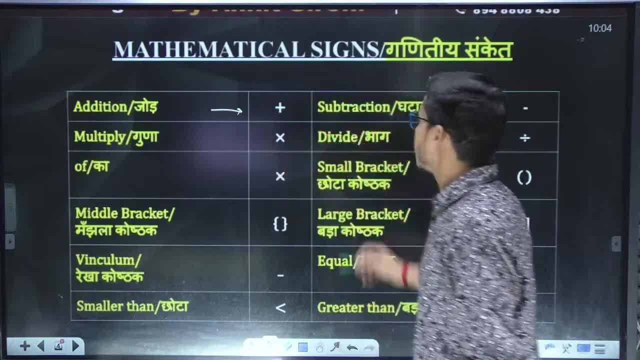 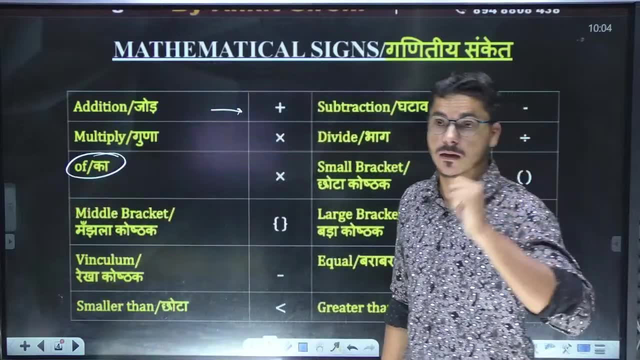 See, This is brother joint. This is called plus. Okay, What does it mean to multiply it? Or what does it mean Whether it is off, or what It means to multiply. What does it mean To multiply? Come on. 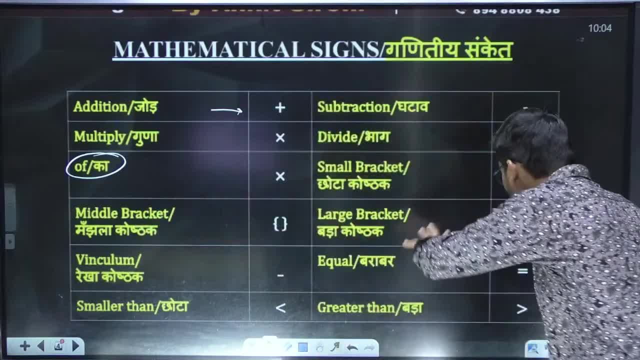 Let's see here, Let's go ahead. All the other things are in front of all of you. If you want to take a screenshot, you can take it. If you want to understand it in your eyes, then you can understand it. 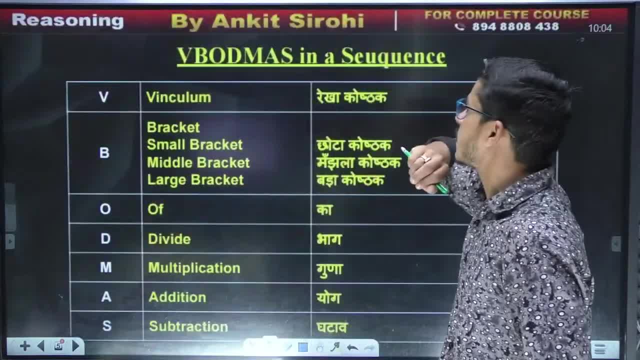 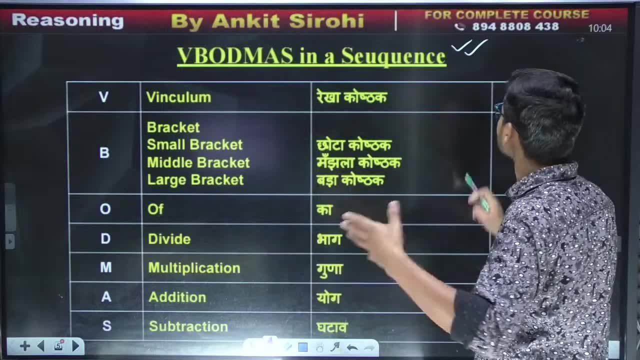 Dear friends, All right, Come on Now. let's talk about this V board mass sequence. Please understand me, Dear friends. The squeeze of this whole chapter is here. Here is the pyramid. Who has come to apply this? If I say squeeze, then it is here. 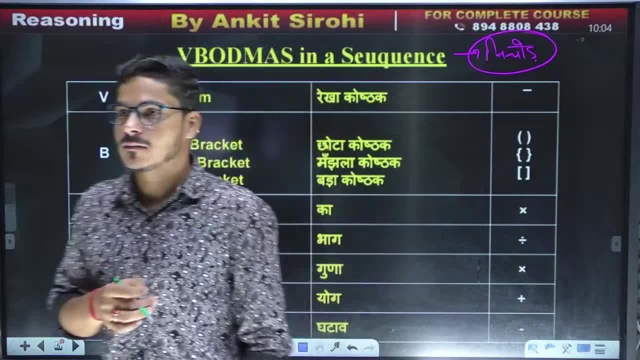 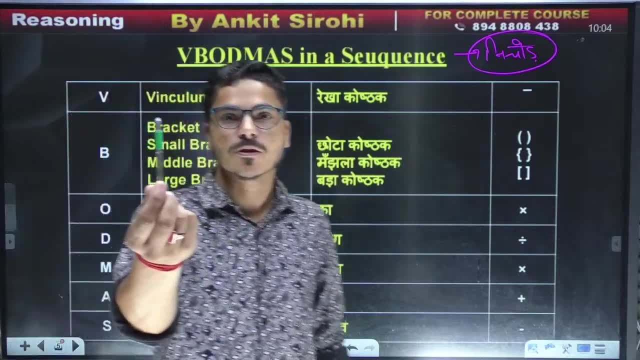 There will be nothing wrong in it If the person who has come to apply this Okay, Without the operation of the cheek, Absolutely. There is no need of the cheek. Dear friends, Here is our cheek And you will have to do the operation first. 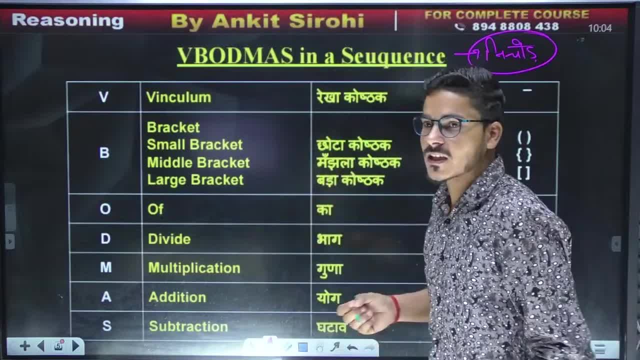 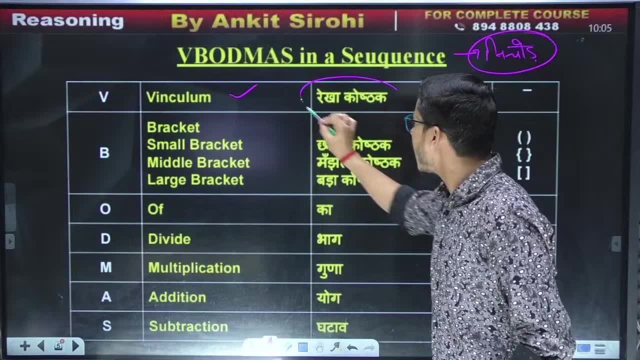 Whose question is it, Isn't it? You have to make a peacock by doing the operation. Okay, See Here. dear friends, Good morning brother. You will see. Now you have to understand me. Dear friends, This is called the first line. curve on you which you call a bar. 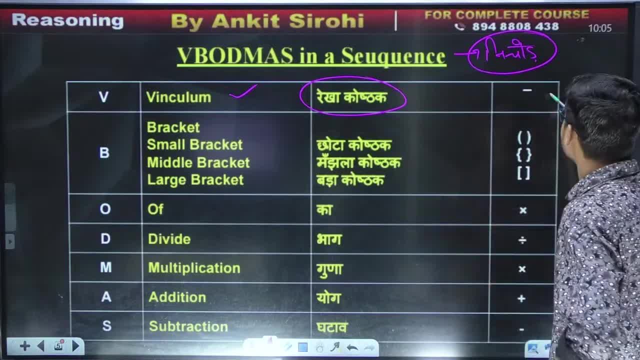 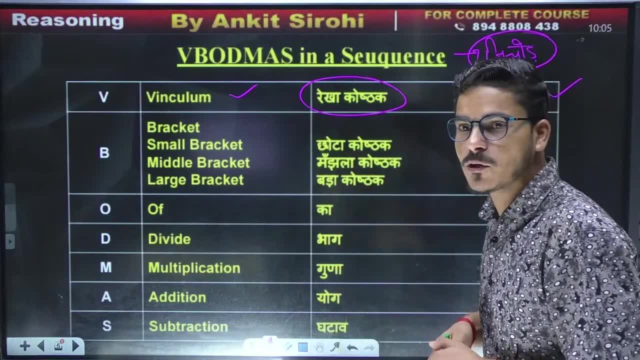 Here it is. The teacher does not say that you should reach there Bar. First of all, we solve this, After that we start, We move forward, We move forward, Brother, Brother. Now I have been in the class and it is still going on. 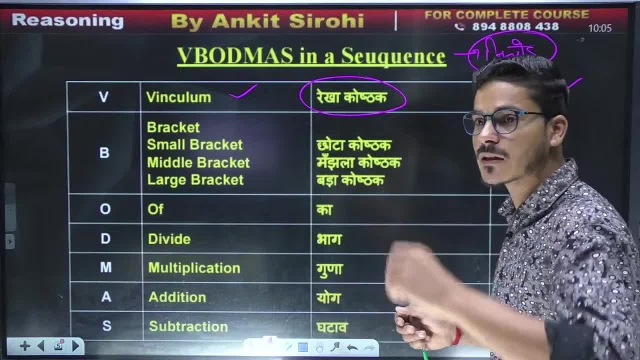 What happened like this? What happened like this? Questions will come, Do not worry, Come, It is the turn of the question. by explaining it, You will see in front of you. Now I will talk to B Friends. B is bracket. 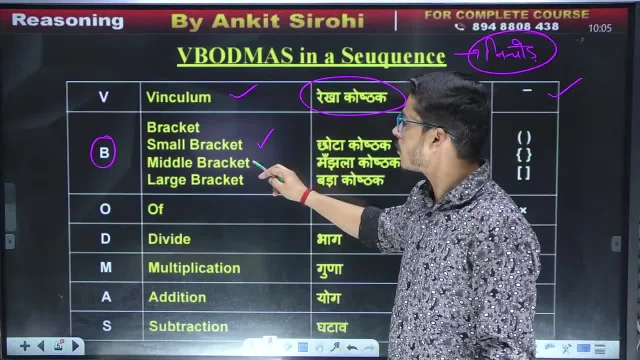 Which bracket will be small? It will be middle And then, friends, it will be a large bracket. That is a small bracket, A big bracket Here. everyone is in front of you. What does the meaning of off mean? It means that the line is a small bracket. 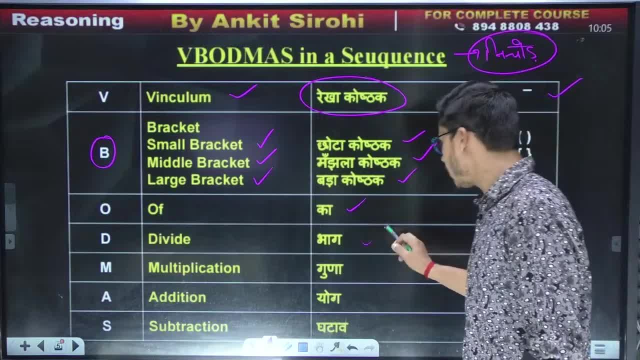 The divide will be a divide. Lack will be large, There will be yoke, There will be decrease. What do you mean by friends? Friends, this is a REVERSE. First of all, we will use the V. When we ask, we will do V. 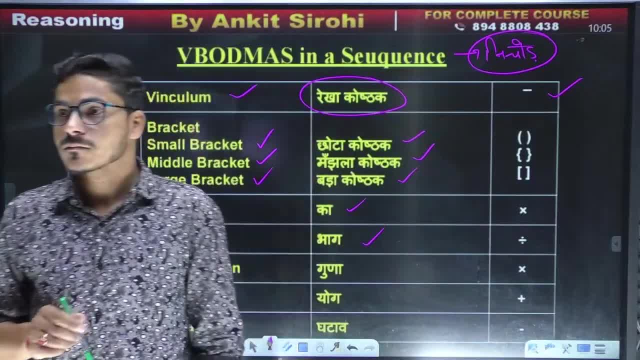 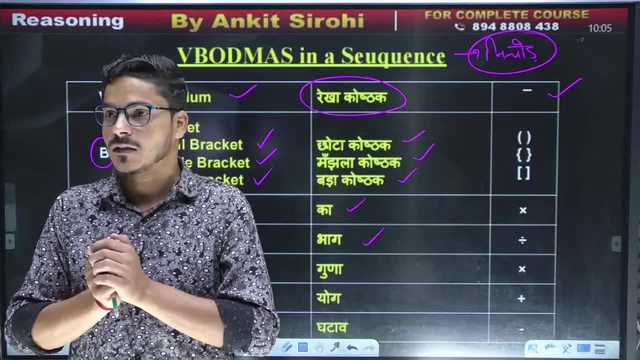 There is something written in life that having won thousands of fights in life is better than winning victory over yourself. If I win victory over myself, then the victory will always be yours. Very good, Very good. Now see what will happen now. friends over here, this is the first REVERSE. 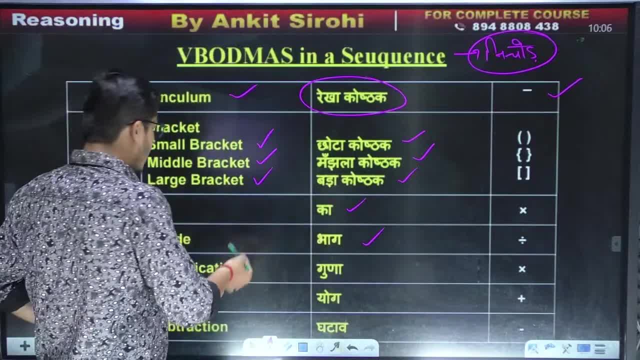 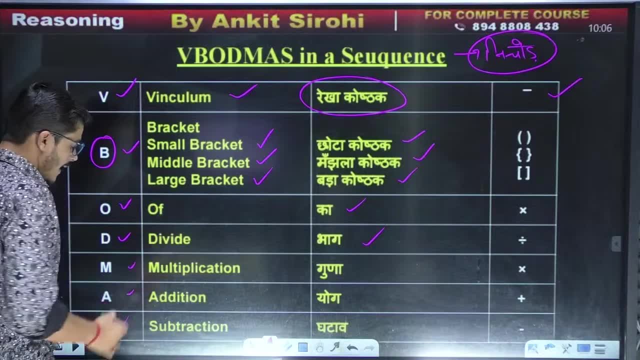 First listen to it first. This is called a REVERSE When we speak about self-reliance. Okay, Everyone is listening. What is this? Then follow this and then follow that. Keep climbing the steps like this. And, my dear friends, this is a step on the basis of steps. 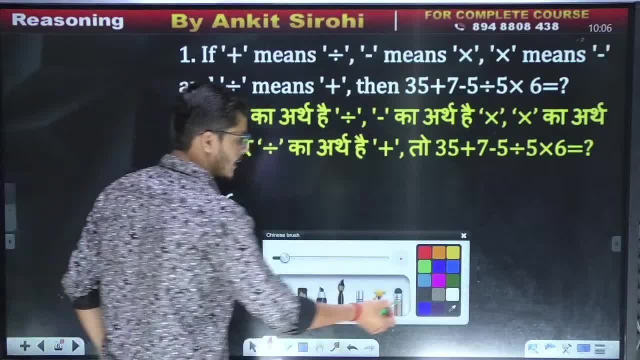 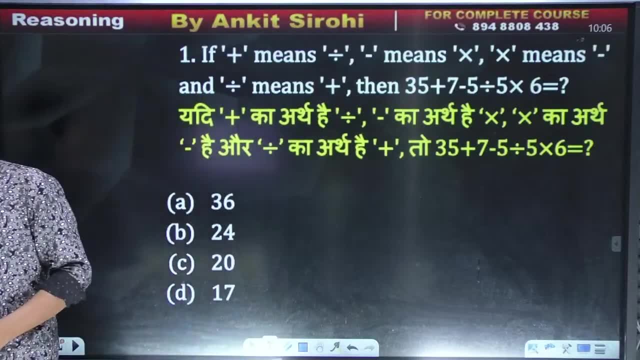 Okay, let's go. My dear friends, the first question has come in front of you all. The first question is posting its presence. Let's see which of its dear friends will give the correct answer. Which of its dear friends will give the correct answer. 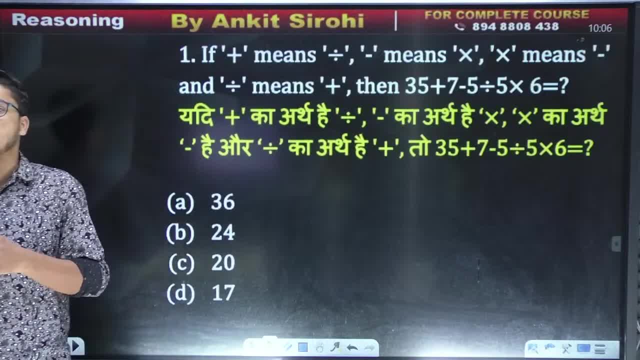 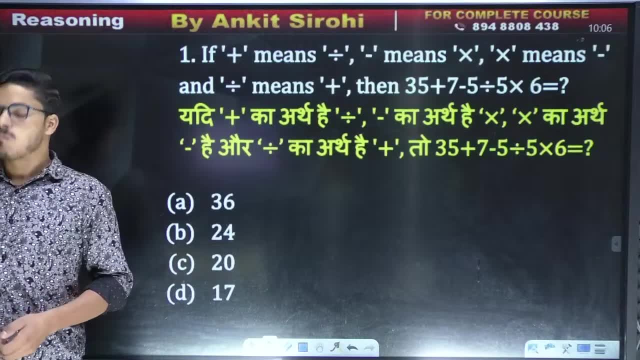 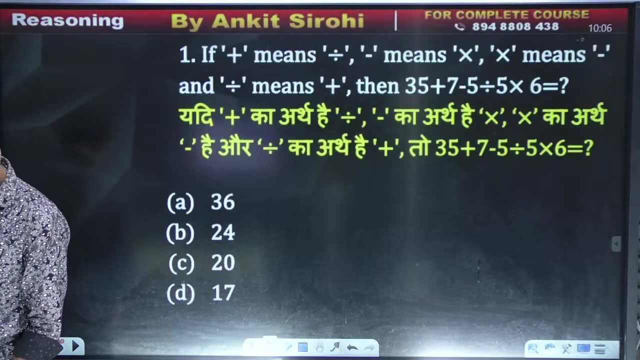 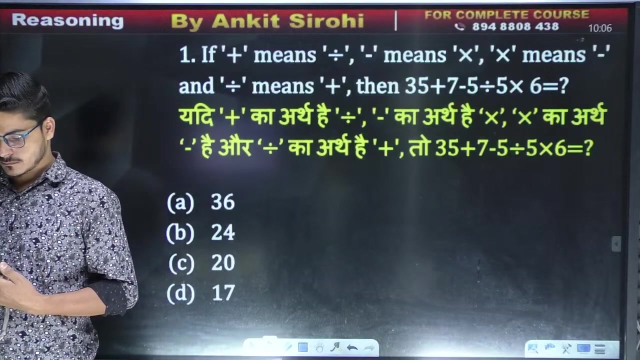 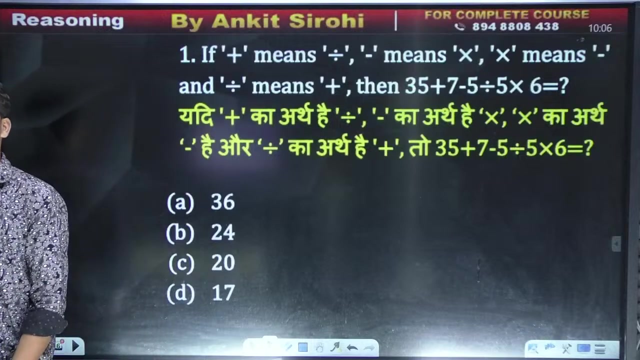 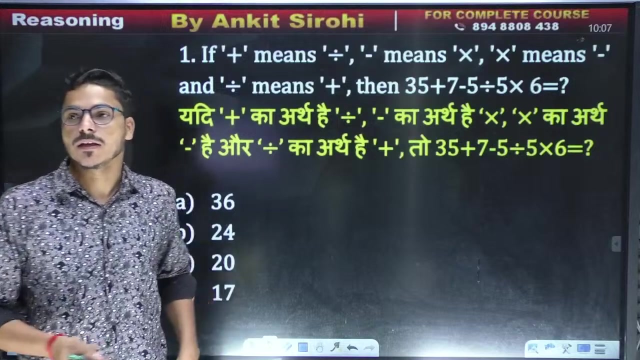 Friends, first of all, tell me, brother, what is the correct answer of this. Dear friends, please tell me quickly. Okay, tell me quickly. Let's see. wait, come on. See, friends, come on 24, whose name is it? 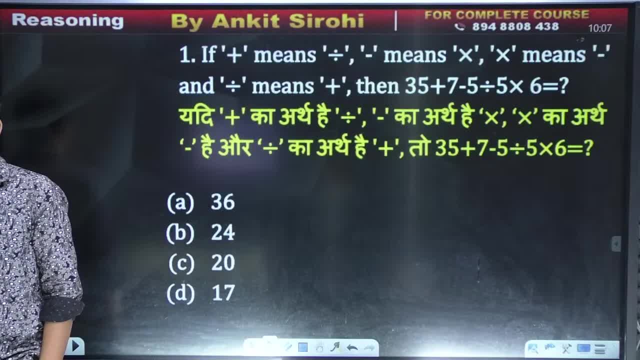 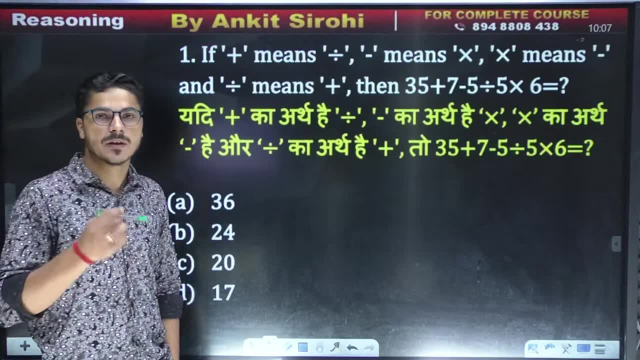 It is Kamya, right, The name is also written in this way. I don't understand. Twenty-four, twenty-four, twenty-four, Friends, how much twenty-four do you all have? See, first of all, my friends, what do we have to do? 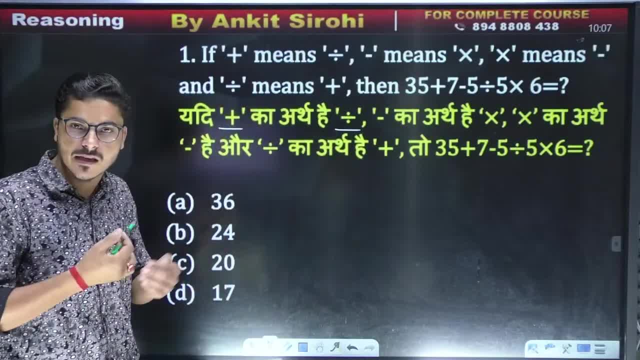 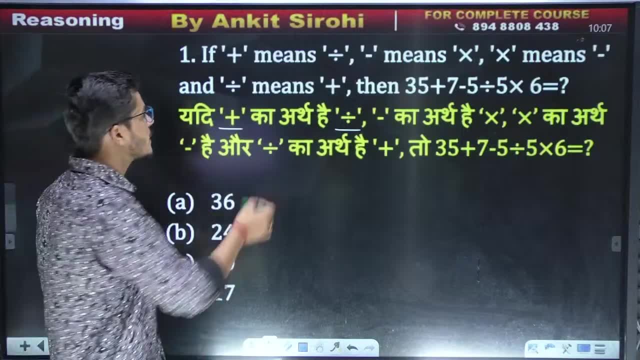 Here, every sign, what does it mean? My every sign, every sign, every sign means something else. For example, plus means part. What is it? Plus means part? Here it is given. plus will mean divide and minus will mean multiply. 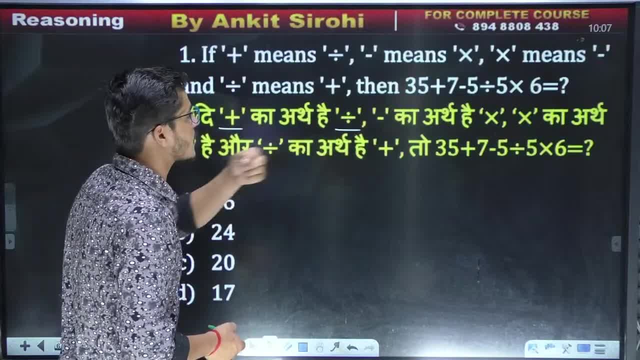 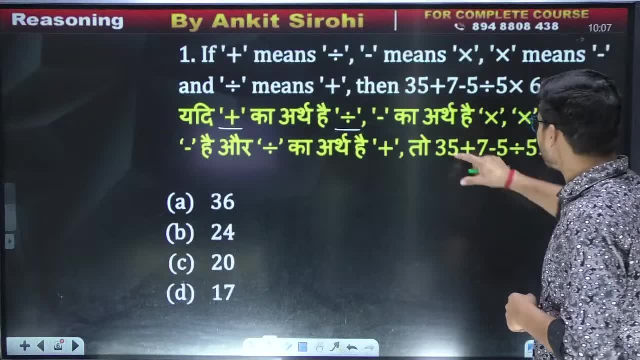 multiply will mean minus and divide will mean plus. This whole thing is given to you, So if you are my friends, if you do this, then your result will be wrong, Because here there is a change in all of them. What is the change? 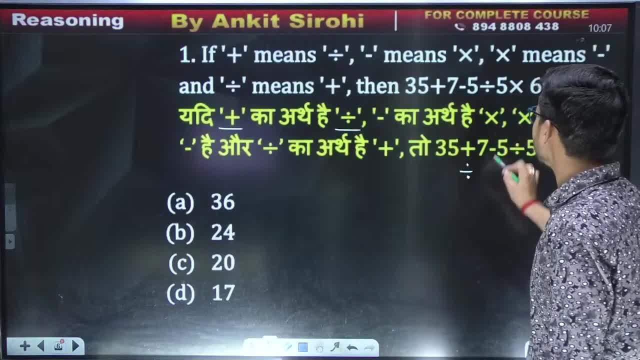 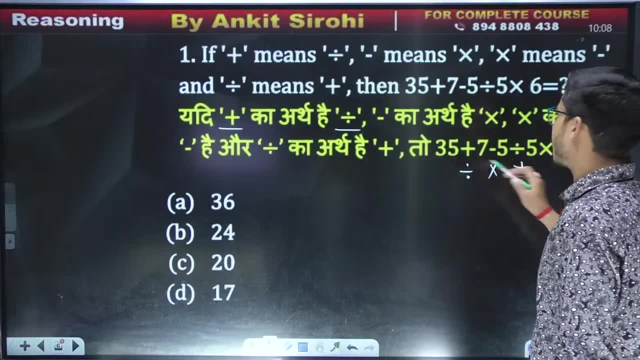 In the place of plus. the meaning of plus will be division. Okay, Parishati, There is a minus: my brothers and sisters. Minus will mean multiply And the meaning of division my friends will be plus And the meaning of multiply will be my Parishatis decrease. 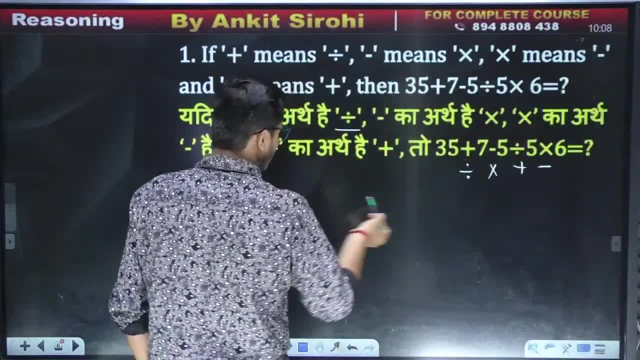 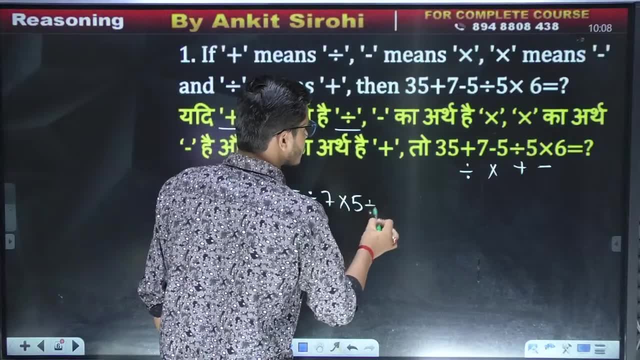 Now, using these signs, we will write the equation here. So he said: let's write the equation. So the equation is 35.. Divide by 7, multiply by 5, plus 5 and minus 6.. He said: okay. 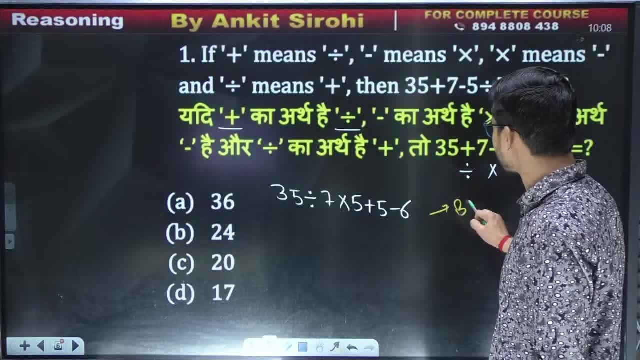 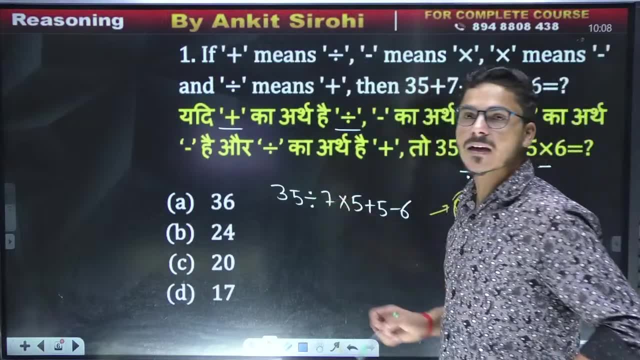 The rule of the board mass says that, using the rule of the board mass, we will walk. So, friends, first of all, B O is over D, mass is remaining only here. Divide, multiply, add or subtraction. First of all, we will divide. 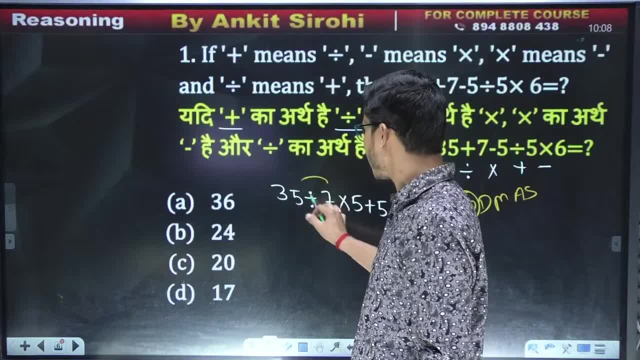 He said: divide it. So, my dear friends, first of all, you will divide this, You will divide it. So he said: divide 7 by 35. How many times is it gone? 5 times means 5 times. 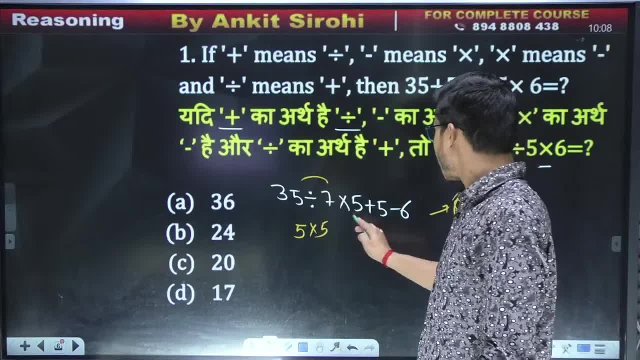 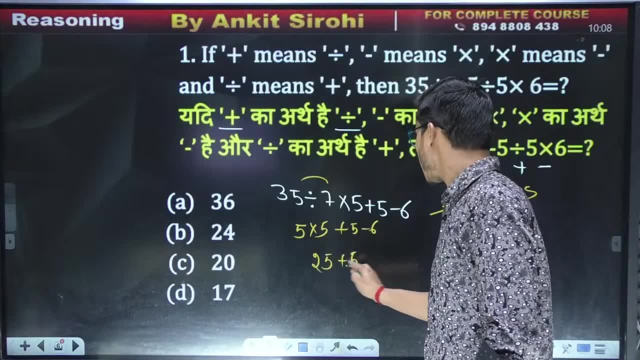 Multiply by 5.. Okay, brother, whose 5's? Now what is it? Plus 5 minus 6. See: 5 times 5 is 25.. 25.. Plus 5 minus 6 is equal to what? 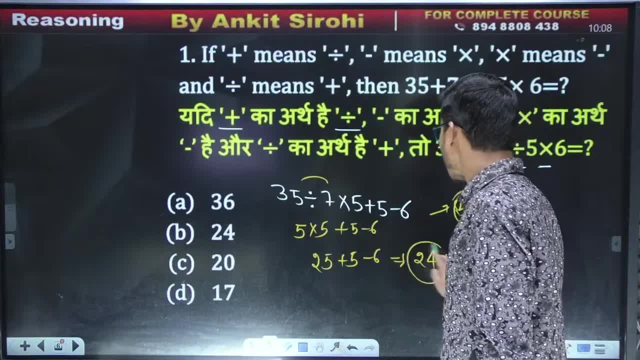 24.. Because 25 plus 5 is 30. 6 out of 30 is left. So 24 is left. Option number B is correct. Which one will be? Option number B will be correct, My dear friends, in the option. 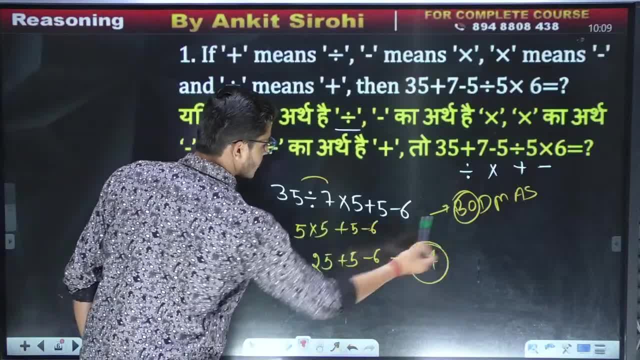 It will work. Everyone's answer was standard 24.. Everyone's answer was good at the beginning. In the meantime, number 2 is in front of you. You have to tell here: This star is here To change these signs. 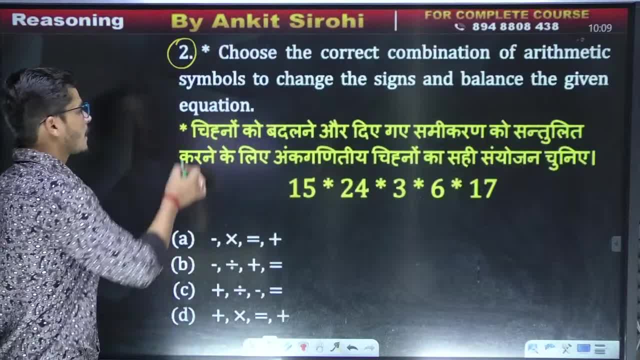 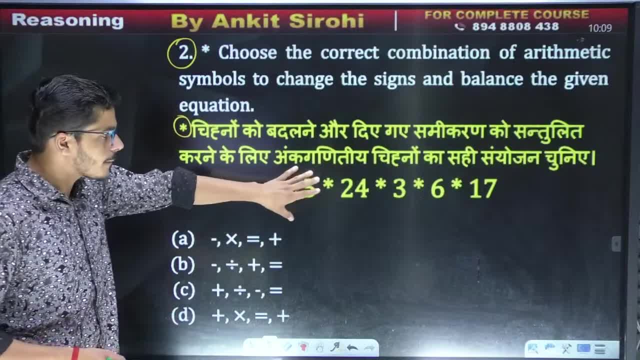 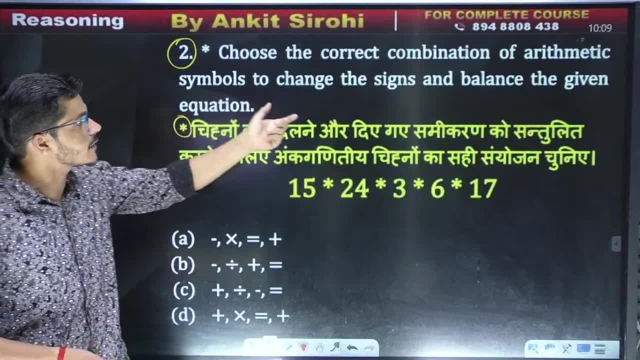 This star is here. Which sign can come here? It is given here. Choose the correct combination of arithmetic symbols to change the sign and balance. the given equation Means It has to be balanced, Have to be balanced. What does balance mean, my dear friends? 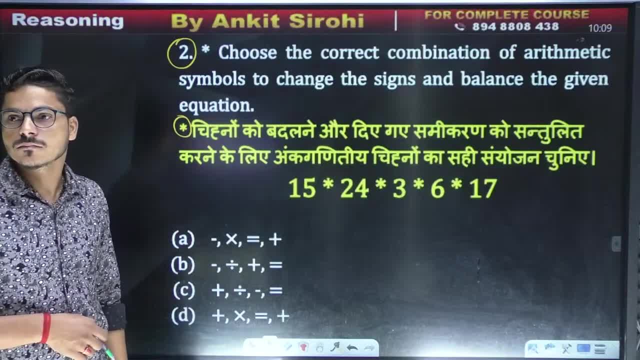 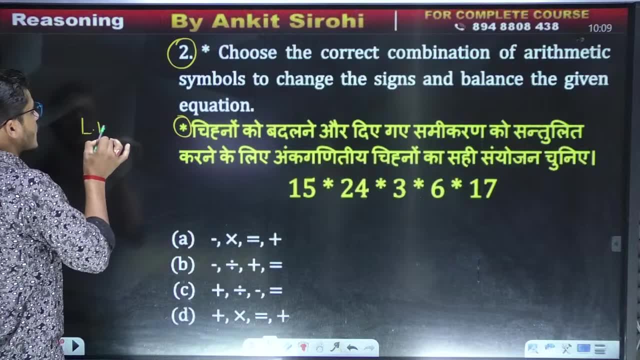 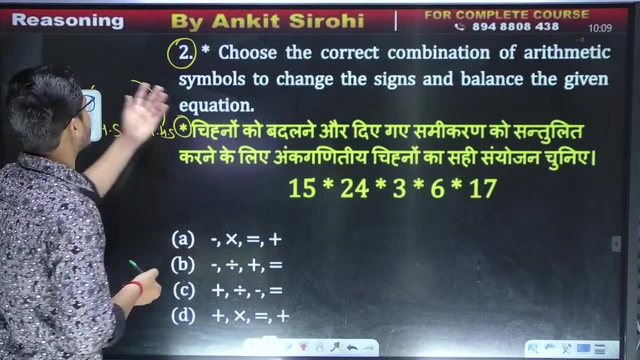 Brother. See What does balance mean, my dear friends, That LHS is equal to RHS. You have all been studying from childhood. Now you will say: Is LHS equal to RHS? The meaning of right hand side is the same as left hand side, which means LHS is equal to RHS, which means the left hand side is equal to the right hand side. 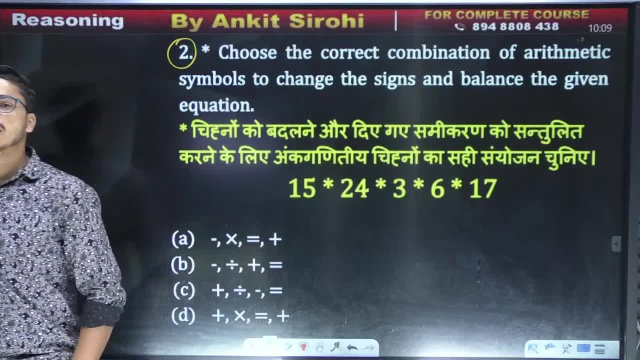 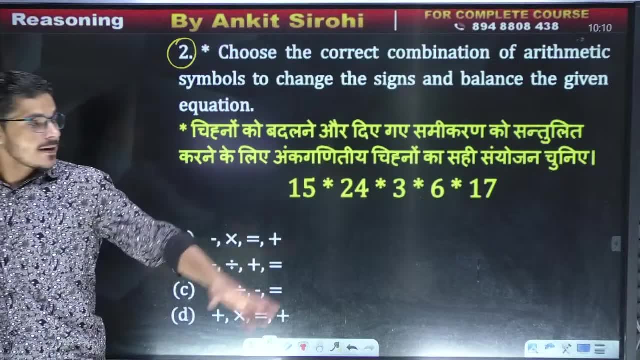 So let's see, dear friends here, you will see whose correct answer is going to come, I will see whose friend's correct answer will come. Who will answer first? Who is ready, dear friends? Brother, you have to tell in whose place which work will have to be used. 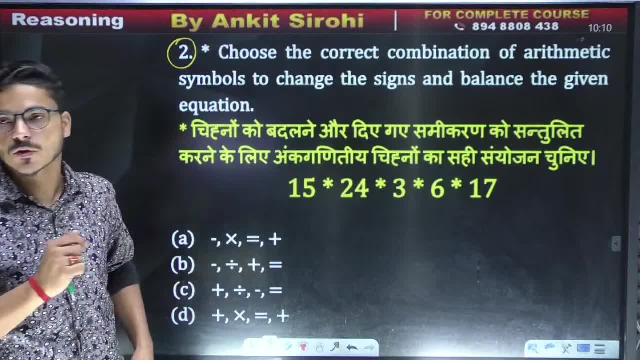 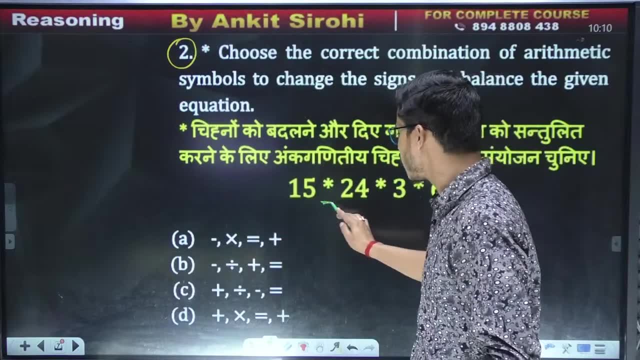 Whose work will have to be used. Let's see, Come, friends. first of all, it is a small thing, so let's start with this: Look, come here, my friends understand. first do minus here. You all can see it yourself. if you have set your mind a little bit here, then it is multiplied. 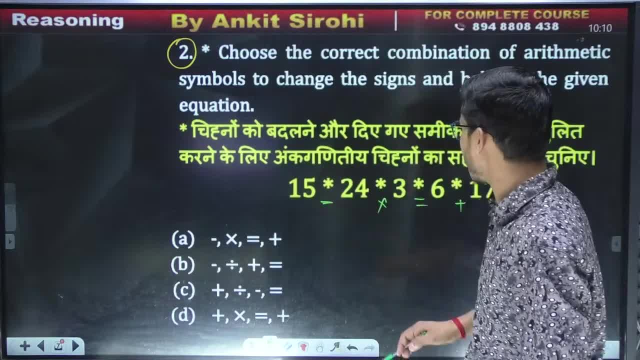 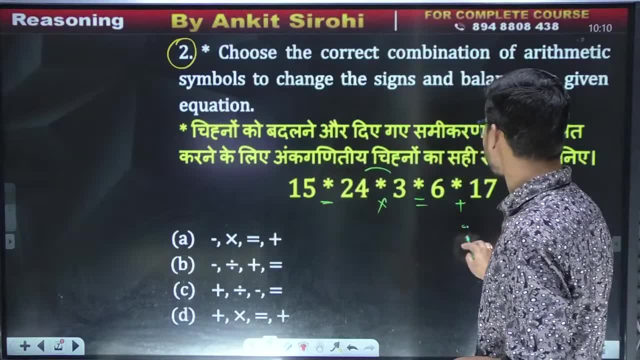 Okay, then it is 12 times and then it is plus. See if my friends go from 24 to 72,, 15 out of 72, then do it here in the mind calculator. This is equal. equal means 23 is coming here, then 23 will come here. 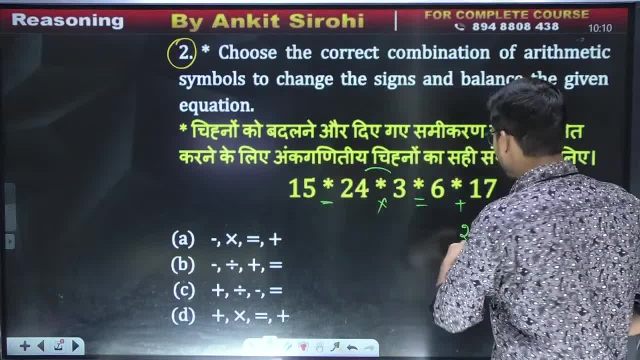 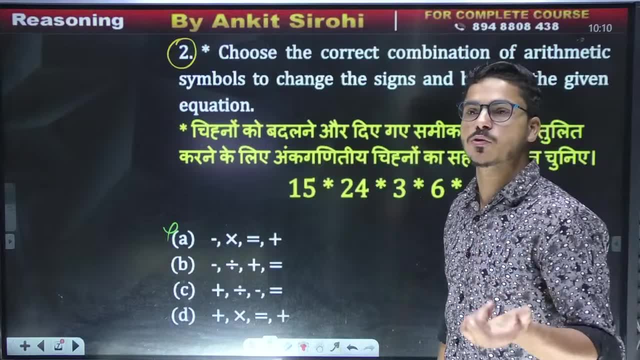 24 to 72,. 15 out of 72 will go, 23 will not come, Did you say? no? It is better to solve the whole thing, dear friends, by talking like this: If the first is wrong, then we try to look at the second. after the first, look at the third or the fourth. 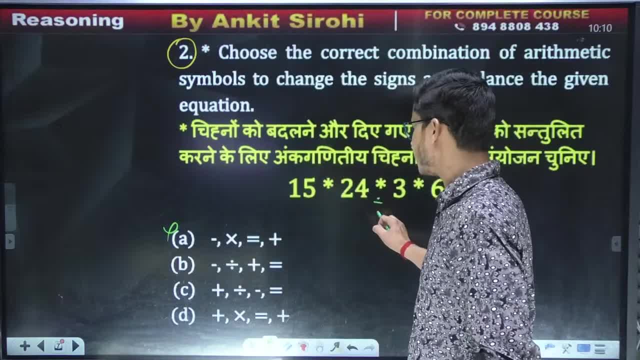 Come on, look at the second quickly: Minus and part. here is the part, Isn't it With you? here is plus, here is equal, And what is here Minus. So, first of all, if you do the part, then first of all it is 8.. 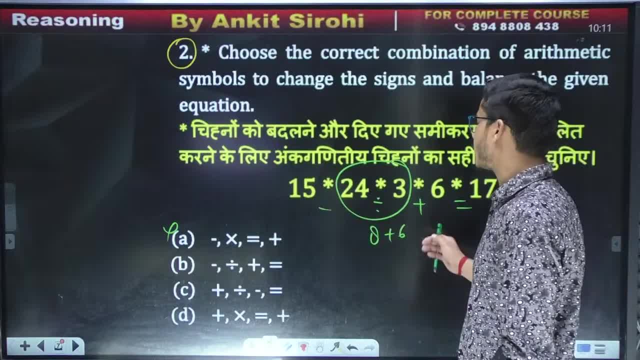 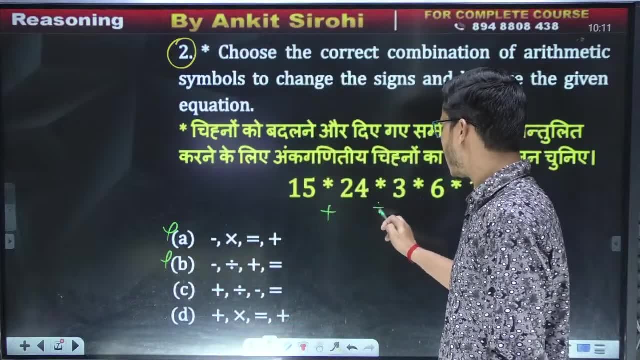 And plus 6,, 14, out of 14,. first of all, if 15 will go, then you will say that it will not come at all. My brother will not come at all. Third, he said plus, part, minus and equal. 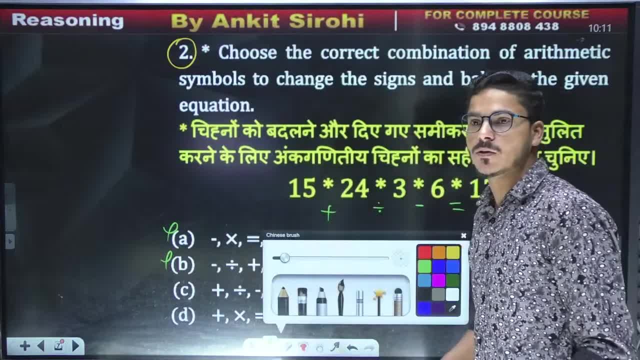 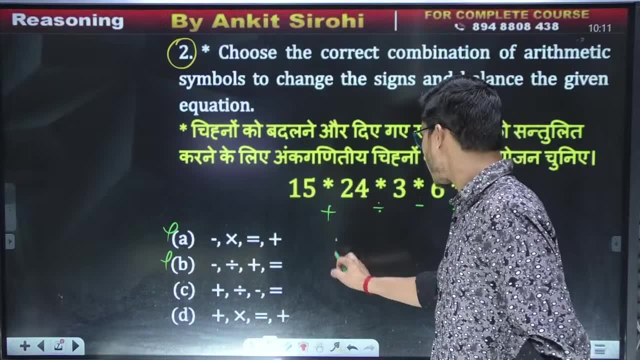 Come on, let's see it once. Let's use this first, Dear friends. okay, C is the answer. C is also the answer in between us. So what will happen of this, my dear friends, You will see. if you solve it here, then it will be 15 plus 24, part 3, minus 6, equal to 17.. 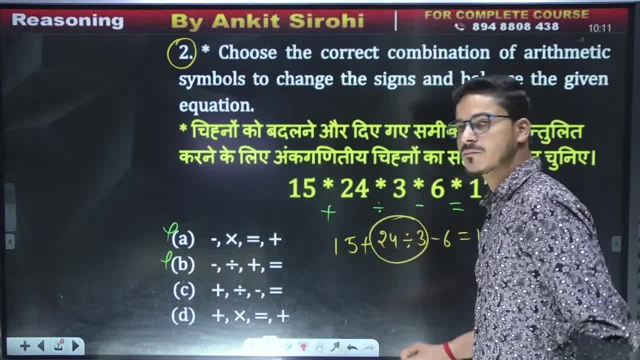 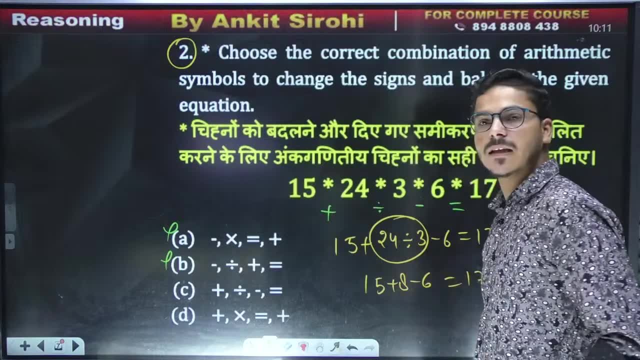 Will it happen or not? See First of all, we will do the part. How many times did it go? Eight times, Dear friends. 15 plus 8 and minus 6.. Equal to 17. See: 15 plus 8, 23,. out of 23,, 6 will go. 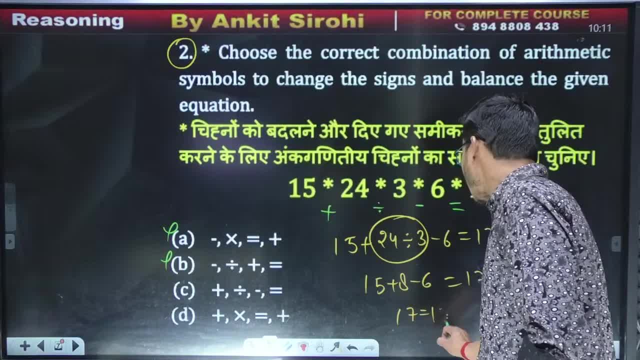 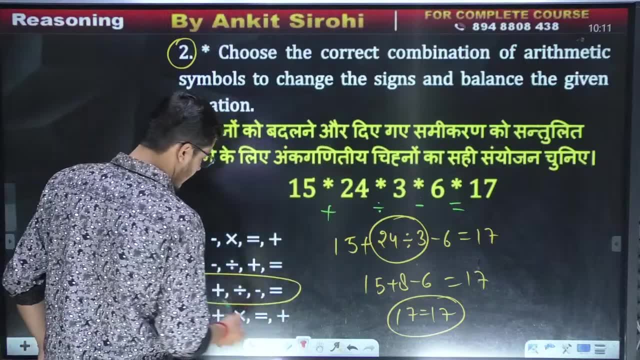 So we will say: yes, it is 17,. that is 17.. So who made 17 equal to 17?? Who made our equation equal? He said the signs given in option number C, the signs given using them. we made the equation equal through option C. 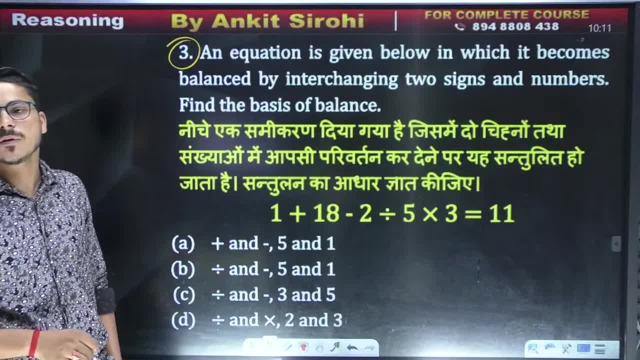 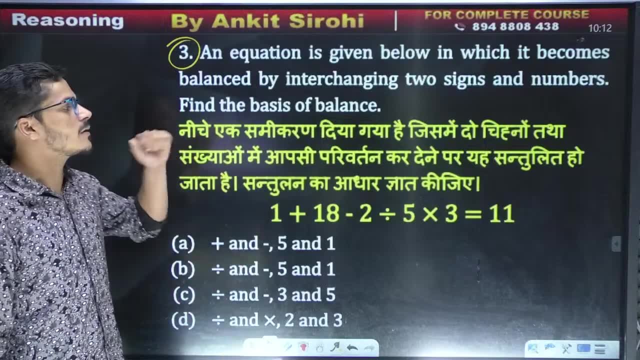 All the friends had a very good answer. In the meantime, the next question has come in front of all of you, dear brothers. What will be the next question? Tell me, Baba. It has been said here, my friends, that there is a equation below in which two signs and numbers change each other and it becomes equal. 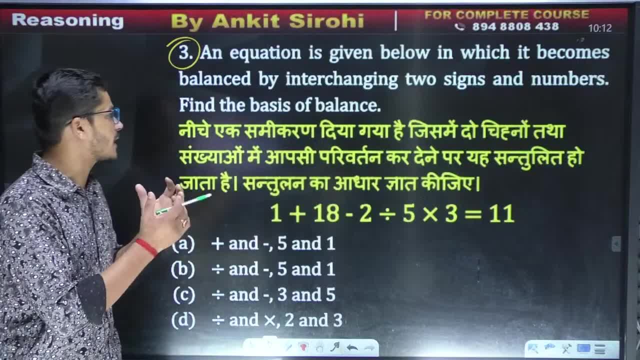 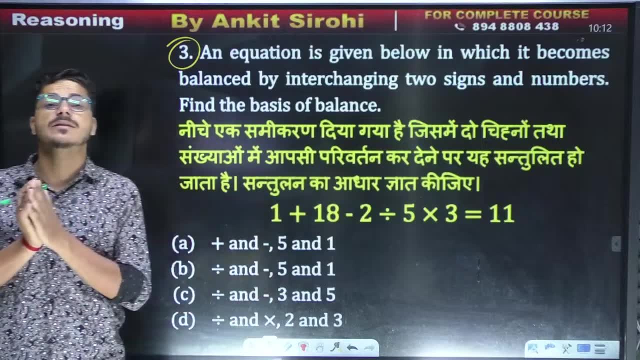 Find the basis of balance. What does it mean to say, Dear friends? We have to tell you the basis of balance Here, which will be the balance from which we will have to choose which option where we have to change in the sign, and if you are a friend, then we have to change in the numbers. 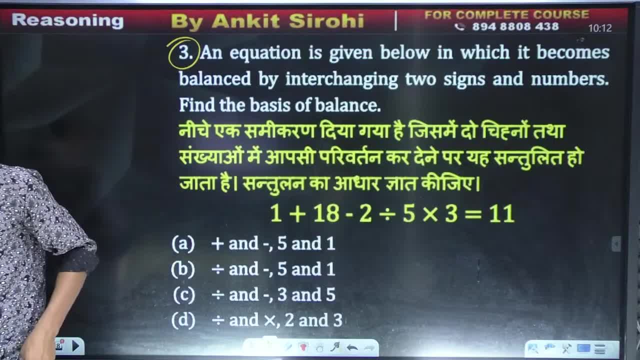 Very good, my dear friends, Very wonderful, Very wonderful. Dear friends, if the class feels that it is going to be a useful class, then please share the class And, dear friends, if you like to like, then it will work. 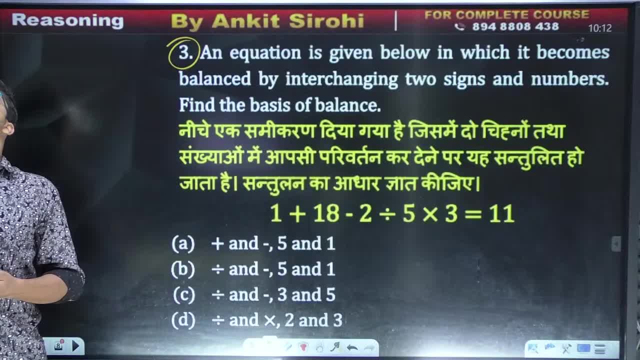 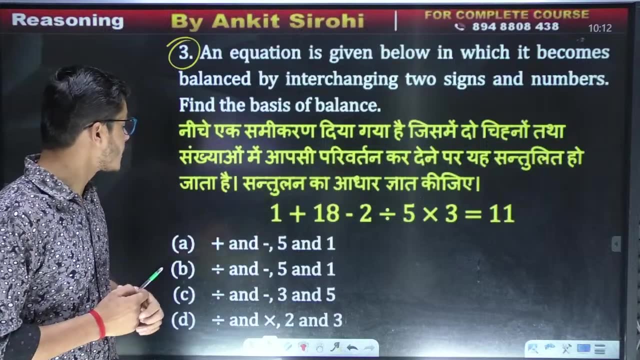 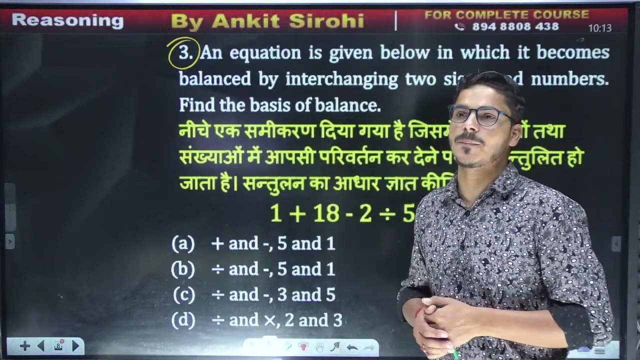 Because the number of likes is very low. Dear friends, it will work. No, dear friends, leave it that way. Okay, Let me tell you, my friends, what is the answer to this. See What it means to say. Pick up two signs like this, which will change, and, along with that here, numbers of the. 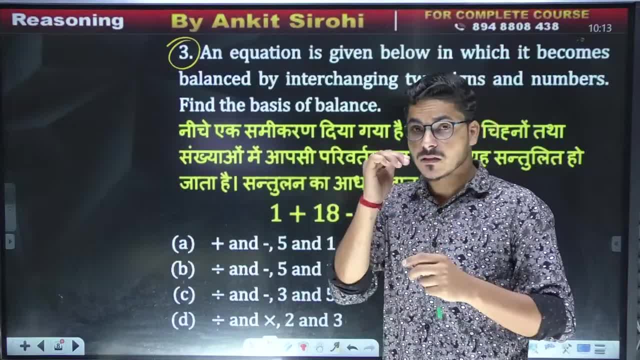 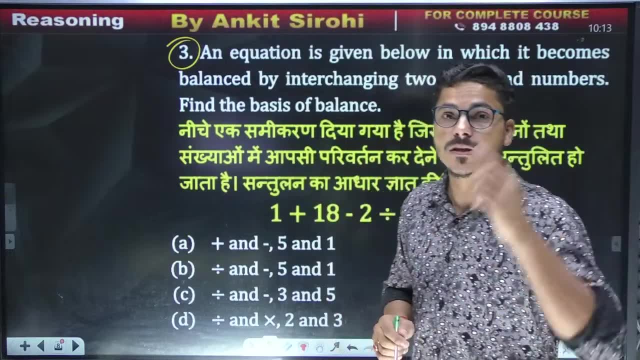 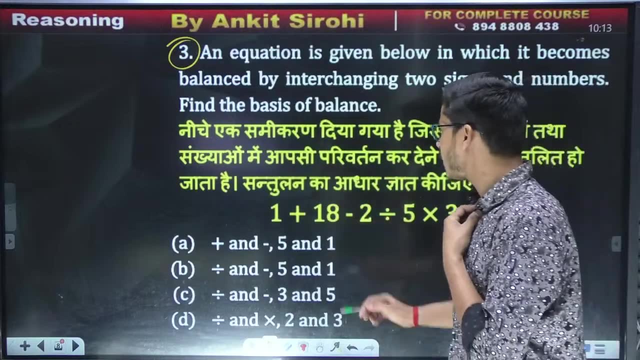 numbers, Look, Look. It means that you all learn to do the calculation so fast in this. You used to say that I am getting into this, So it means that prepare yourself well in this. For whom: For calculation: See Change in plus and minus. 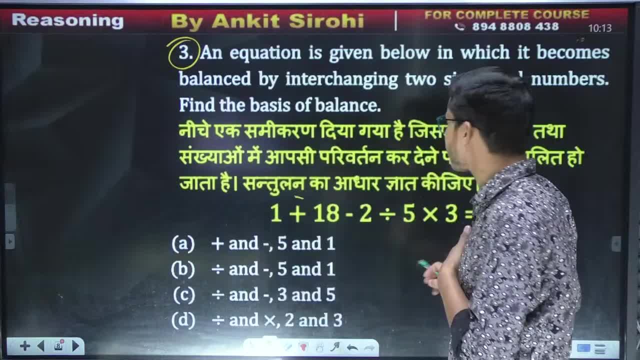 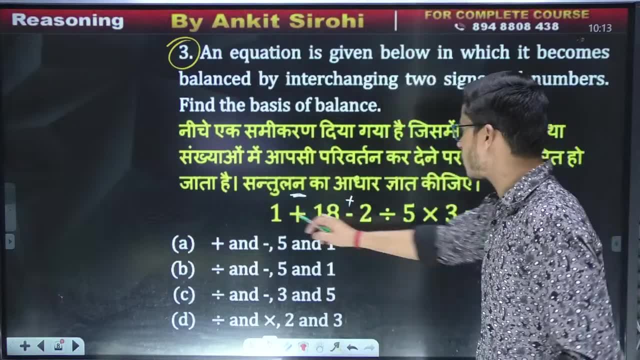 It means that minus will come here. Change in plus and minus means that in the place of plus friend, we will get minus, And brother plus will come in the place of minus. If you change 5 and 1, then in the place of 1, it will be 5.. 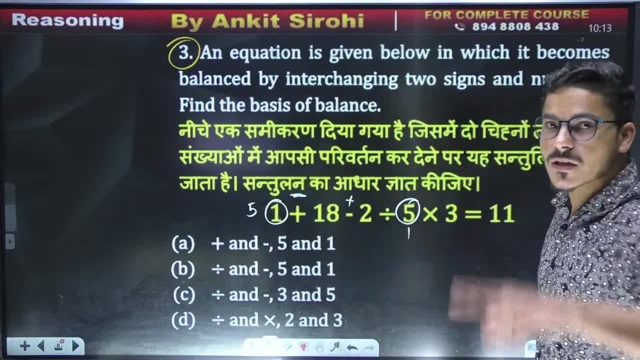 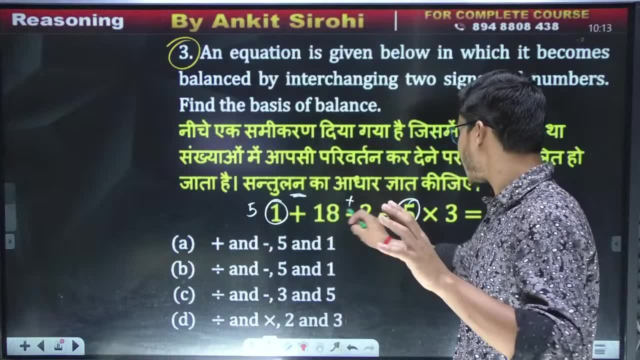 And in the place of 5, it will be 1.. Now you all have to think about one thing here. What did I say? See, There are two parts here. Now, if you think to solve it, See here: 18 plus 2.. 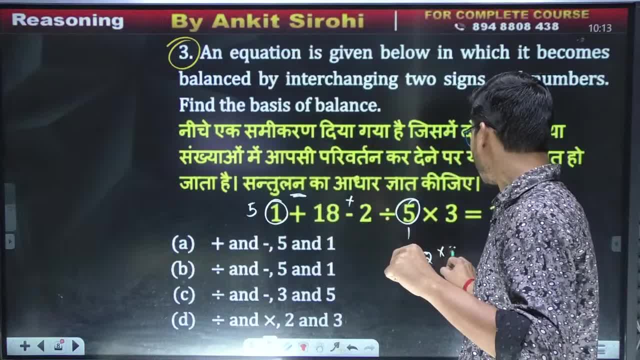 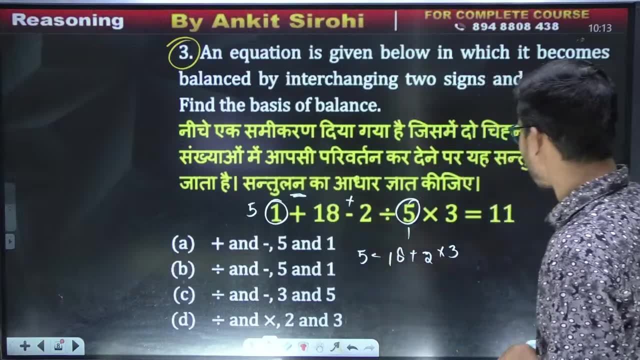 Two parts: 1.. So it means that 2 is 2.. 2 times 3. And brother, 18 plus Right And 5.. Sorry, 5 minus. This will happen. Will 11 be equal? 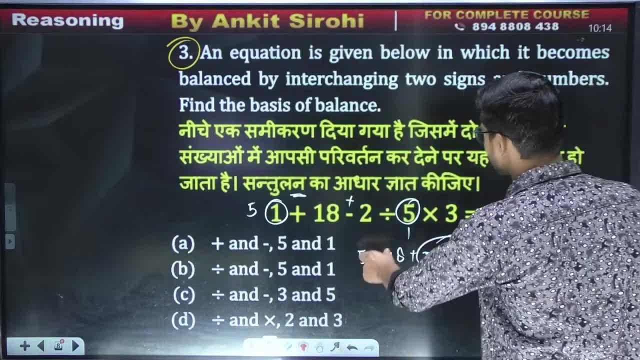 See 18 and 2, 20.. 18 and 6.. 24 out of 15.. 5 is not left. It is not left at all. Finish it, Brother. finish it, It will not be left. 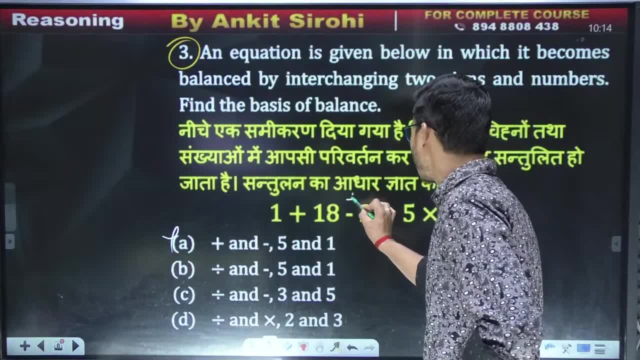 Come to the second. The second will see Part and minus have to be changed. Keep the part in the place of minus And keep the minus on the part And change 5 and 1.. Keep 1 in the place of this 5 and keep 5 in the place of this 1.. 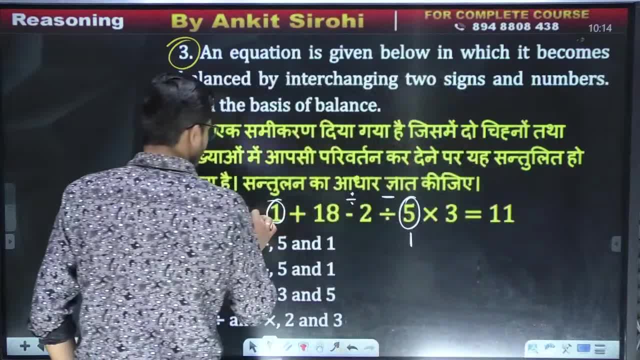 So will there be any change in the equation by cutting this 5?? Will this be balanced? So you will see, Let's write here: 5 plus 18.. Part 2. Minus 5. Minus 1. Times 2.. 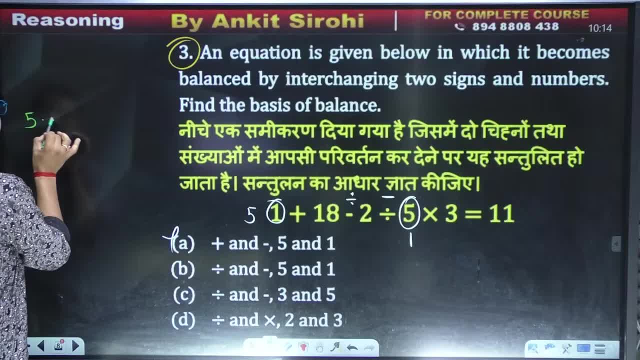 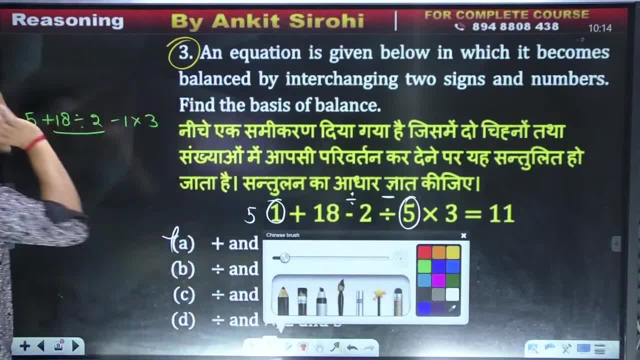 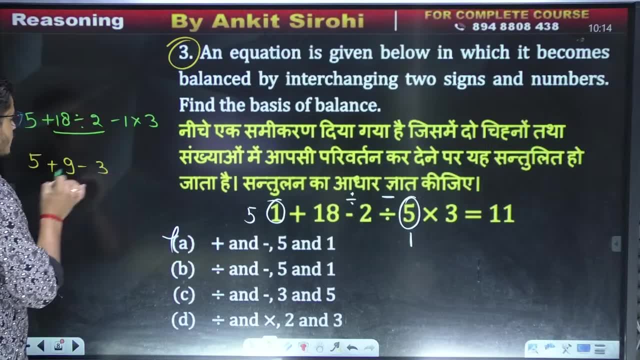 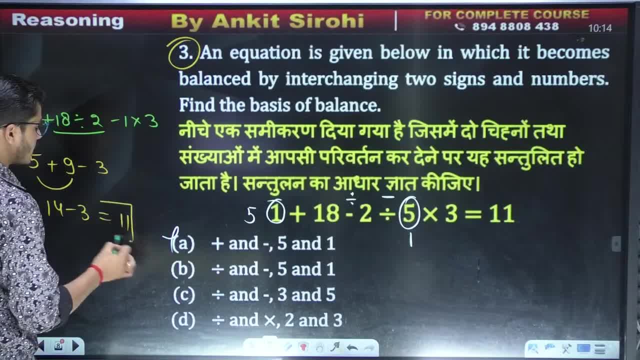 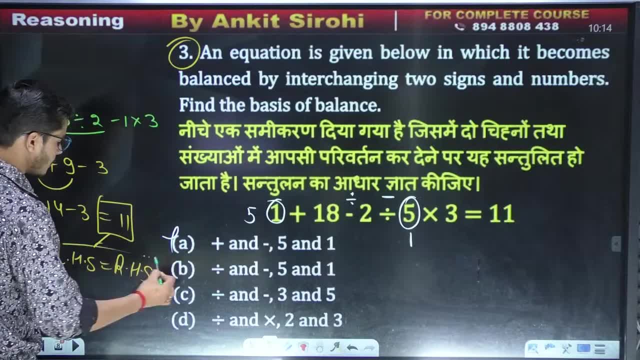 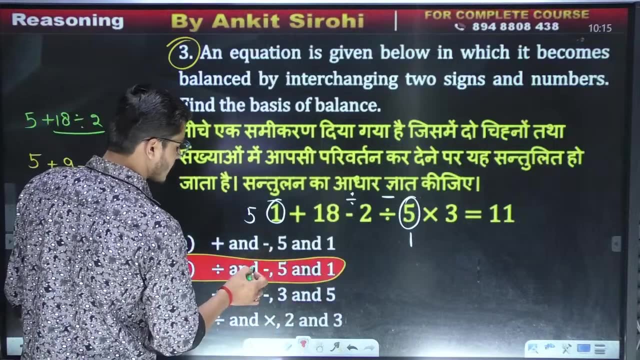 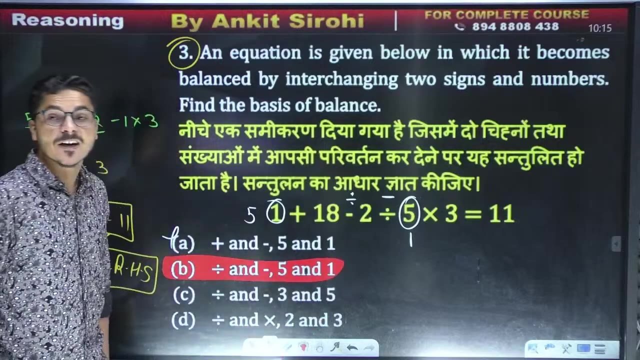 1. 1. 1.. Can I get 11?? Can Iリ get 11?? will we solve First? we will solve it, Brother. solve this. Take a look, brother dot plus, With the help of option number B, the sign that we have changed here, here, friends, we have changed the number For that. dear friends, thank you for option B. Option B will also be the correct answer. 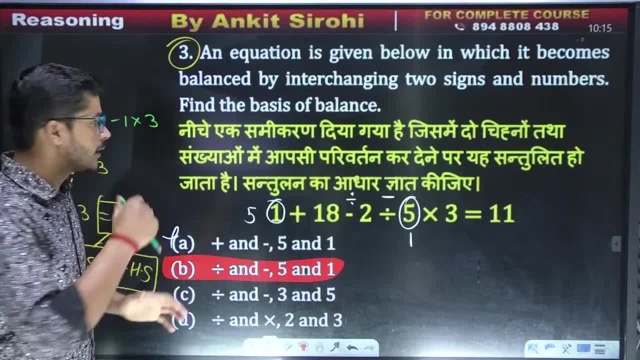 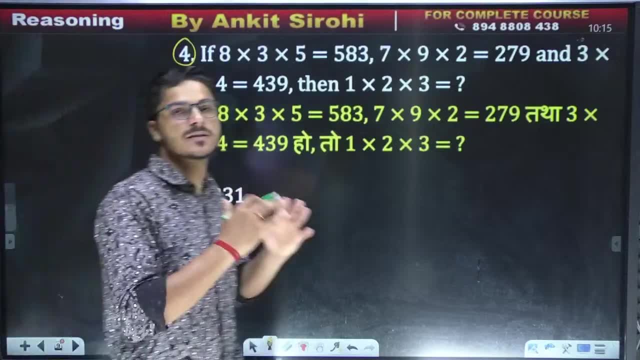 The third one is also a wonderful friend. Good morning. In the meantime, my dear friends, there is another wonderful question, number 4, in front of you. Which is the question number 4?? Let's see, which is the question number 4,. dear friends, I will answer here by focusing, Because here you will see a wonderful thing in front of you. 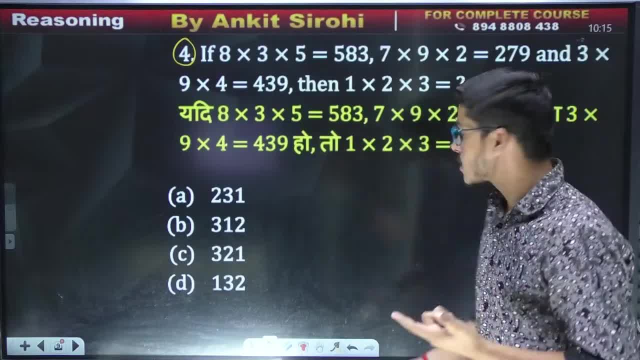 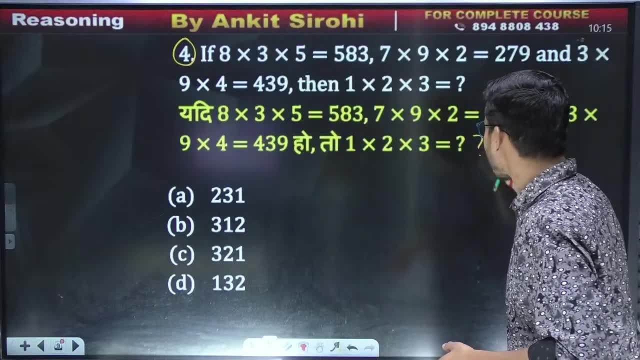 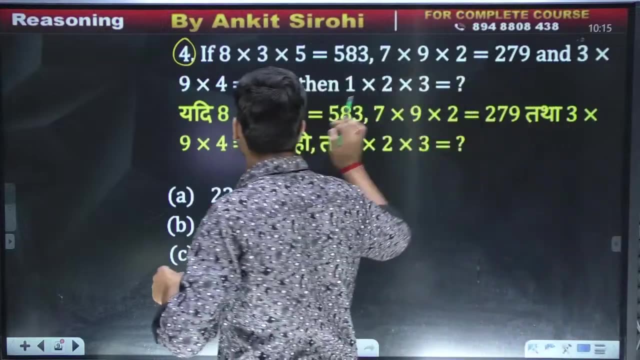 If you all think that every question I have done so far, all of you have different types. many types have been given to you to see, This is also of some different type. So tell me, my dear friends, what will come here. What will come here For this? dear friends, whatever is wrong, whatever logic, whatever is done here, it will be done here. 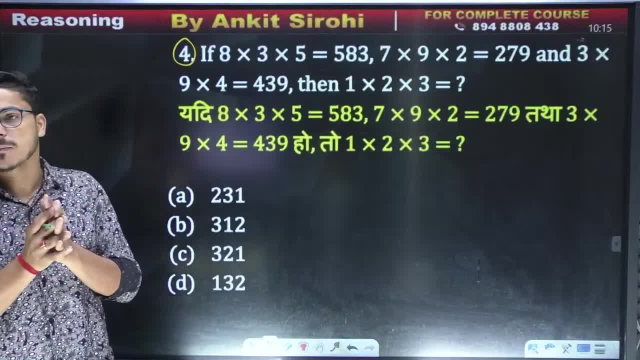 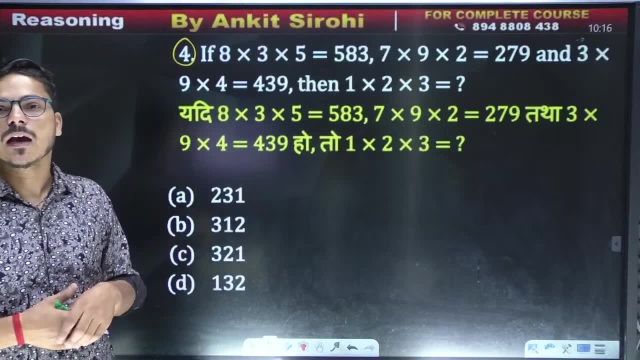 See 312.. Very good, Brother is coming. Brother is very good. Kambya ji has 312.. Dear friends, Archana Pal ji is saying that I did not understand. Archana ji will understand. There will be many such questions. 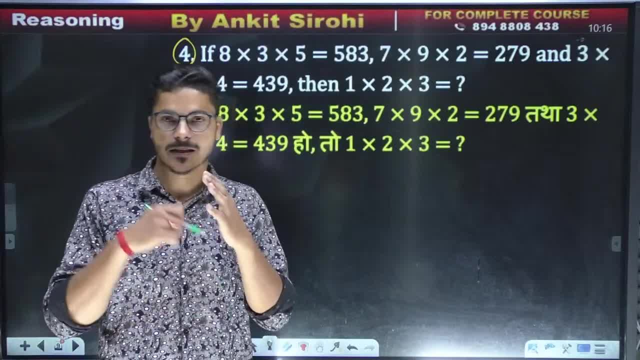 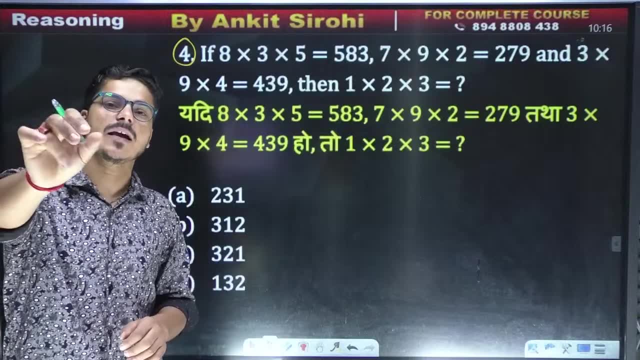 See here. If you understand from the first question, then you will leave the class and go. This was just a joke. See, Dear friends, do not worry, You will understand. Have faith in this Here, it is Okay See. 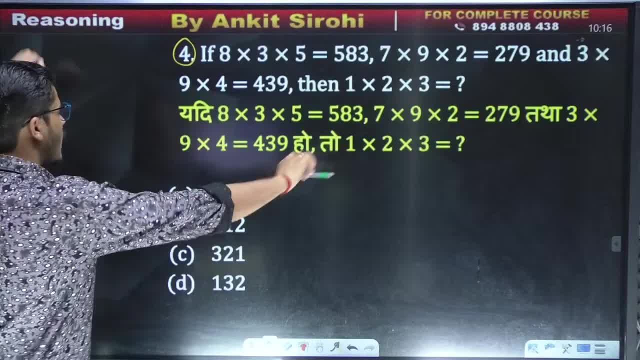 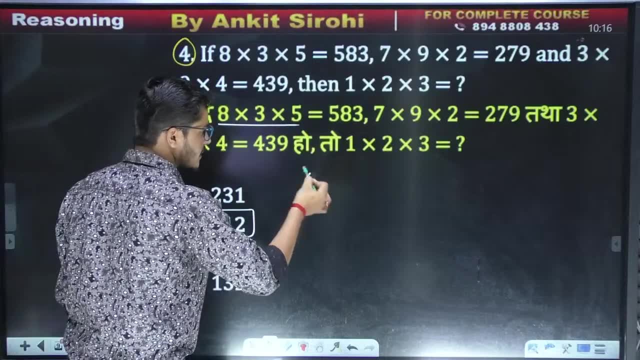 Here 312 answers have come, And I say that as far as I think 312 are correct answers. See Why Here 312 answers have come. See Why Here it is written: dear friends, understand 8 times 3 times 5,, dear friends. 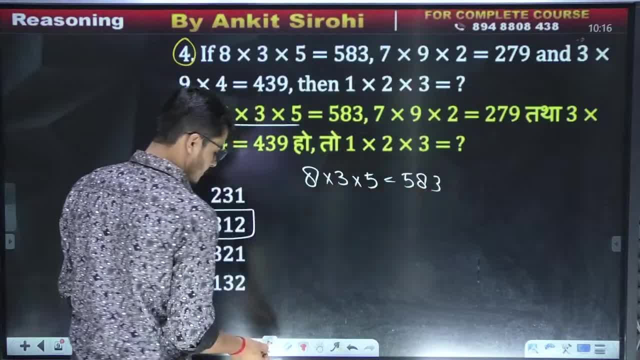 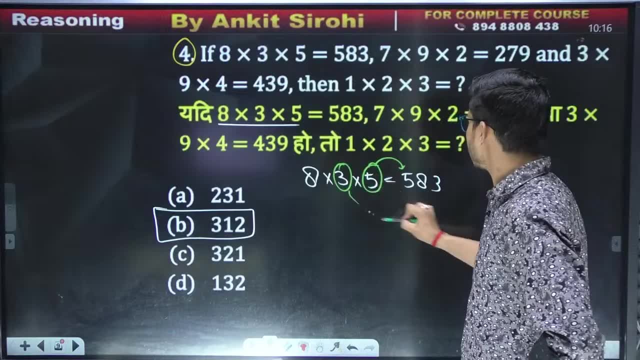 Equal to what 5, 8,, 3.. Did all of you see? Yes, What did we see? You saw that 5, here it is, wrote. the last one here Wrote the middle one at last. 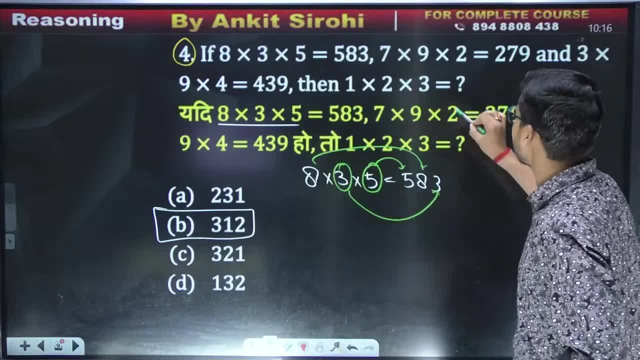 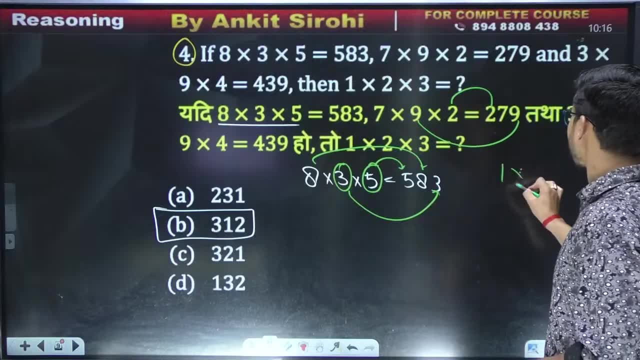 And this one is written here. What is this? You said that, See, And the last one of 9, the second one, And this is the second one, exactly. So how is 1 multiplied 2 multiplied 3 going to happen in the same way? 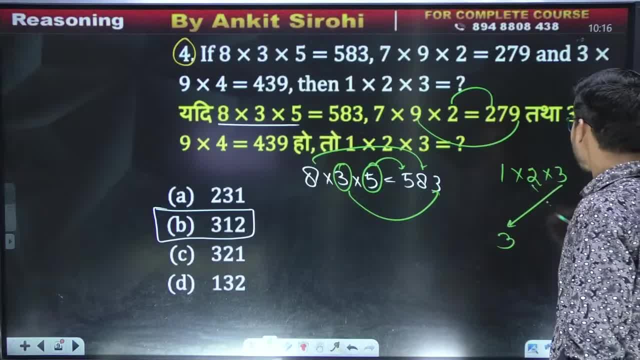 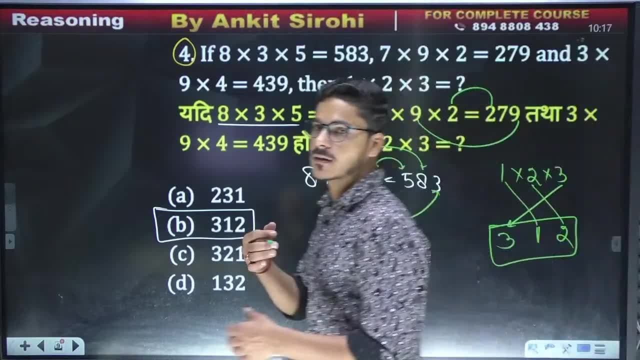 So you said: First write this as 3, write the middle one at the end and the second one in the middle. So 312 is done. What has been done here is that 312312 has been changed. Dear friends, it is very good. 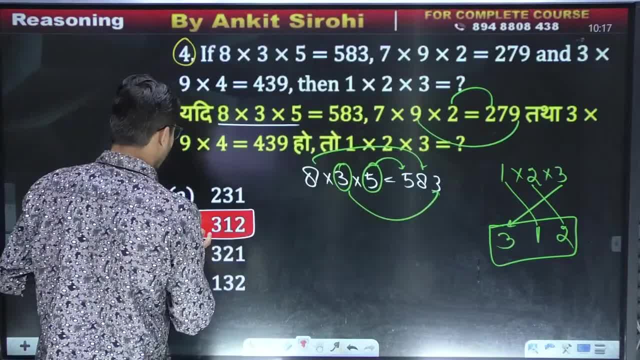 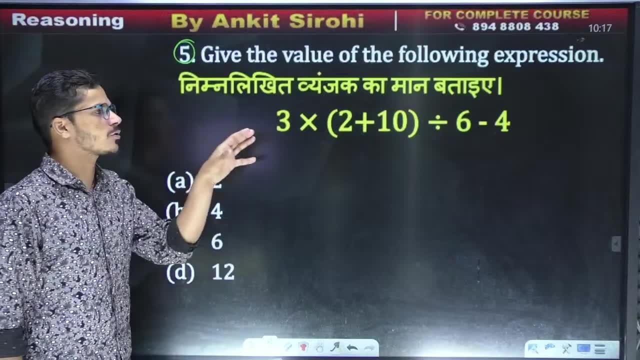 Which is 312?? It is 4.. It is the correct answer, dear friends, and it is your honor. Okay, let's move on to the next question, Question number 5.. Now you have to tell everyone that, after solving this, dear friends, you have to tell everyone the value of this venjak. 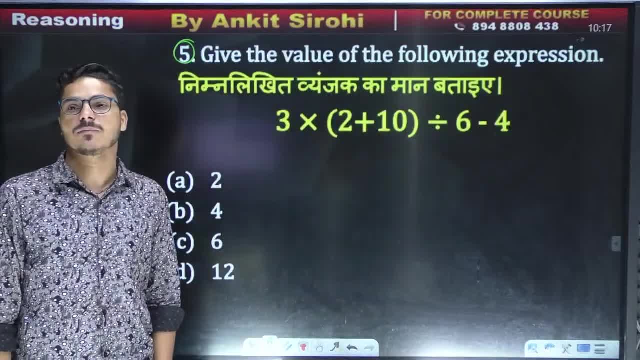 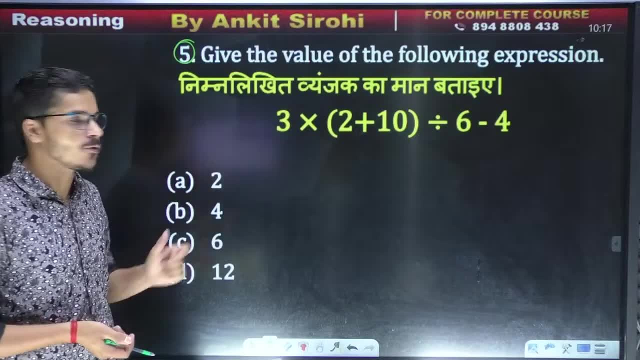 So I want to see what is the value of this venjak. Dear friends, 312 is the correct answer. In the meantime, one more question has come in front of all of you, And you are all ready, Dear friends, you are all ready to make a peacock out of it. 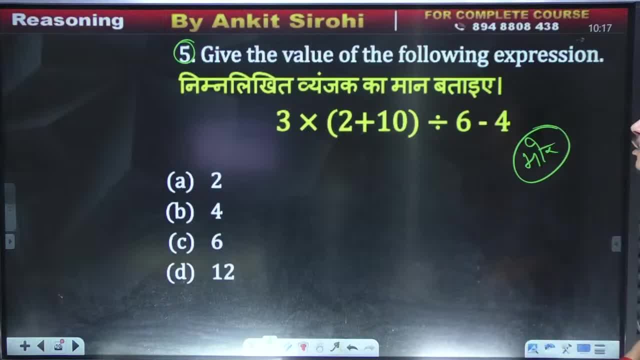 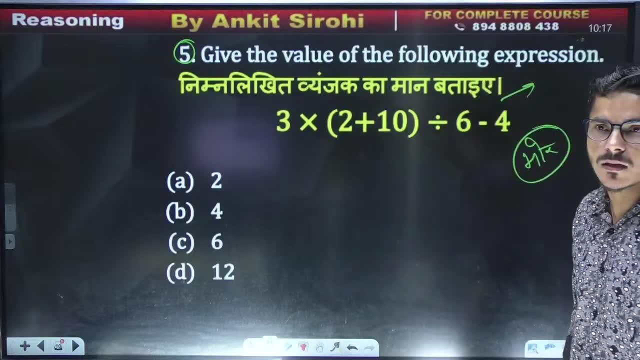 And brother, you will make a peacock and leave it. I know Because the mathematical operation is going on without a doctor, without a cane. Dear friends, we are doing the operation of questions. We are doing the operation of questions Why? 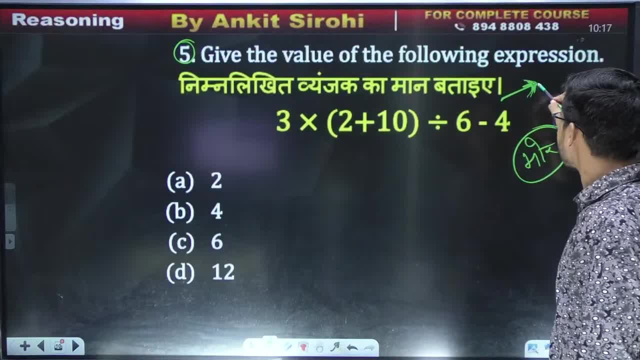 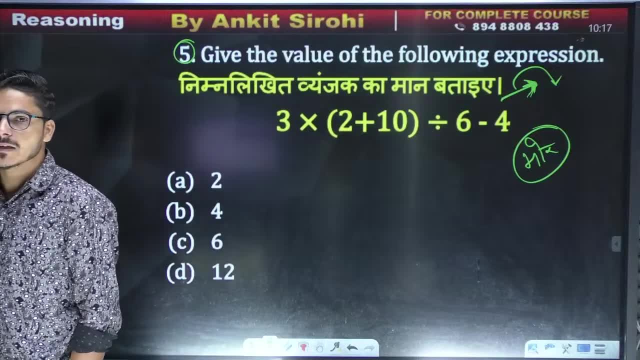 Because the person who makes the peacock, the person who makes the doctor, the power we have tomorrow, The power we have tomorrow 5a, Dear brothers, 5a, Oh brother. 5a is very good, Dear friends, very good babu people. 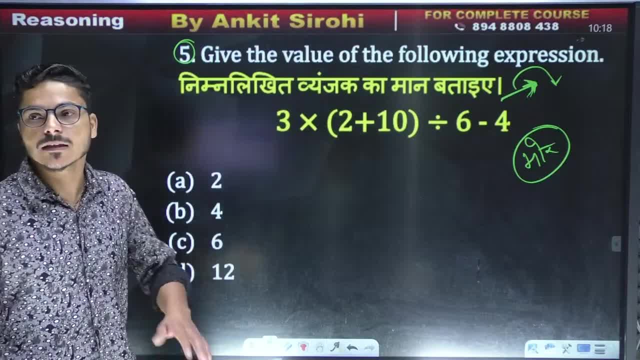 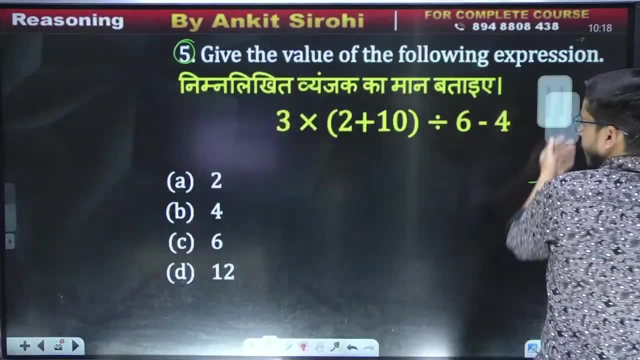 Dear brothers, everyone is getting 5a, 5a. Okay, let's see Whether it will be 5a or not. dear friends, all the things come quickly. Look if I talk, dear friends, that first of all, we knew that by using the rule of the board mass, we have to solve the bracket. 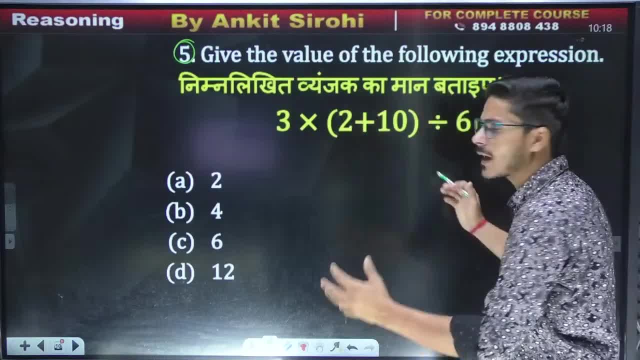 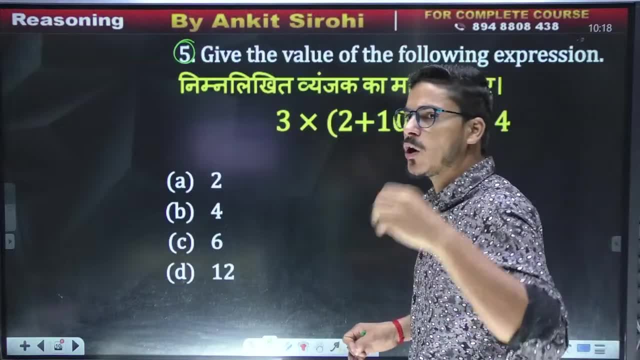 We have to solve the bracket. Even if there is any mess all around, there is a wall. these two are in it. dear friends, first there will be a fight, we will solve the problem and bring it out. Okay, He said there are two of them. I will tell everyone that you all are looking right now. it will be right. 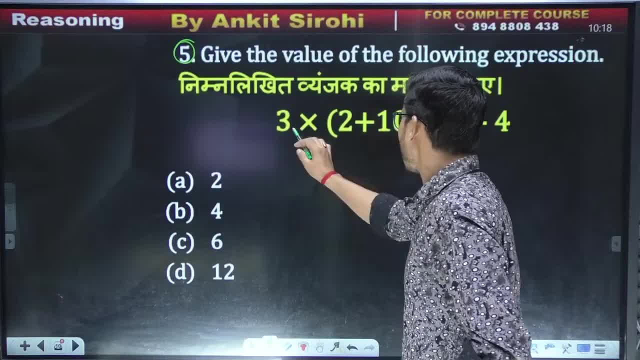 So you will see, there are 10 and 2 bars. So, dear friends, what will be 3?? Dear friends, what will be 3?? Multiply Now, it came out 10 and 2, it is 12.. Done. 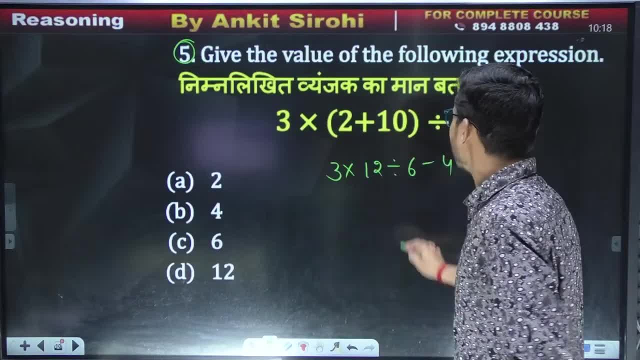 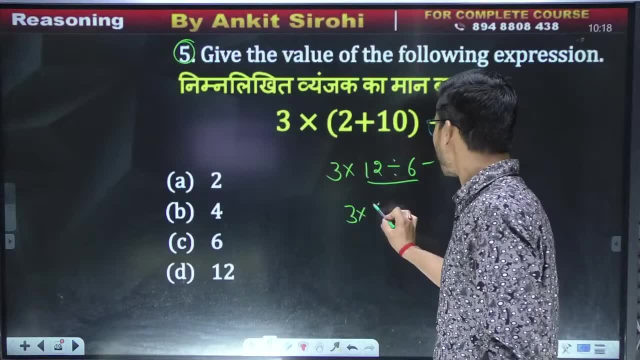 Dear friends, divided by 6 minus 4.. So first of all, then the rule of the board mass will be taken. now the D mass will be taken. it will be divided. If I say 3, multiply 6 times 12 minus 4,, 3 times 6, 6 minus 4, my first brother will be 2.. 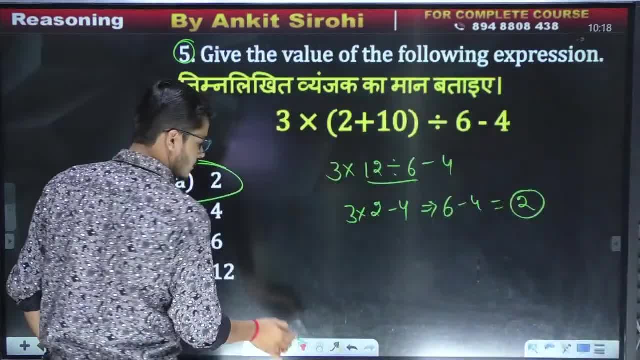 So our correct answer will be option number A 2.. Which one Option number A 2 will be? Don't worry, all of you have an excellent answer, dear friends. In the meantime, we will solve it in front of all of you. 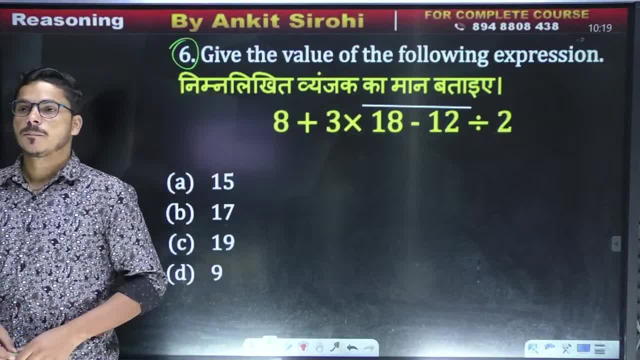 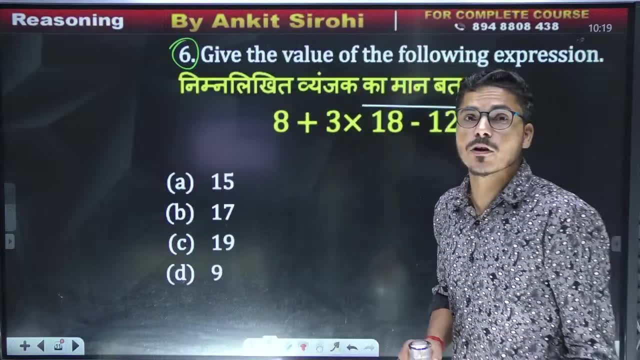 Question number 6 has come, Question number 6.. First, break the wall. Yes, absolutely. These are the fire ones who put the glue ball, or these are the pubg ones. I have seen many of them, So they put it. 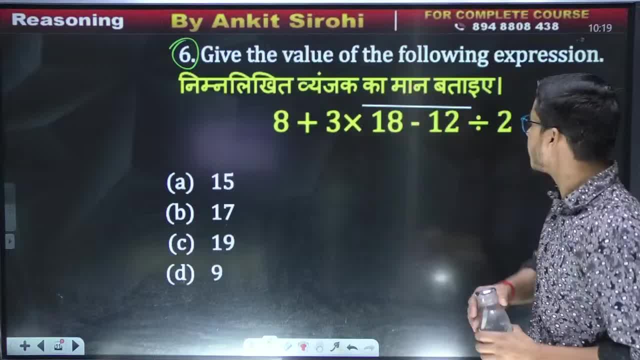 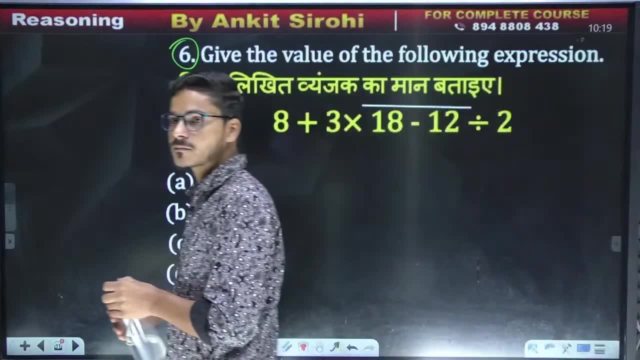 First break it Before breaking it. just like that brother, you have to break it Now. look here, Baba, Look here. a wonderful question is in front of all of you. Now let me see whose correct answer will come. dear friends, 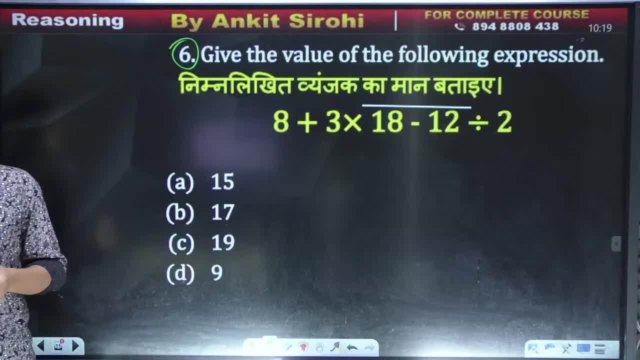 Come on. Yes, absolutely, Very good, Wonderful, Yes, it was absolutely good. the last two Tell me about this, dear friends, what will happen to this? Good morning, sir, Brother, good morning, Good morning to all, dear friends. 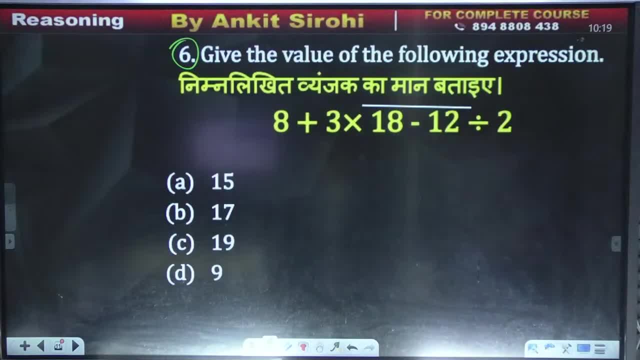 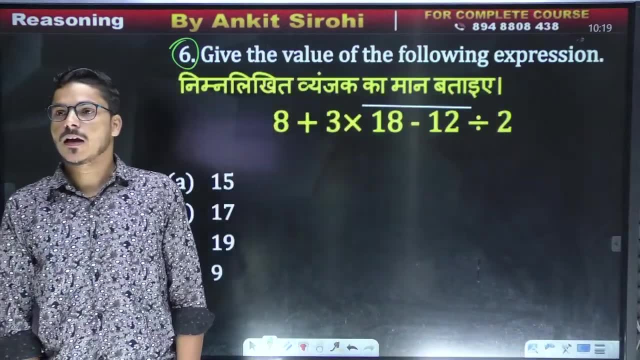 Good morning, dear dear good morning to all friends. May your day be a happy one. May your day be a blessed one. Dear friends, come on, Yes, brother of someone else, Of someone else. dear friends, If the answer is this, then tell me. dear friends, 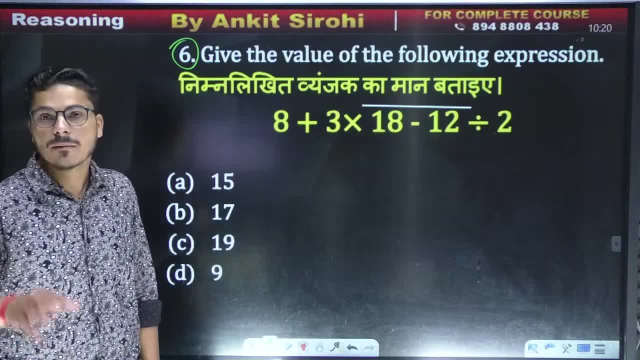 Six questions in front of you, Six, Come on, Baba. none of them came. It didn't come right. Come on, we will tell you. The option is wrong. We were seeing dear friends. it may be that the option is wrong. 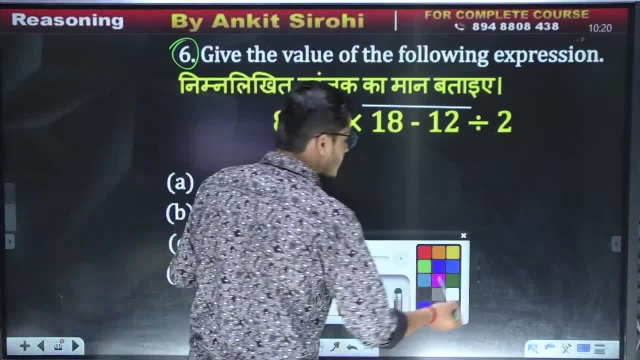 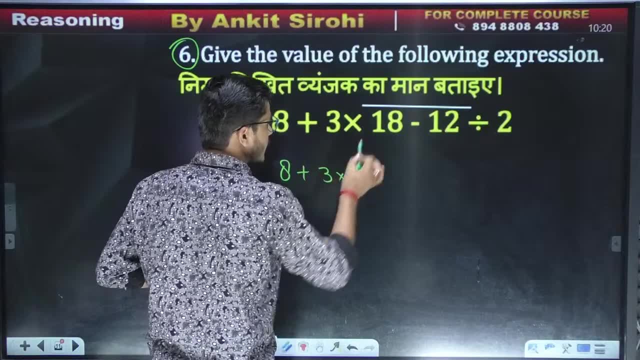 It may be. I don't say this. Come on, First of all, you know that we will solve this. So, dear friends, solve this. So say here eight plus three times Eighteen. out of six, say six. 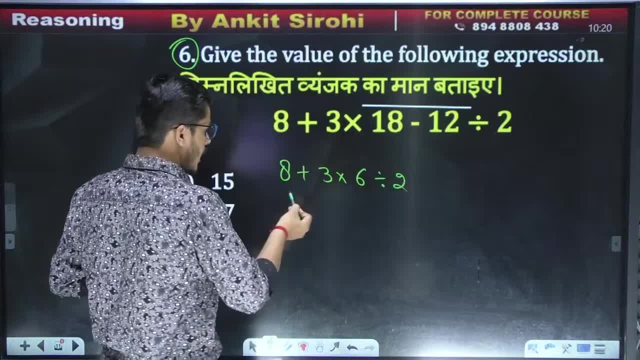 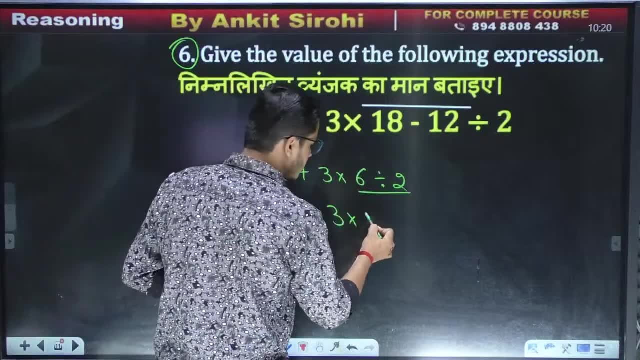 Part, my dear friends. two, Is this done? Yes, Now what to do? Eight plus three times, Dear friends, to use the board mass, first of all you have to give the part Two, three, six, See. 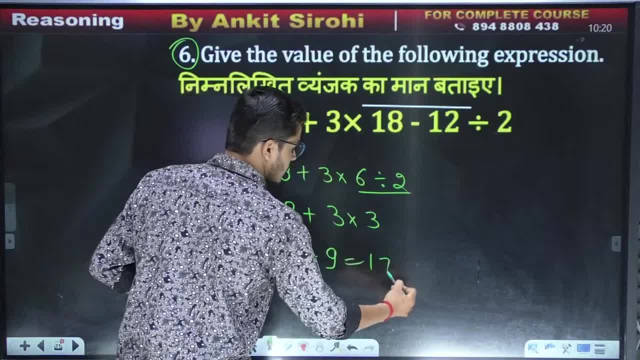 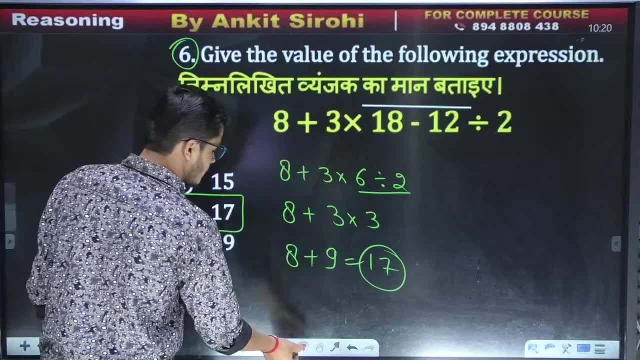 Eight plus three, three, nine. Equally, my dear friends, it will be seventeen. Is it seventeen anywhere? Because, first of all, you had read That, dear friends, it is half of ours. If our dear friend knows it in the form of a bar, 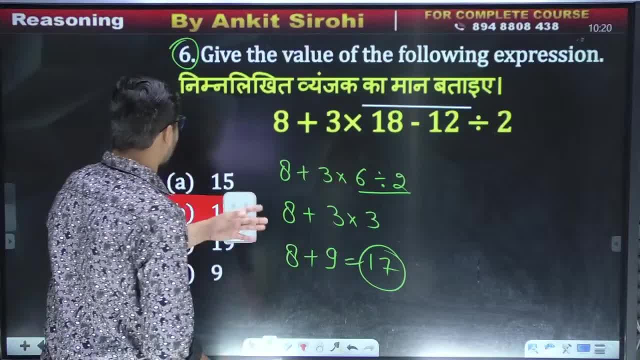 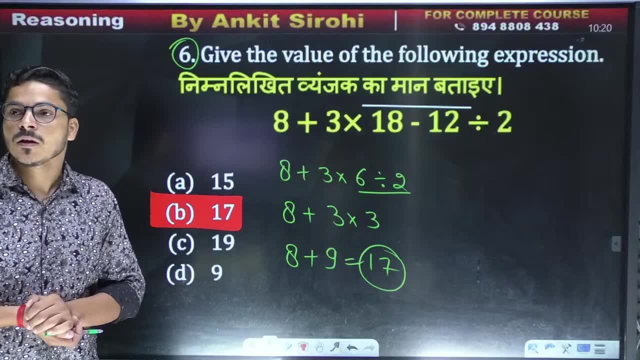 Bar brother, which bar The same bar. This is the bar with the question. So it will be seventeen, Dear friends. there are seventeen options. Option number B: Yes, Absolutely, dear friends. Absolutely, Once dear friends done. 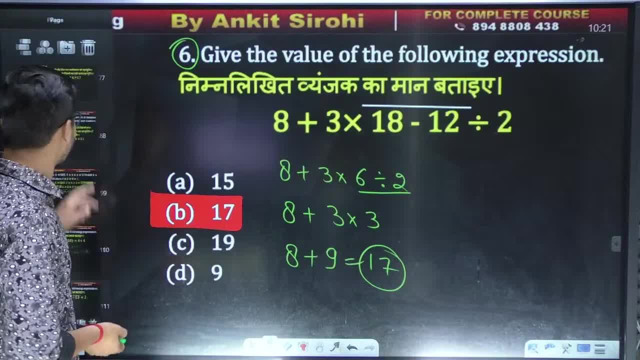 How will 56 come? First of all, brother come, See, brother, come here. How is 56 coming? My dear brothers, eighty-eight, fifty-four, Babu people, See, come here. Here we saw that the line will be 16 first. 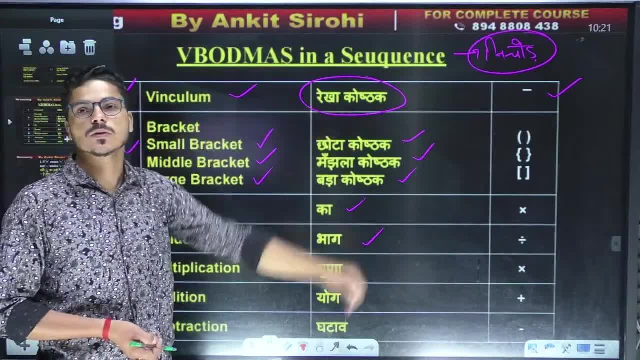 What will happen? The line will be 16.. What will happen? What will happen? What will happen? The line will be 16, first, And what will happen? And what do we do? So, dear friends, we have done the same thing. 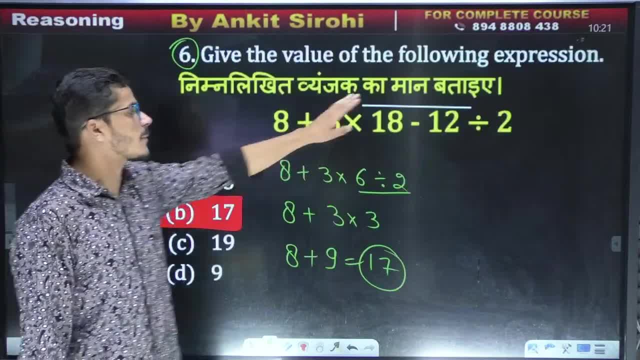 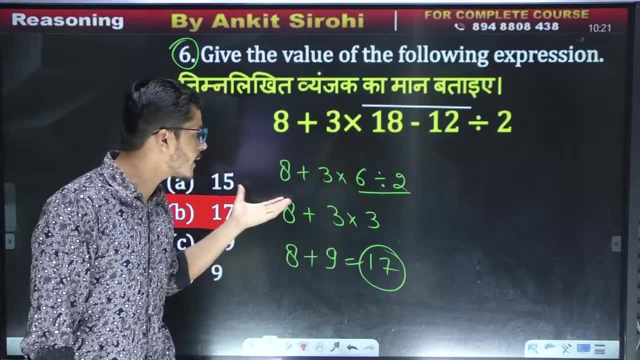 We have also solved the line box. first, Then we went to solve it from eighteen to twelve, then it is six, Then it was written by the same way six times. now it has become our new way. we have solved one. 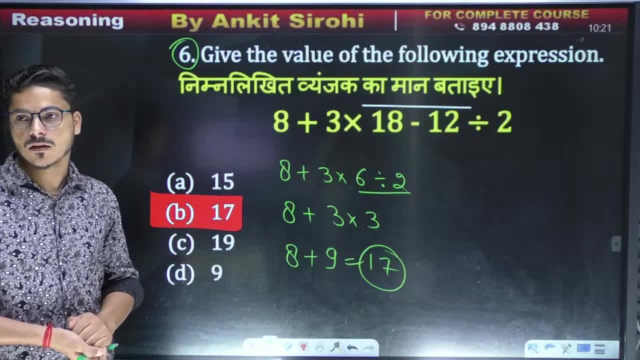 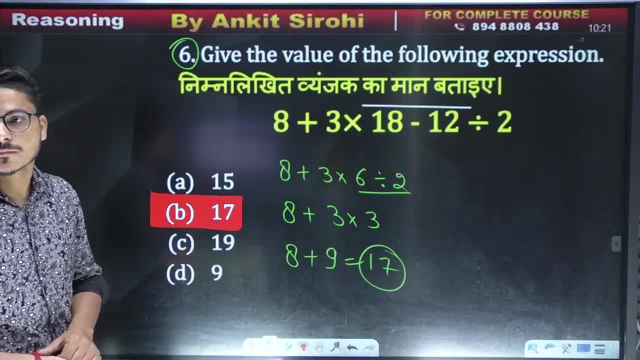 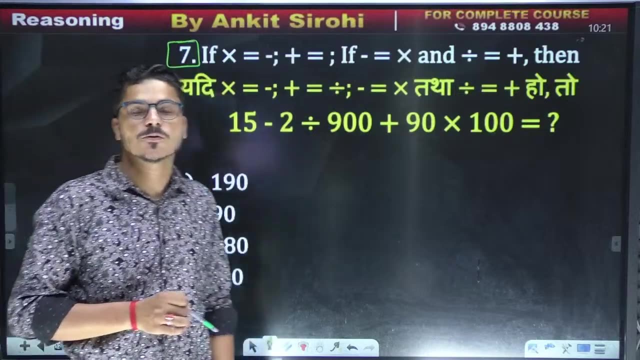 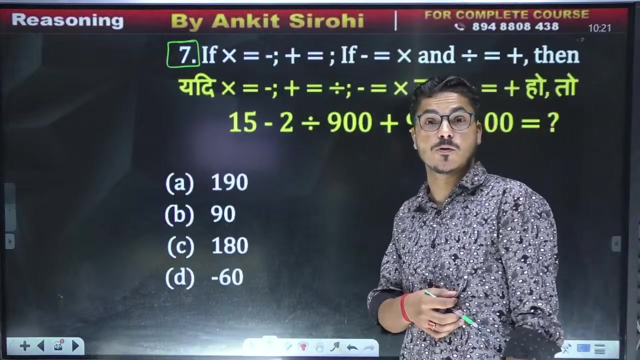 Right. No, dear brothers, only seventeen is the right answer. Yes, Do you see? the fault of all of you, my dear friends. the deceit of the eyes. the deceit of the eyes is nothing else. To be careful with the eyes. it takes its pride in anyone and tries to prove the right and the wrong to anyone. 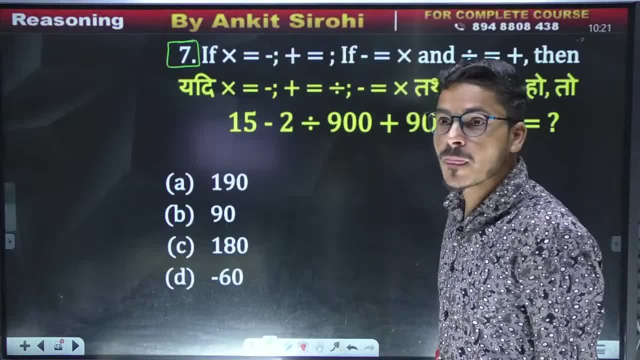 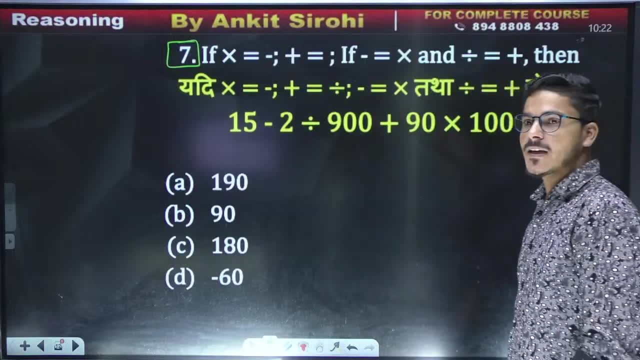 So you all have to decide, you have to understand and take it. Okay, no problem, I didn't look outside. come, come, Oh brother, very good, Come on, tell me the answer to this. what will happen to this? 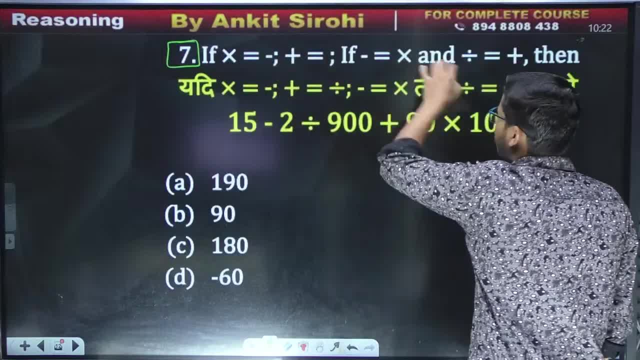 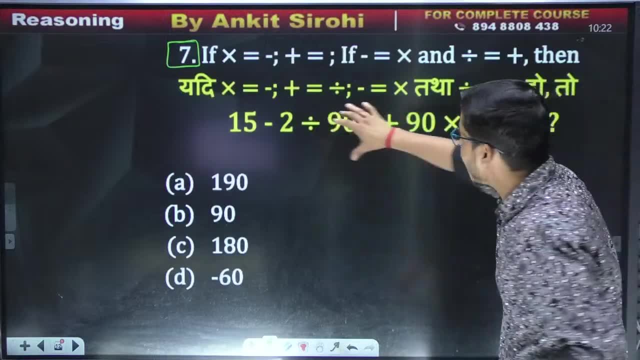 Means that the quality is equal. so much this, that everything is given. If, dear friends, you all made a mistake, Assume that this, dear friends, is the heart of a poisonous snake. The poisonous snake is sitting there. 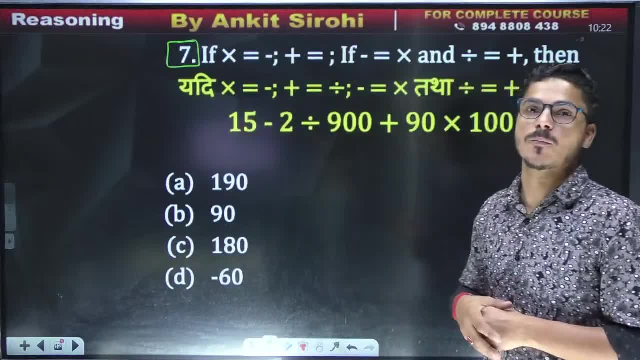 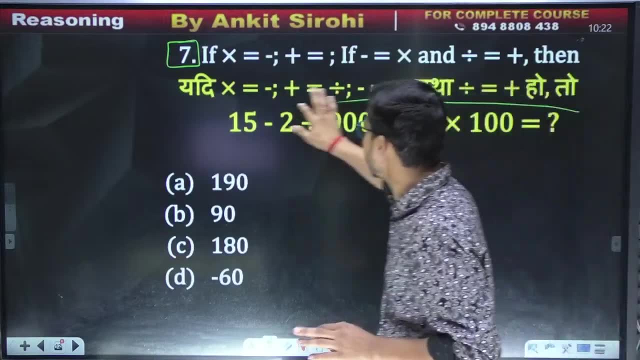 If you accidentally give it such a hand, it will bite you. There will be a loss. It means that if you do not pay attention to them, you put a board mask on it and, my dear brothers, If you have asked a question, then understand that all of you are your own. 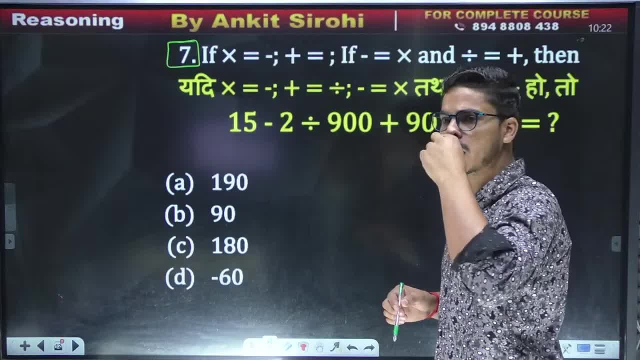 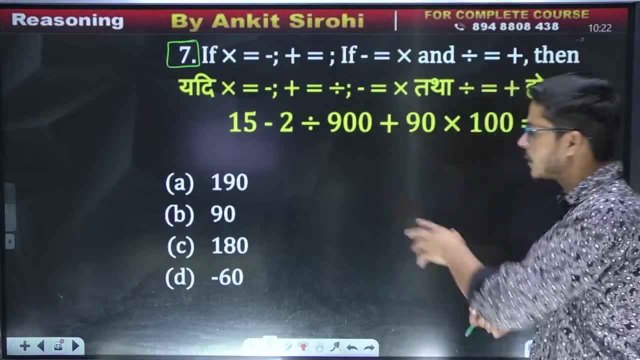 All of you have hurt yourself. All of you have hurt yourself, dear friends. So see, come quickly. Minus 60.. Minus 60, all, Oh brother, very good, There is absolutely minus 60 in the option. 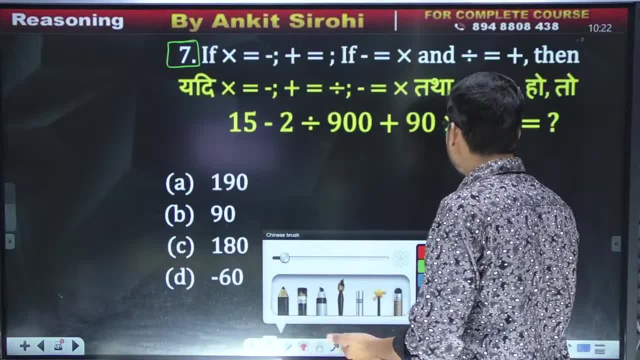 What will you have to do for that Easier question than this? What can happen to my brother? He said that nothing can happen. So come, at least give the answer. If it can't happen, then minus 60 has come. 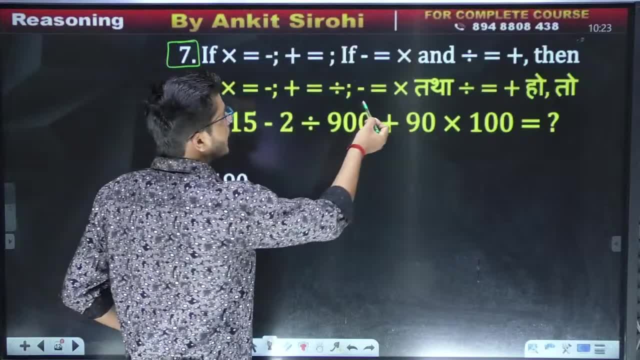 Minus 60,, minus 60.. See the meaning Minus. Oh brother, minus is equal to the quality. Take it, father. What is equal to the share. Give plus What is equal to the plus, My friend, 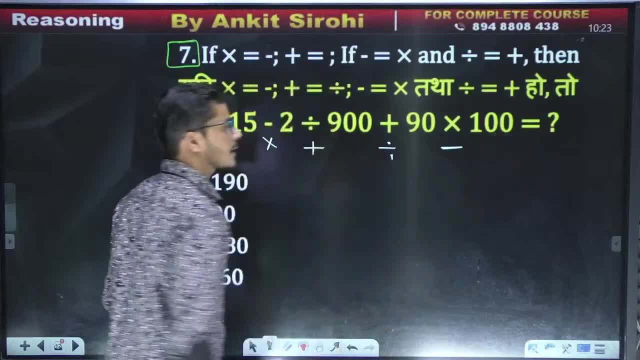 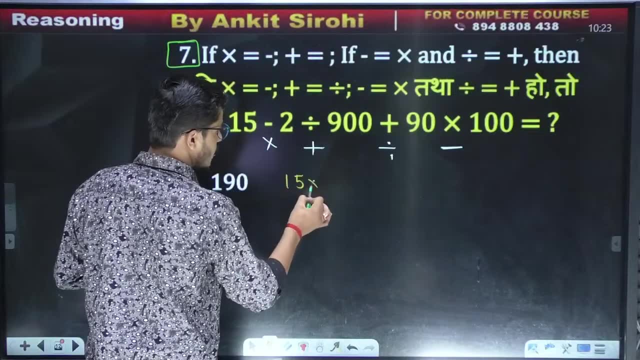 Take the share, And whose share is equal Minus What will be equal, So it will come to solve equally. Let's write What has become the equation: my dear brother, 15 times 2 plus 900, divided by 90 minus 100. 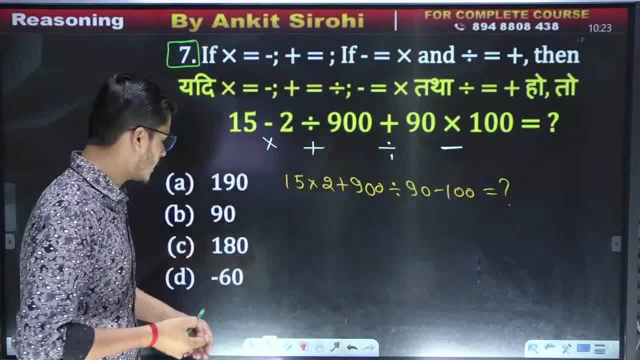 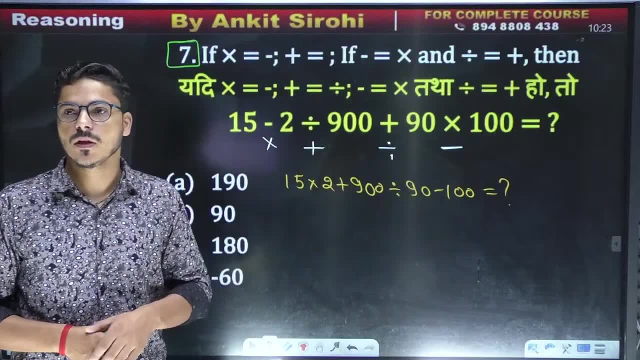 What will be equal. He said now, what do we do here? We will solve the equation in a very wonderful way. Minus 60 is very good. Good morning, You will see here. You know that the law of Baudouin says that first of all you don't have to do anything. 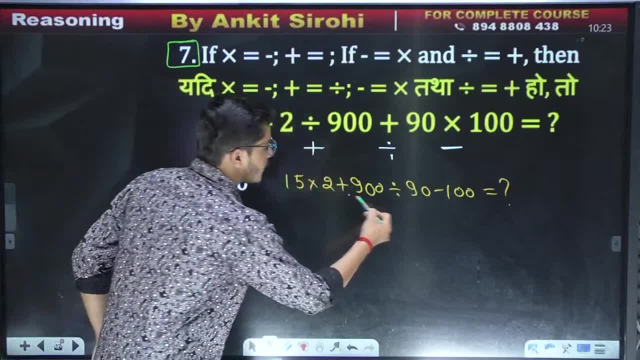 First of all, you have to walk on the stairs and divide here, So divide. So we found that if you want, you can multiply. When you do this much, you will understand that there is a plus in between. 15 times 2 is 30 plus. 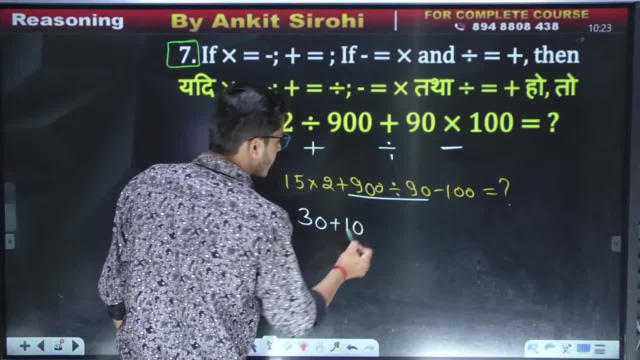 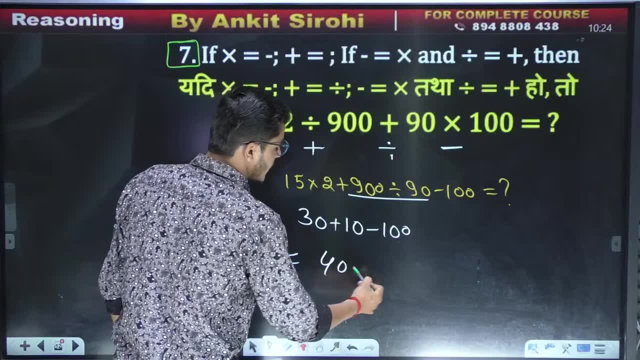 In 900,. if you run away from 90, then, my friend, how many times 10 times? How many times is it 10 times Minus 100.. So Who will be equal? 30 and 10 are 40, plus and minus is equal to 100. 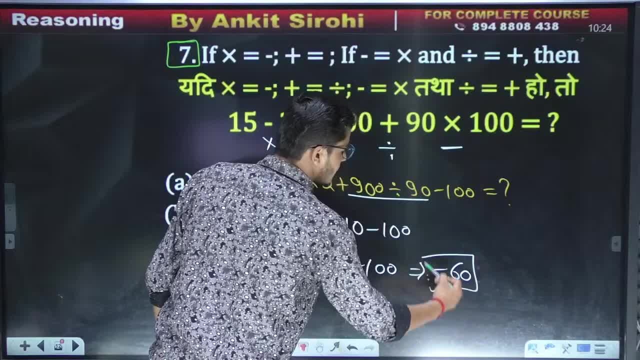 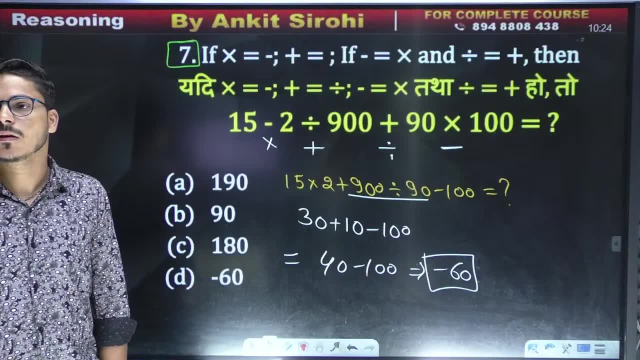 So he said, if it decreases, then who gets the sign? The big number? Now, who was the big one here? So, So minus 60 will be the right answer. Absolutely, dear friends, A little, Okay, let's go. 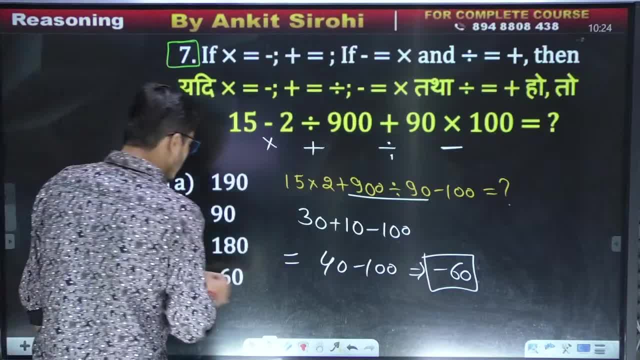 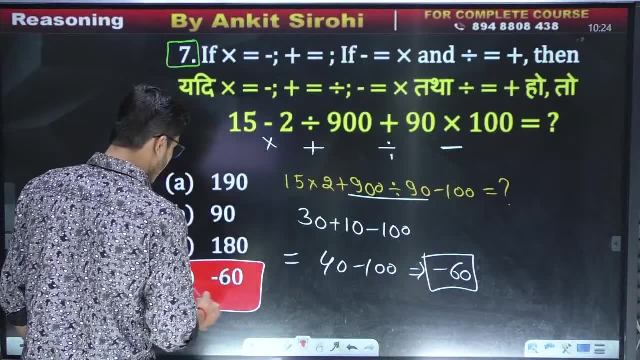 No problem. So minus 60.. My dear friends, Minus 60. here, Dear friends, Our answer will be absolutely correct. Minus 60 will be correct. Okay, dear friends, Very good, Very good. B gave you a very good answer. 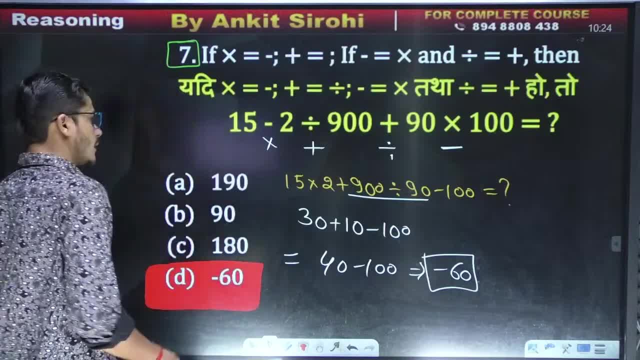 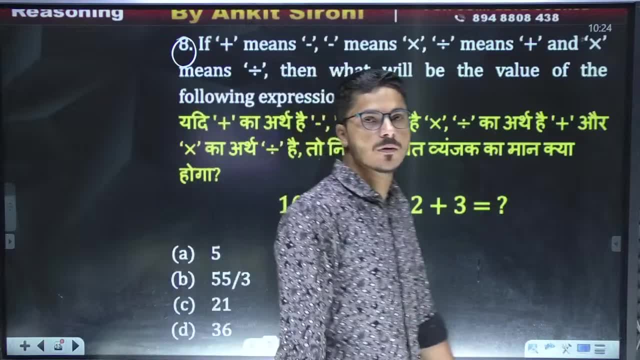 Let's go In the next class, when his class number will be 2, then, my dear friends, you will see, I will try to ask you good questions. Yes, yes, Yes, Yes, Yes, Yes, All right, 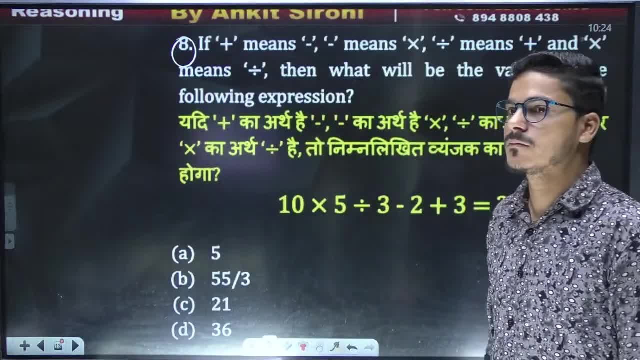 Okay, friends, Let's go. Come towards the third level. Yes, it's okay. Yes, Yes, Decir, tell the dear friends quickly that what will be the answer to it? Minus 60 is a very, very good answer. 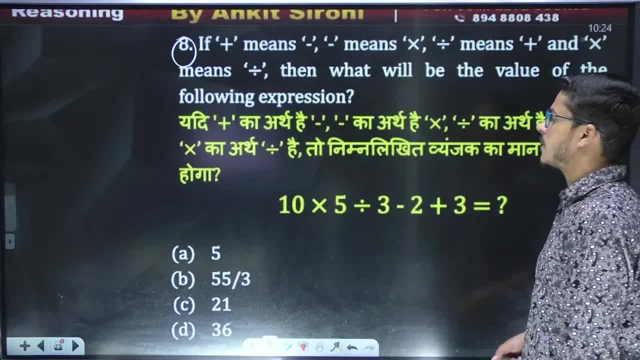 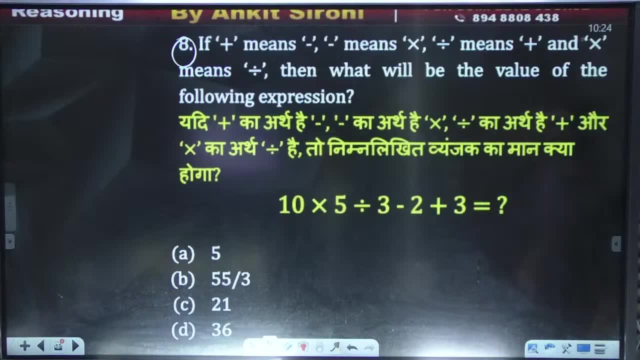 The next question is in front of you: 8. He says: the same thing has also happened in the last presentation, The same thing happened in the last question. The same thing happened there as well. Is, brother, what the matter is here? 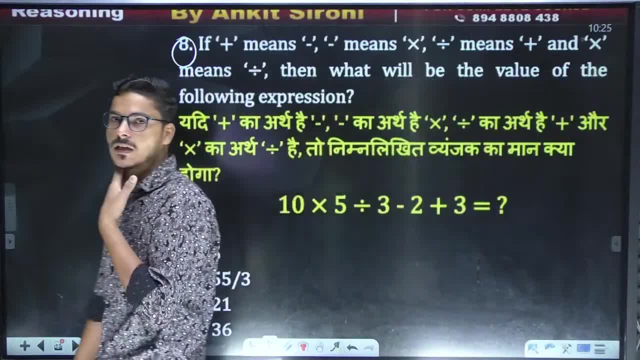 What is the matter here? guns jumper Guys, you have to give you, All of you, That. what will it be, dear friend? What will be the gun, Barbie, As I protect it from enemies. Tell everything, Jackie, All of you, tell me quickly, we will see. 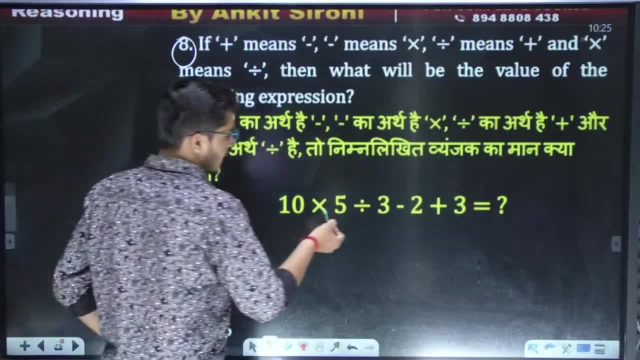 Here you don't have to do anything. at the place of plus, the meaning of plus will be minus, and then where there is a plus, you can do minus. Minus means that there is an old man, you can do the old man here. 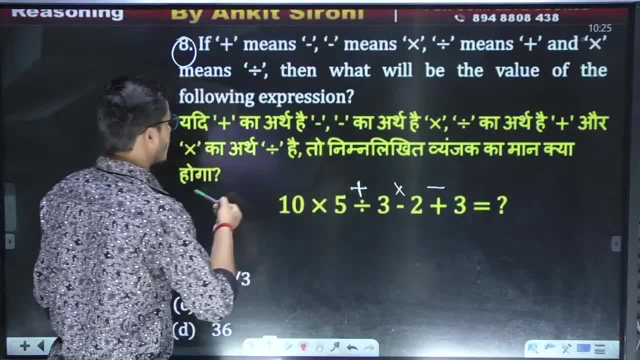 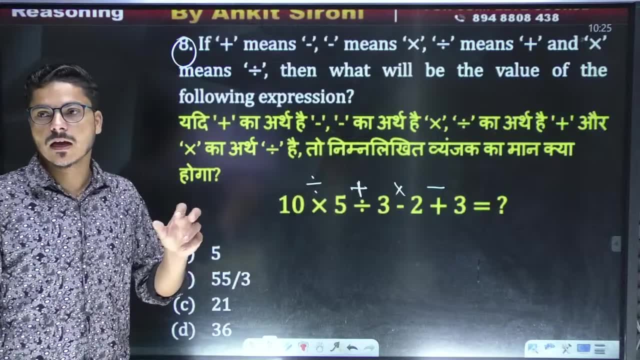 The meaning of the old is that there is a plus, my dear friends, you can do the plus. And the meaning of the old, my dear friends, is that the old is gone. Now let's solve it all together When we solve it here. my dear friends, the status of G has come 5.. 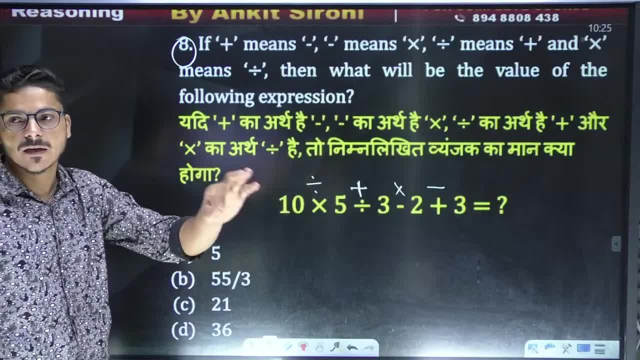 How much 5 has come, my dear friends? okay, okay, very good, Everyone's 5 has come. so it means that the voting of 5 is more, so it means that the possibility of it being correct is of a very good level, see, 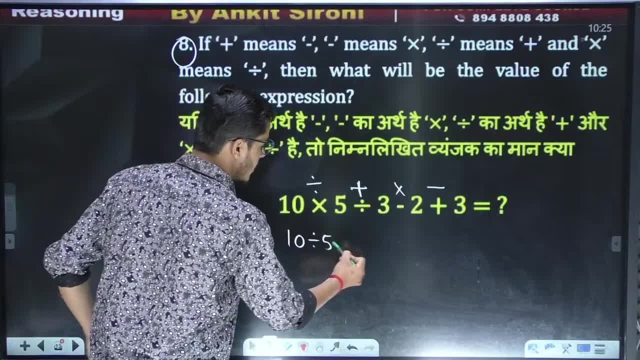 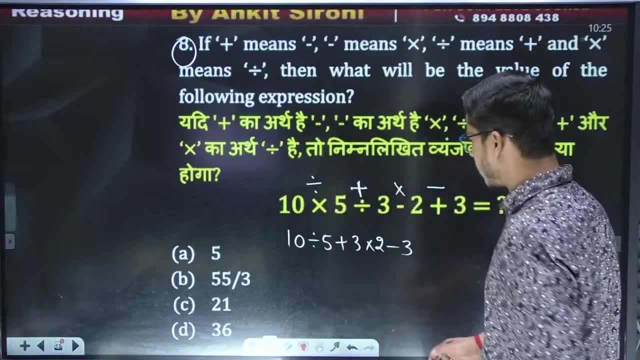 What we have to do here is that 10 divided by 5,, my dear friends, plus 3 multiplied by 2 and minus 3, that is fine. So what to do now is that nothing has to be done. the board mass is not used. the board mass says that if you divide it first, then the number of friends is 2.. 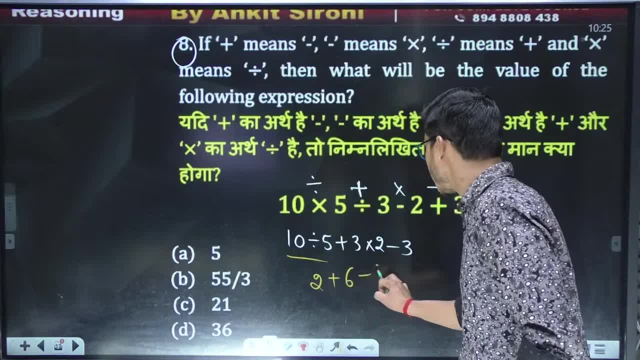 You said that it is fine. plus 3 divided by 2 is 6 and minus 3 is the number of friends. He said 6 and 2, in 8, he said 3 and he said 5.. So what is the result of this? 5.? 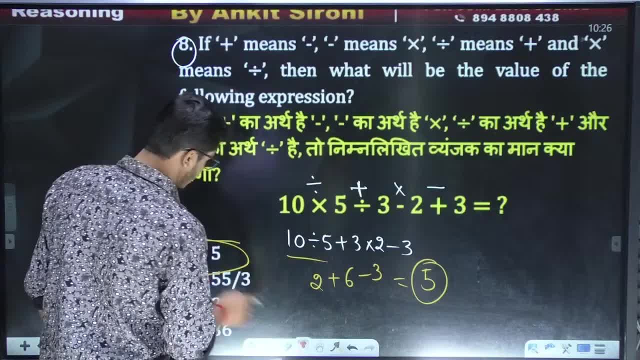 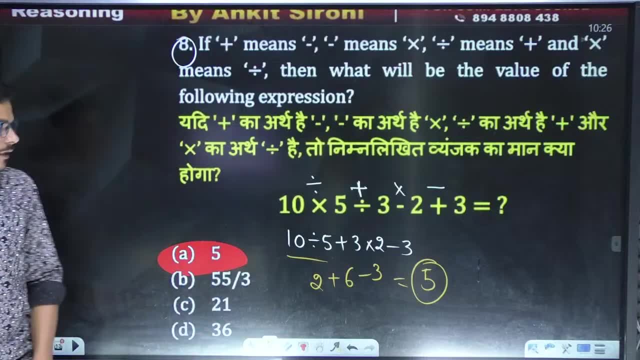 Is there 5?? So see, my dear friends, to scare you all, 55 divided by 3 is also written. such a big number, 55 divided by 3, is also written, so that some confusion will go in your mind: brother, how much can it be? 55 divided by 3 will also be. its correct answer will be 5.. 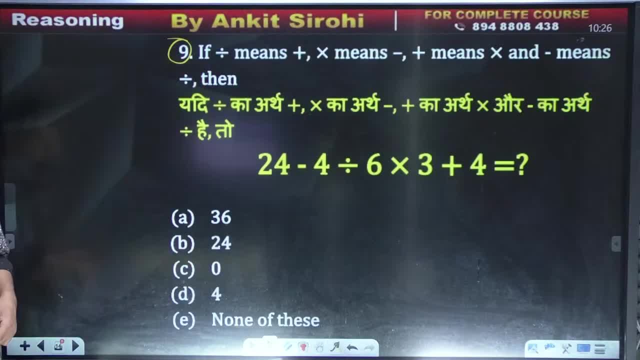 In the meantime, 9 questions have come in front of you all, My dear friends. 9 questions have come in the meantime, in front of you all, Isn't it, dear brother? The correct answer of all 8 was 5.. 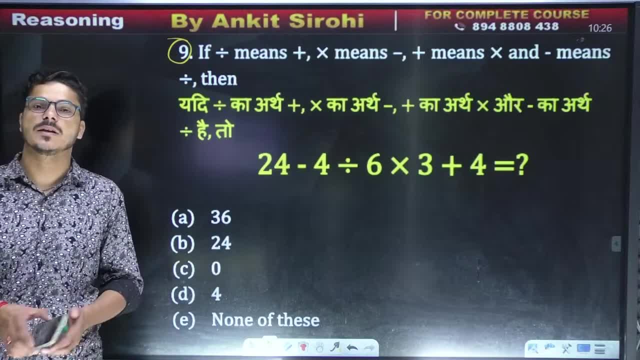 What will be the correct answer of 90 questions, my dear friends? tell you all quickly, brother, what will be the correct answer of this? Quickly, my dear friends, If you like the class, then bring it. If you like the class, then definitely like it. 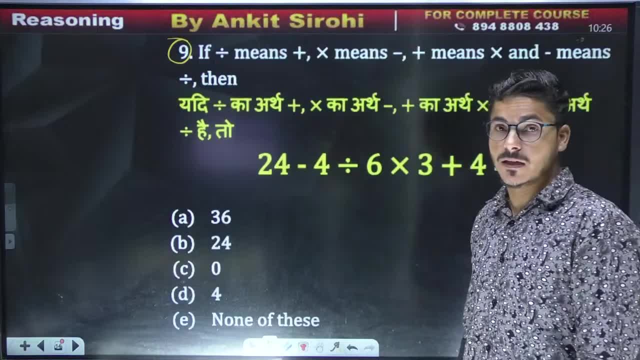 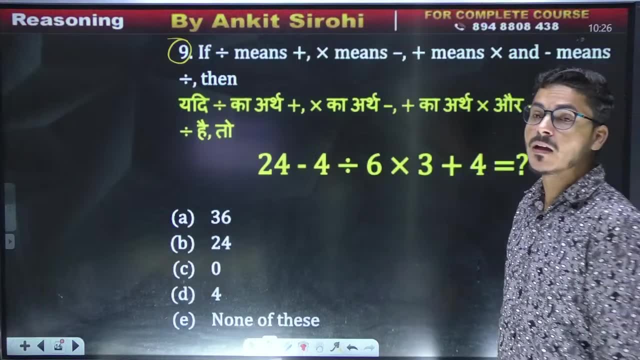 Otherwise, it is your wish And, dear friends, like it or not, but subscribe to the channel Because, dear friends, the notification will reach you very fast, In which, dear friends, you will know that, yes, brother, come here. the class has started quickly. 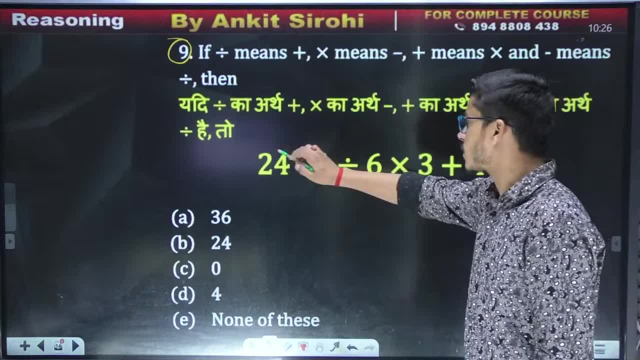 See if the meaning of the part will be: my friend, plus, Keep this thing here. The meaning of the part is: plus, Keep it. The meaning of the part is: plus, Keep it my friends. Here is the plus. 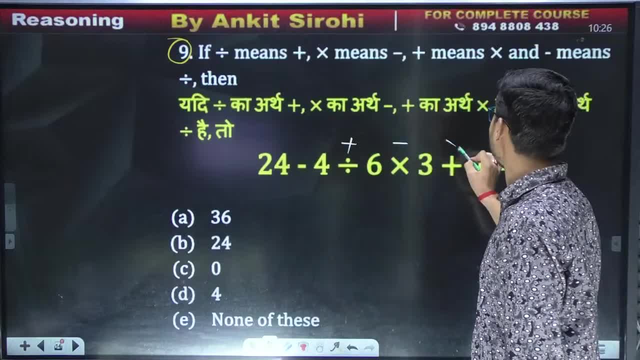 What is the meaning of the value? It is minus. What is the meaning of the plus? It is the value. And what is the meaning of the minus? It is the part. So, dear friends, now it has become in the form of a new semicron. 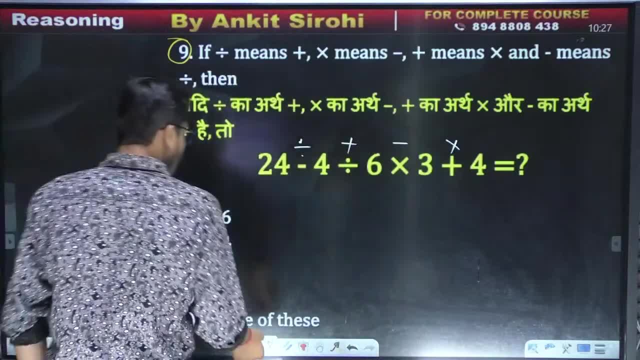 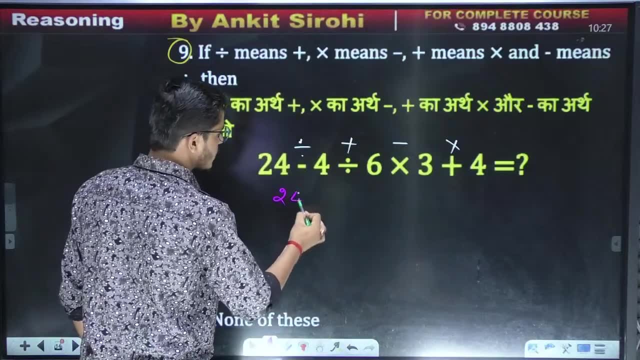 So the answer of zero is absolutely perfect. It is perfect. Take a look. We check whether to listen or not. Here's how we will ask questions. Our question will be 24, part 4 plus 6 minus 3 and multiplied by 4.. 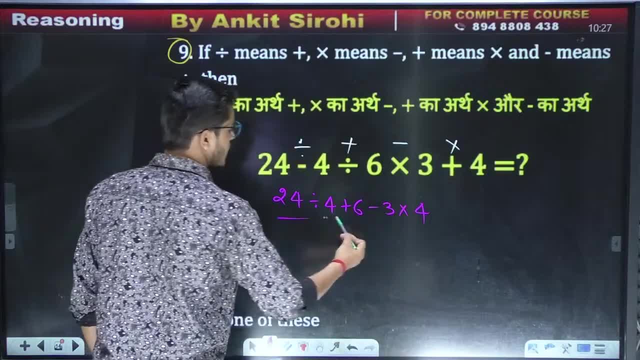 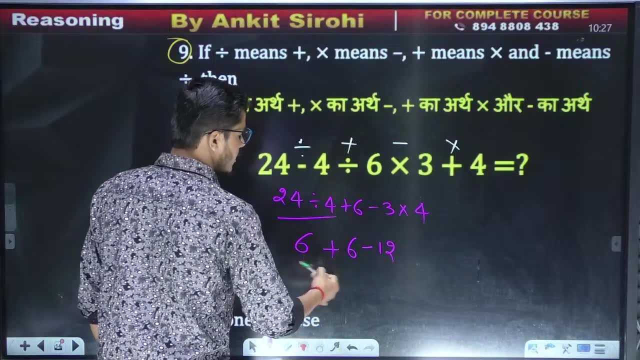 So say: first we will use the board mask friends, First we will do the part. So how many times did it go? Six times Plus six minus 4 is 12.. You see, 6 and 6 is 12.. 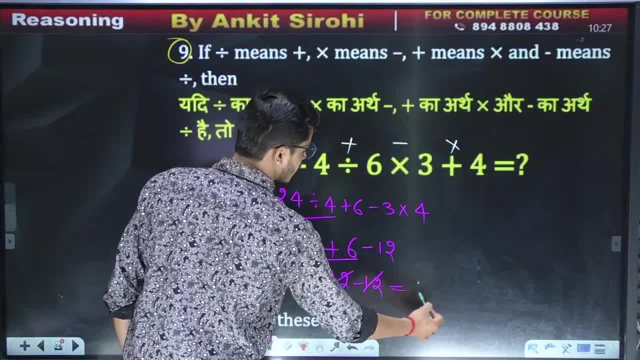 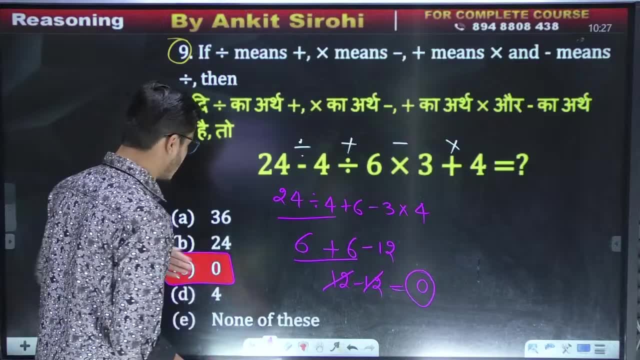 You all know that two numbers are the same: one is of plus and one is of minus. so cut it and it is obtained in the form of zero. So its option number C will be absolutely correct: zero. Dear friends, whoever has given zero, the answer is absolutely perfect. 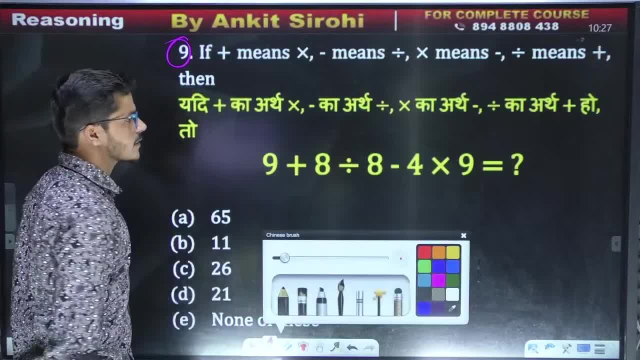 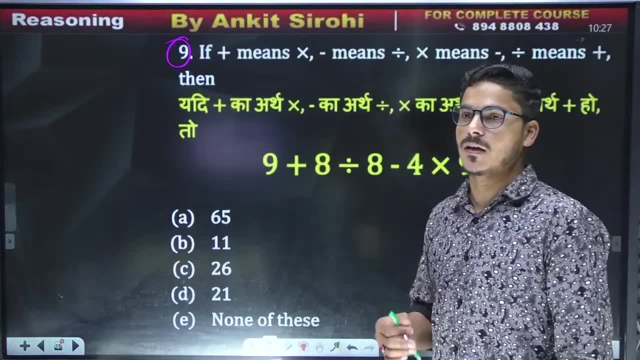 There is a new question in the middle. If you see, here too it is exactly the same question. If you see, you have brought a lot of such questions in front of you all, but still you are not answering. Why? What is the reason? What is the reason? 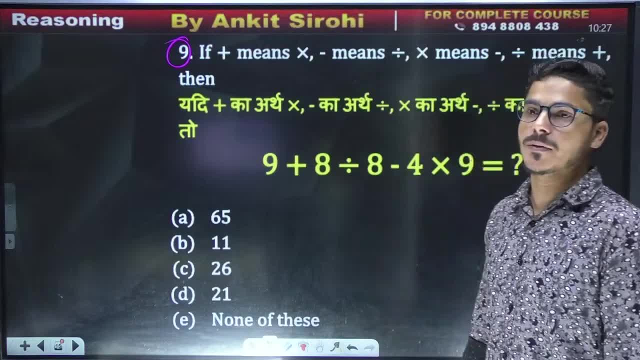 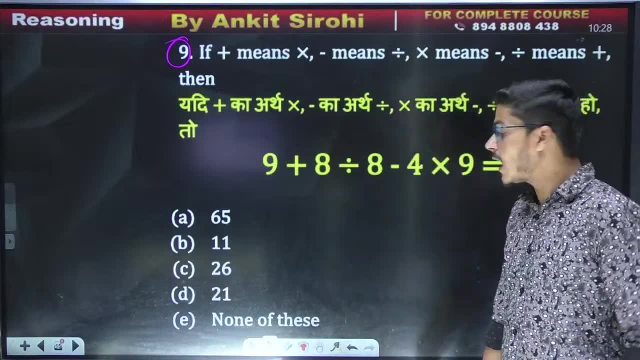 Dear friends, it will be zero. Why is your calculation slowing down? Why is it not fast? Okay, the color of the pen is not looking good. Okay, let's change it. See here, dear friends, what has been said here. 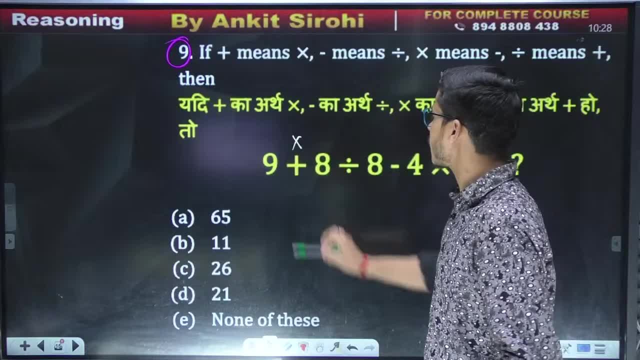 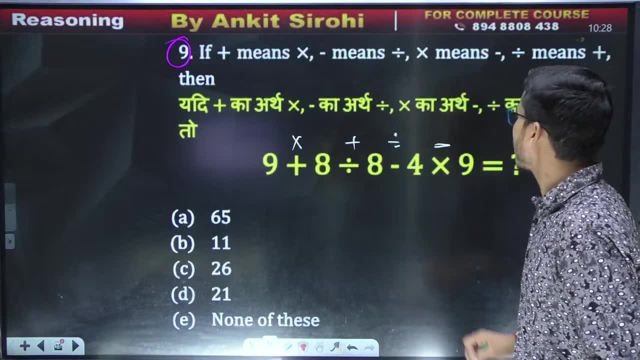 Whatever will be plus right. What is the meaning of plus? It is equal. What is the meaning of part? It is a plus. What is the meaning of minus? It is a part. What is the meaning of equal: It is a minus. 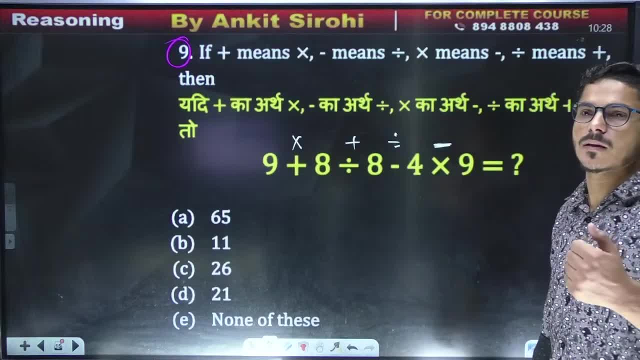 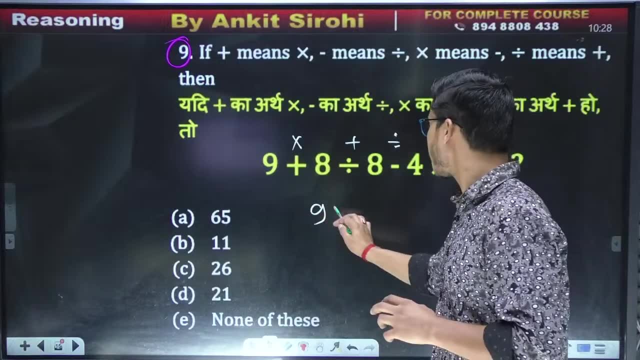 Now, here you all have to see what will come in the place of the question after solving it. Our task is to solve it first. Dear friends, let's solve it First of all, write the equation correctly. Here it will be 9 times 8 plus 8.. 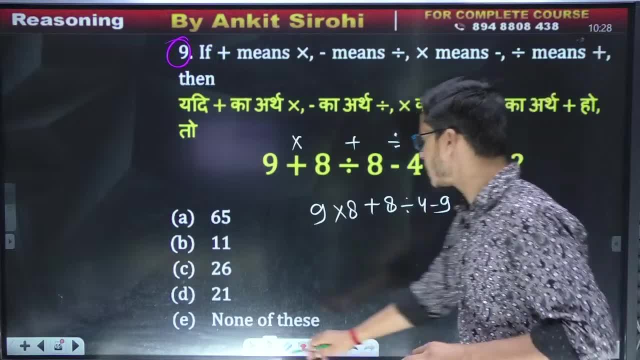 Dear friends, it will be a part of 4 and minus 9.. Okay, my dear friends Say yes. okay, Let's move forward and see what will happen, Dear friends, what will happen After solving it. do it like this: plus. 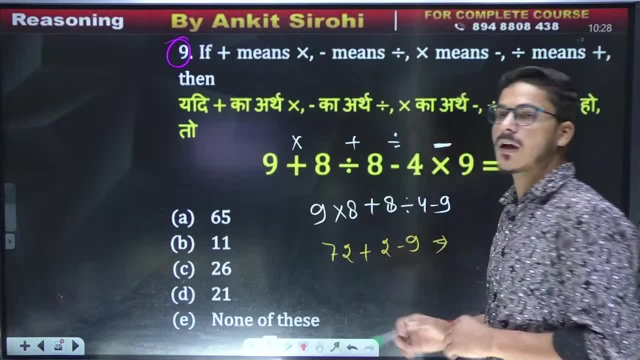 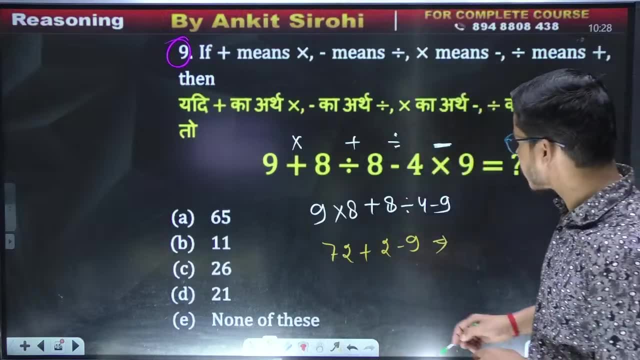 You will see twice and minus 9.. Now tell me, dear friends, how much did it come? Did any of the dear friends come? Okay, there is no problem, Calculation is done. Okay, no problem, It happens. Just keep in mind, dear friends, that it is a game of calculation. 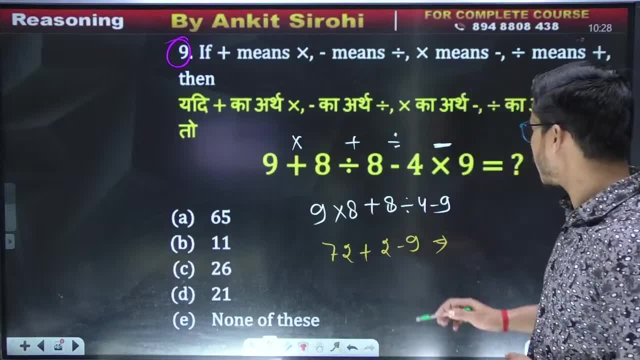 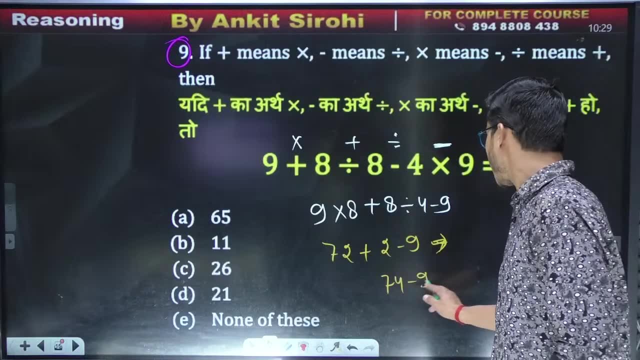 Isn't it? It is a game of calculation, dear friends. Let's go And see. the offline papers are also dangerous for them. Here you see: 72 plus 2 is 74.. Out of 74,, dear friends, when 9 goes, then you all know that you will get the result in the form of 65. 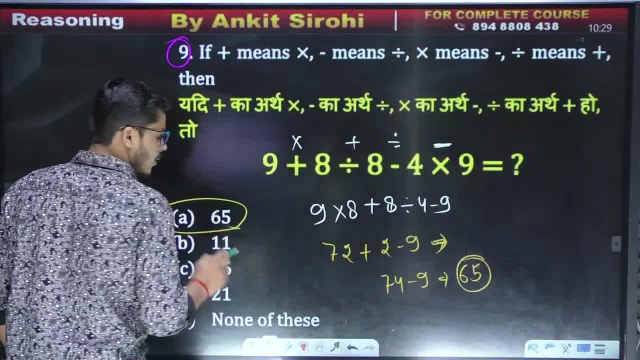 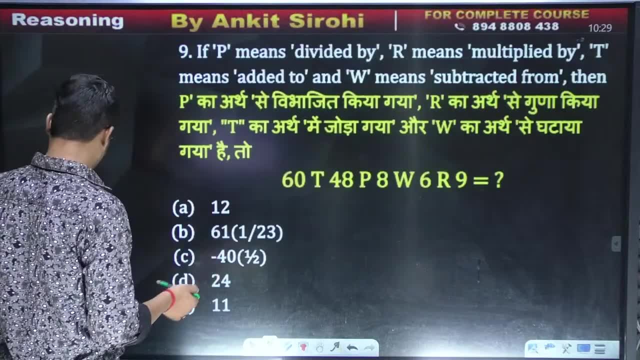 In which form? 65. Where Option number is the same 65. Okay, So 65 will be the correct answer. Dear friends, very good. In the meantime let's go Question number. Oh brother, Come on. 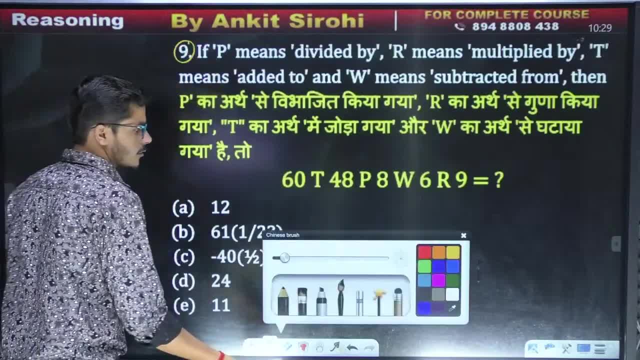 This is the tenth. Okay, it is the tenth. Let's assume it is 9.. They may not be able to make any changes in it. Come on, Come on This time, dear friends, this time some different level has been shown to all of you. 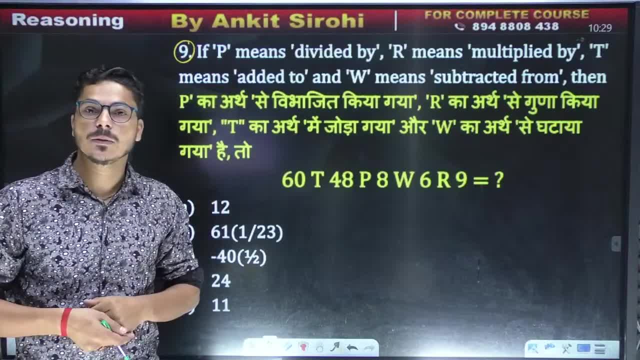 What has been done here? A summary has been given, But this time there is no sign here, There is no star Here. your alphabet is present in the middle. Now, the alphabet is present. Reena ji was not 9.. Reena ji, how were you saying? 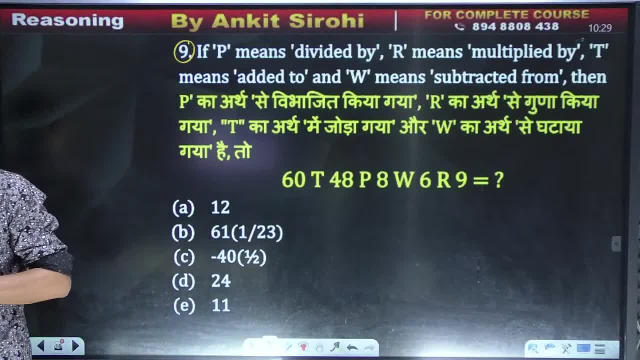 9.. What are you saying, Reena ji? Yes, 65.. Okay, 65 of 9.. Write it like this: The whole thing will be 65 of 9.. I got scared at once. It will be 65 of 9.. 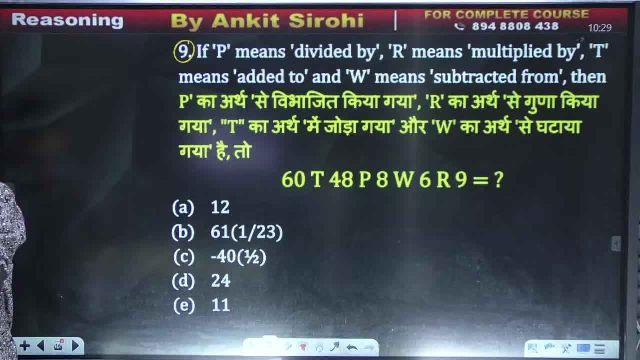 Dear brother, Absolutely, Come on. Will it be 65 of 9 or not? Come on, Let's go ahead, Let's see here. Okay, Now I think 9 has come three times 8.. What is this, my friend? 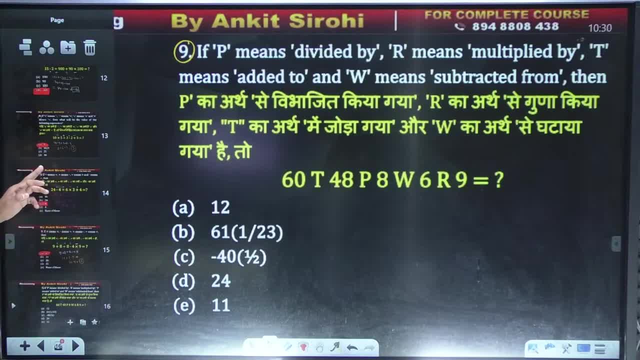 To listen to 9.. Are you seeing? The master has written 9 three times. He has written only 9.. Come on, This is done, my friends. Our question has come This: 9., 10., 11.. 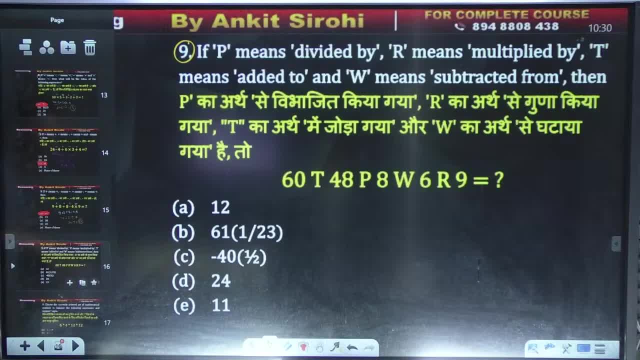 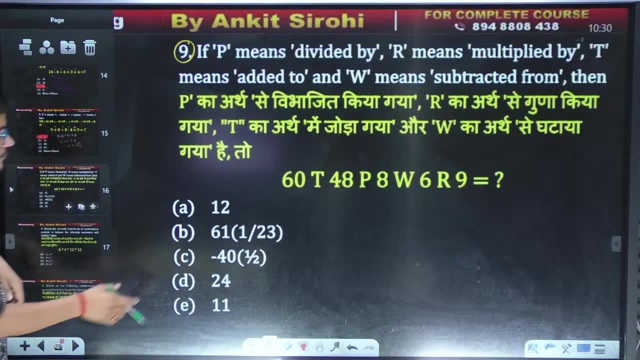 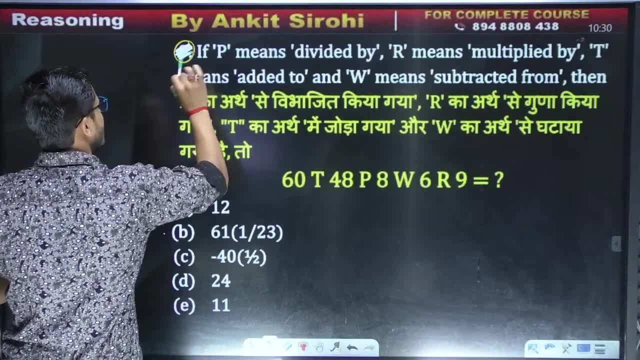 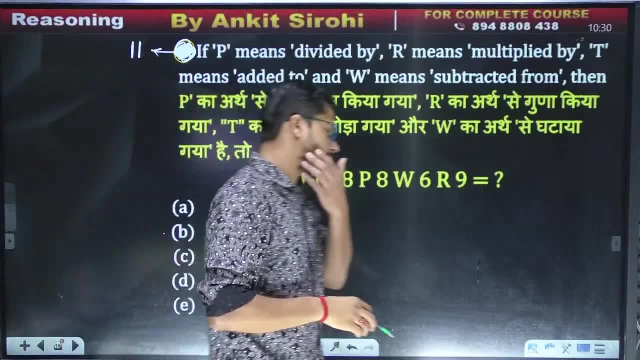 This is 11.. 11.. This is 11.. This is 7., 6., 7., 6., 7.. Definitely nothing. Six, 11., 17., 2., 2y y 3.. 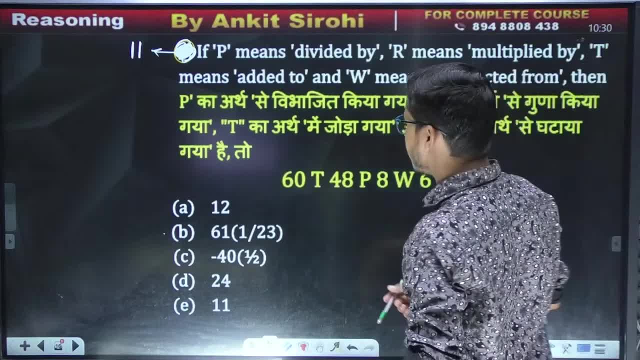 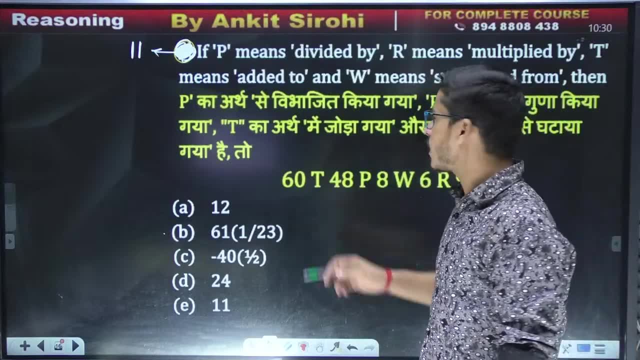 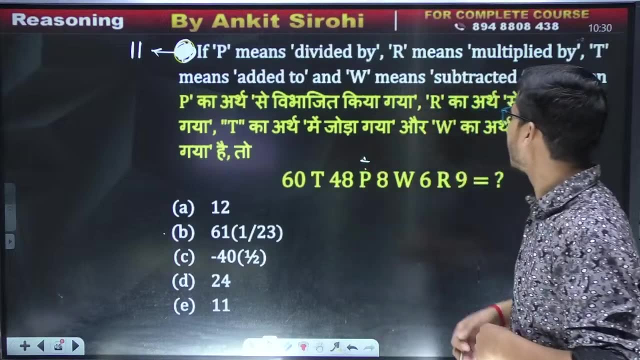 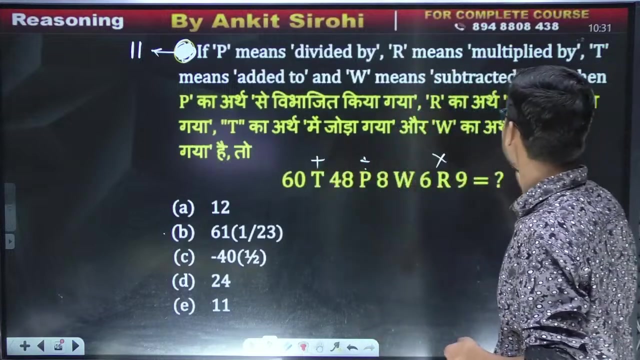 2., 2. 2h. 1., 2., 2., 1., 2., 2., 3., 1., 9. 9. 1. 6.. divided means multiply, t means to join and w means to subtract. 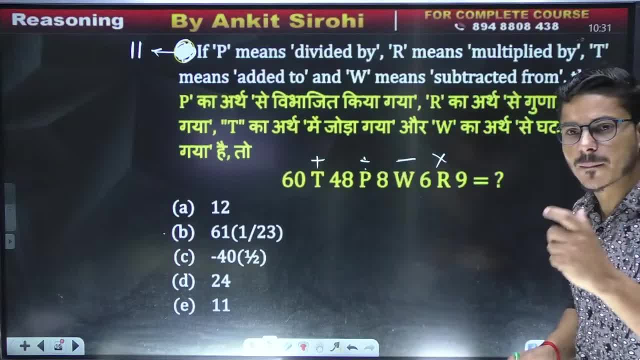 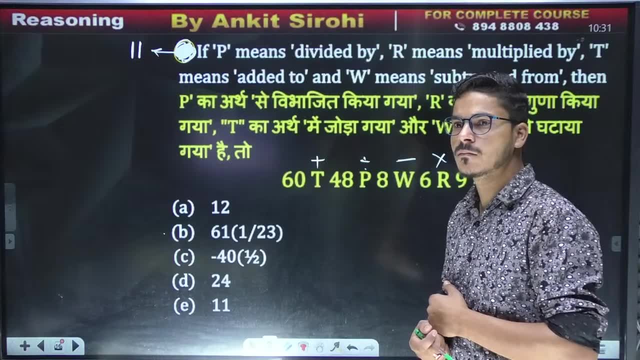 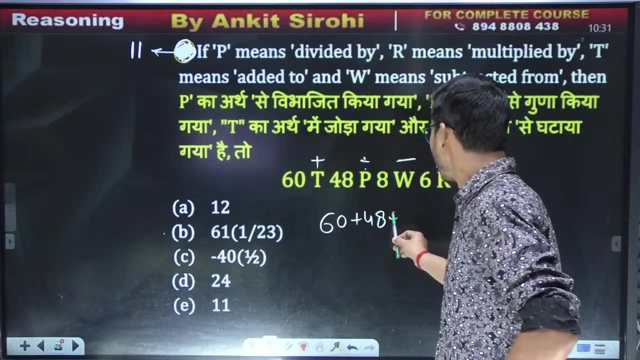 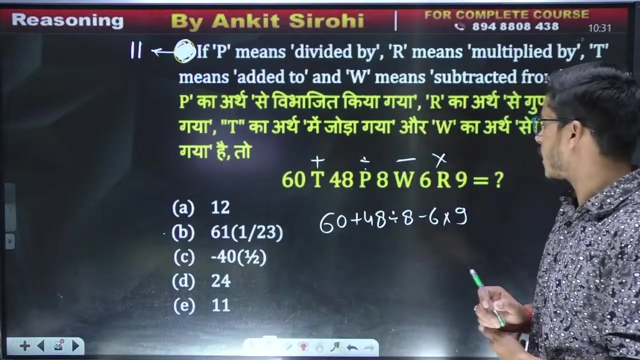 here we are at the place of all your marks. ok, here you see, my dear friends, for you all, 60 plus 48, and first brother. divide 8 minus 6 times 9. this is written. so first, friends, you all have to do one thing: first of all, use the board mass rule. the board mass rule says that first of all we have to divide. 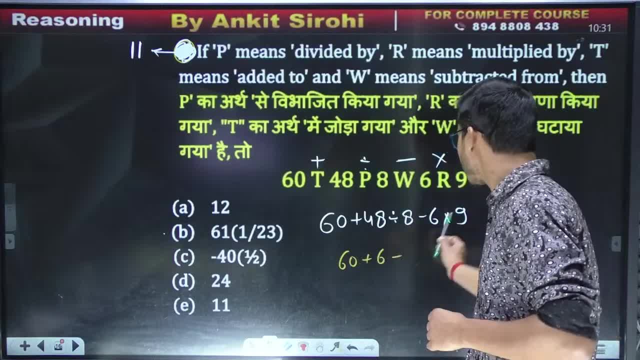 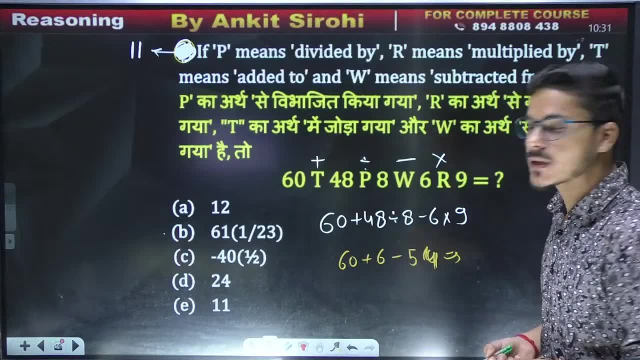 8 times 6 is equal to 48. so 60 plus 6 minus 9 times 6 is equal to 54. ok, friends, if you see the result of this, you will know that 60 plus 6 is equal to 66, and if we go from 66 to 54, then 12 will be left. so 12 will be my correct answer. 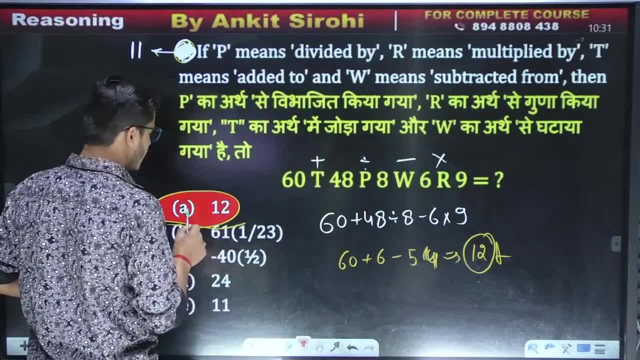 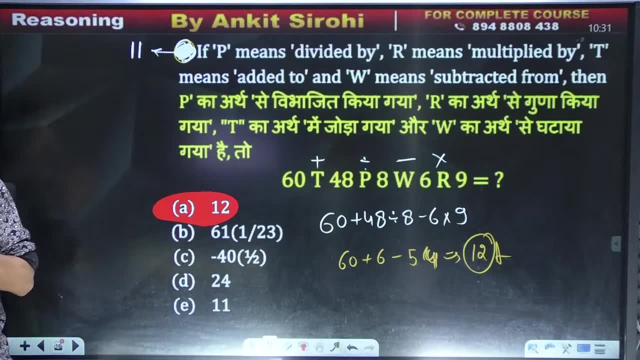 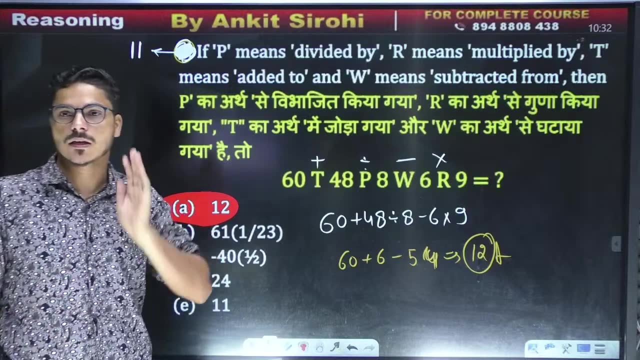 option number a, you will see 12. here you will see first friends. here you will see 12 and 12 will be absolutely correct with me, ok. ok, brothers and sisters, what is the class of the class? Pratiksha ji rpf. railway class is going on after this. 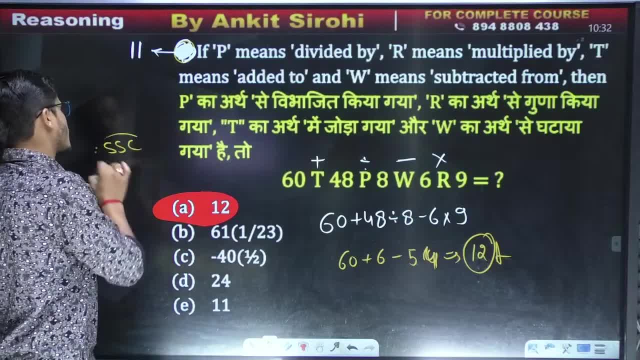 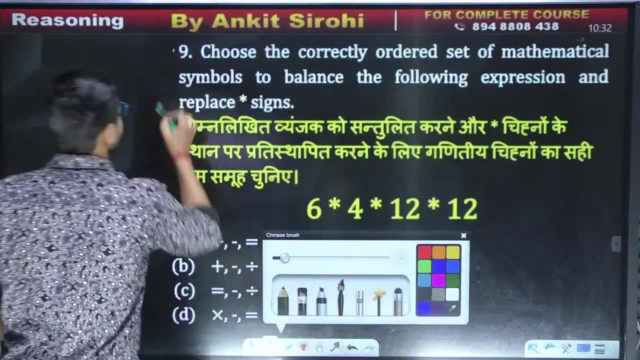 on which family is it on lab, ssc lab. ok, i am present there today. we will go there. blade relation 2. let's go in the meantime. brothers and sisters. what will be the question of number 12, brothers and sisters? which 11 is correct in the meantime 12? 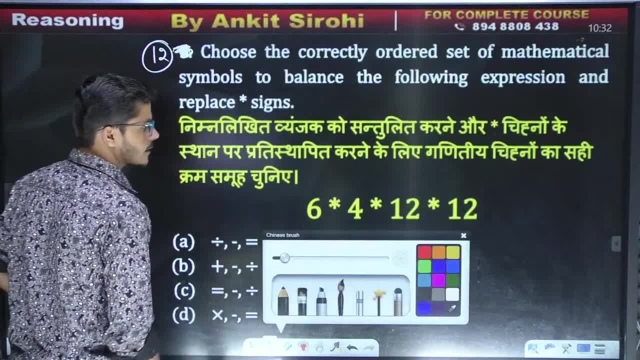 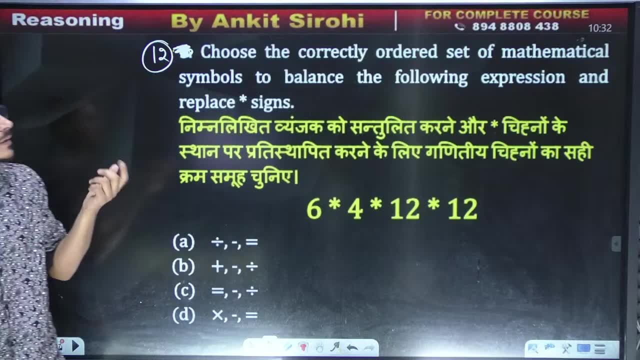 what will be the correct answer of the question? tell 12 dear friends. what will be the correct answer of 12? see quickly that. come to the place of these stars. and, dear friends, what does it do you have to tell all of you here, after the symbols, come, dear friends. 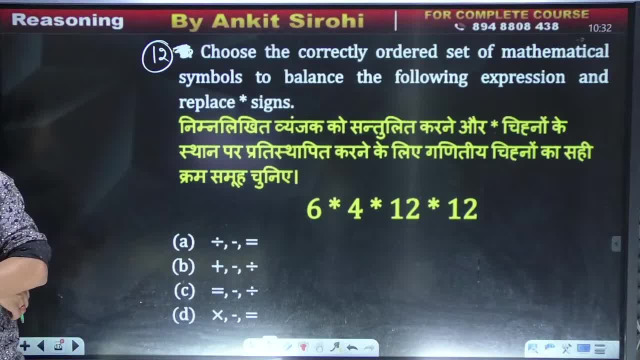 what will happen. choose the correct order of the numbers so that we get in the form of LHS Paravara, LHS 24 of the previous one was 24. yes, no, dear friends, it will not be 24, remember it, it was 24. wait a minute. wait a minute 28. 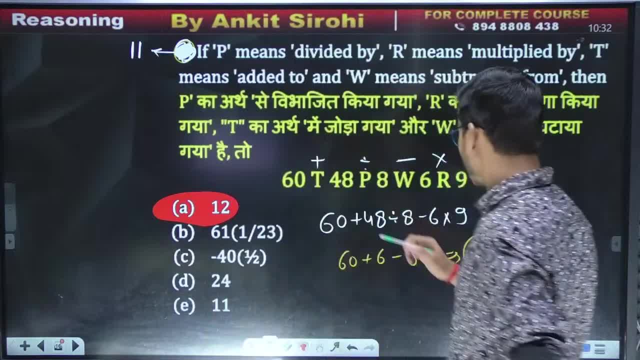 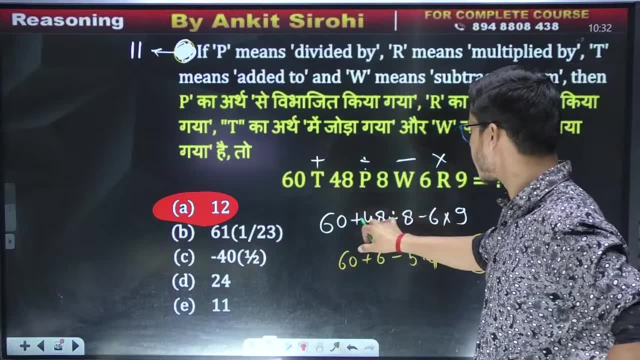 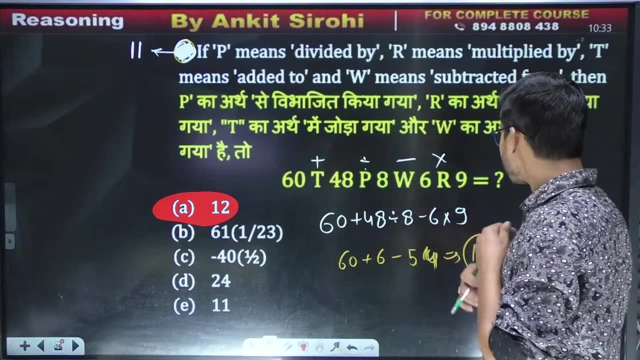 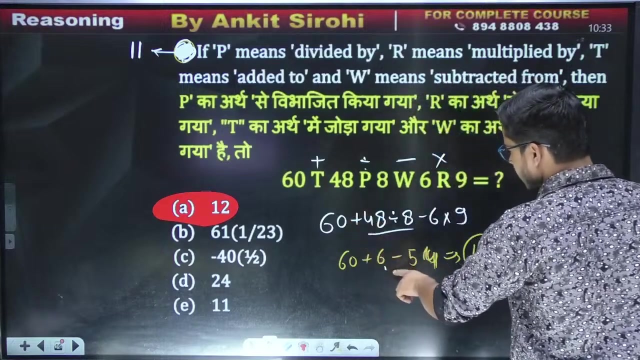 how much is 24? i will give you eight. ging are 48, 66, 60 such times plus. gave 48 part 8 W bank minus 6 x. write radius statement. come in 48 category. 48 was 18 Garar 64, 60 plus 6 minus يا. 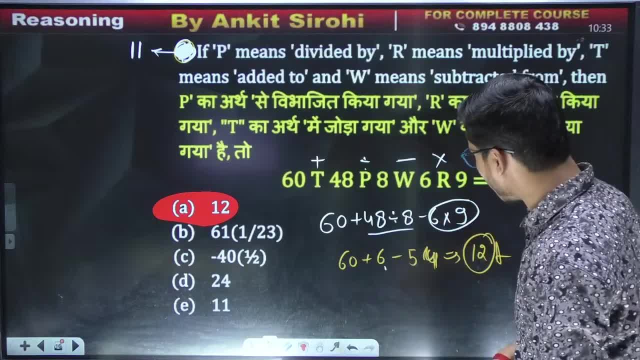 After that, the value of 9,, 6,, 5, and 54 will come. So, first of all, friends, 60 and 6 are our 66. If we go from 66 to 54, then how much will be left? 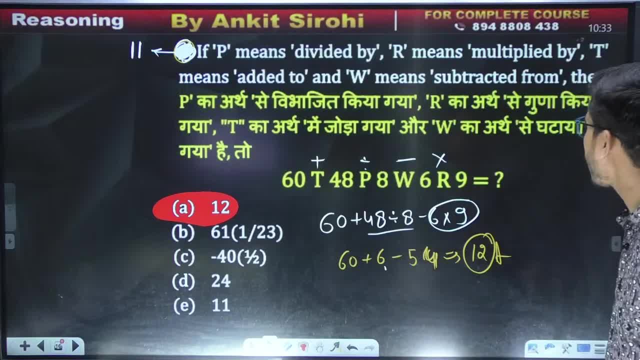 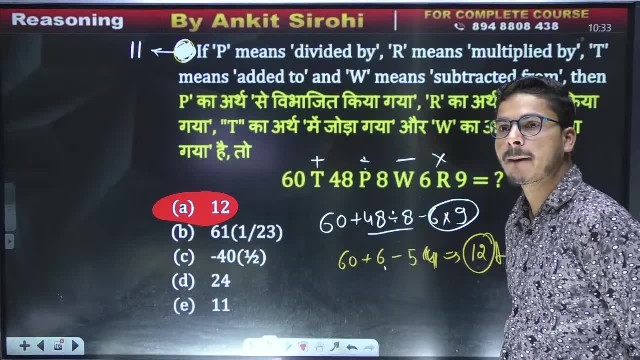 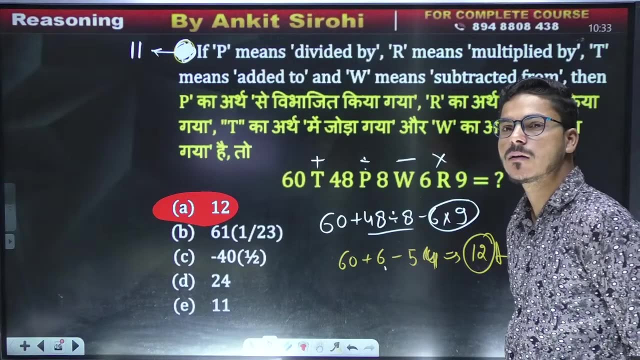 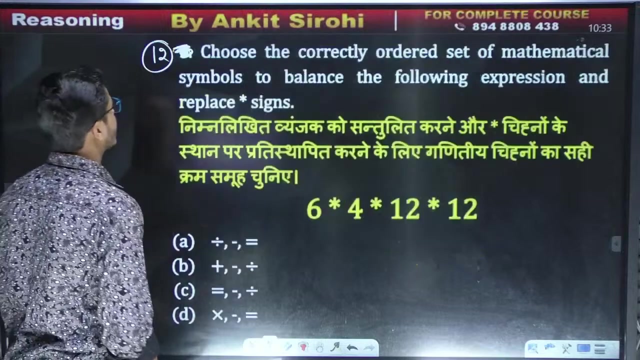 12 should be left. How is 24 left? How is 24 left, Arsha, tell me, how is 24 left? Come on, tell me how is 12 left. Okay, how is 24 left, Arsha, tell me. let's see, we have made a mistake once. 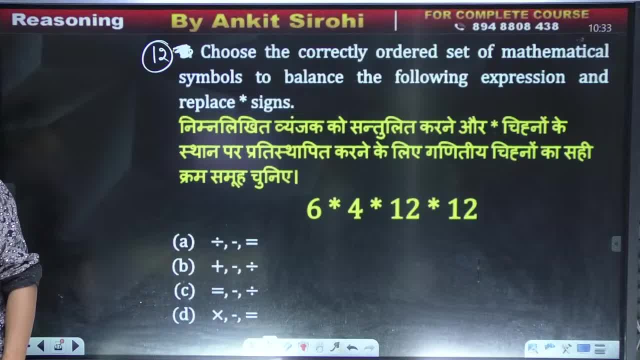 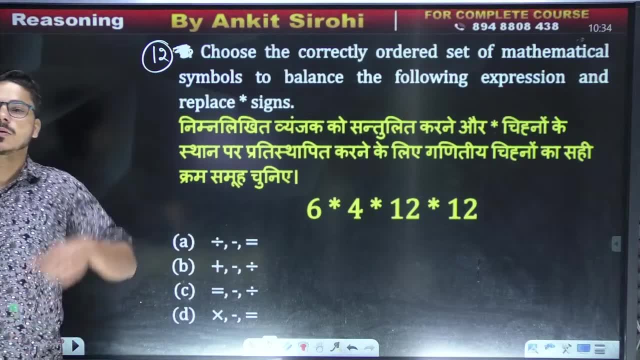 Right, See it quickly. There is no mistake at all. friends remember, Right? Okay, you check it once. See it, My dear brother. what was the 12th question? What was the 12th question? See it. 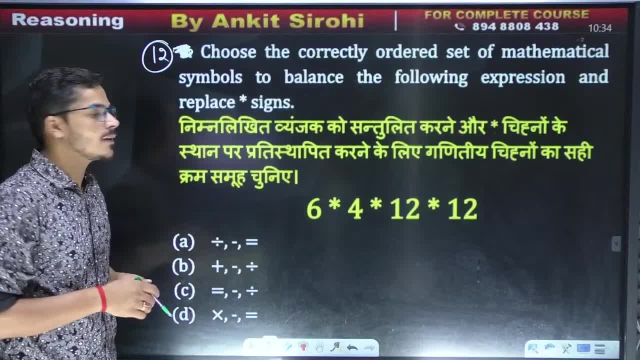 Did anyone answer here? It must be 12.. Yes, absolutely. What will be the 12th question? See the correct answer In this place. dear friends, what should we use so that, dear brother, we get a equation in a balanced way? 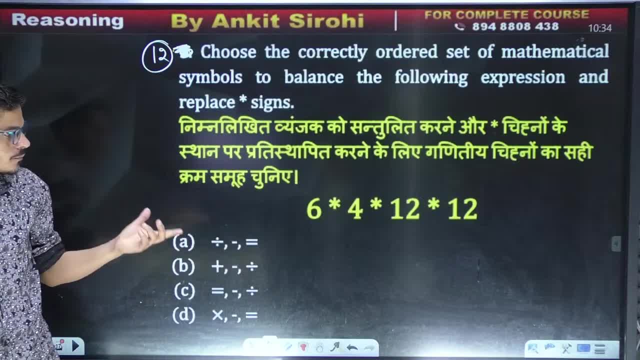 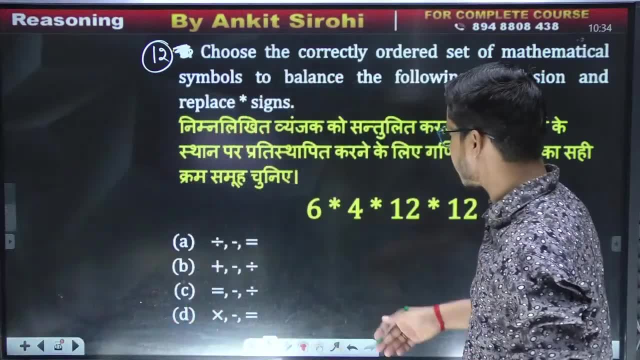 So that we get a equation in a balanced way. He said, okay, what will we have to do to get a equation in a balanced way? He said: first of all, what should we do? He said, okay, Now let's start from the bottom. 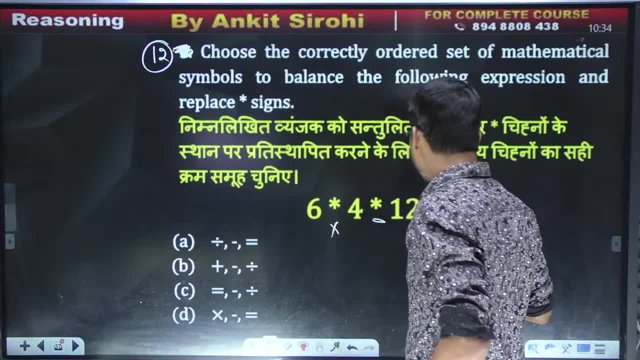 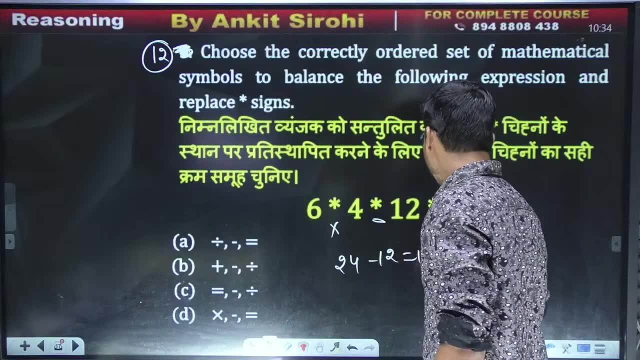 So here you will see that the value will be minus and equal Means. here, dear friends, you will see that if 64 becomes 24, he said: okay, minus 12.. Equal to what 12.. So how much did we get? 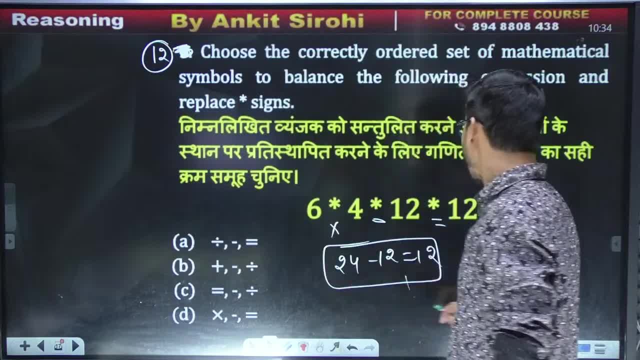 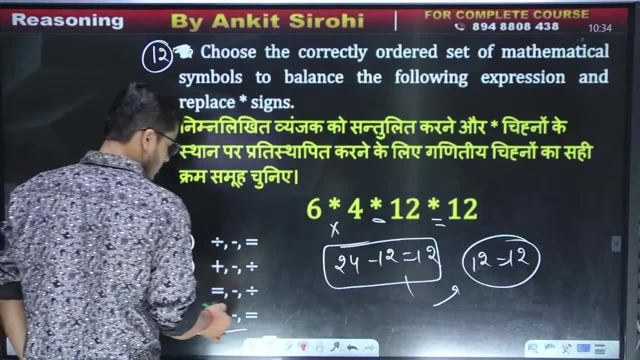 24 minus 12 is equal to 12.. He said 12.. So to say that it is equal to 12, by whom has it been proven? The symbol that came on option number D, which is our group symbol, by which, dear friends, it has been balanced? 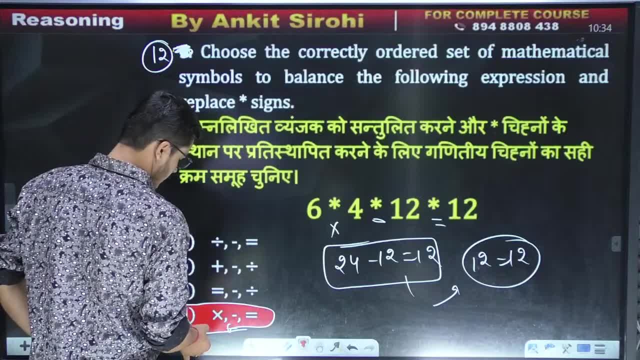 When it is balanced. dear friends, here you all sent a good answer to it. What is the correct answer to this? Come on, dear friend, the correct answer to this will be option D. It will be exactly D. Oh my God. 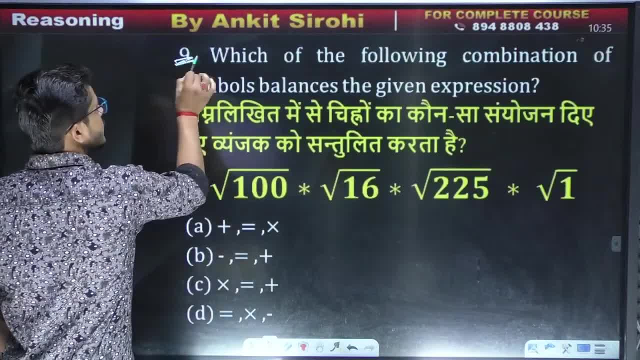 Let's move on to the next question, Question number 13.. What is it? Question number 13 will be in front of you all. Which one will be my first friends? Question number 13.. Question number 13.. Question number 13.. 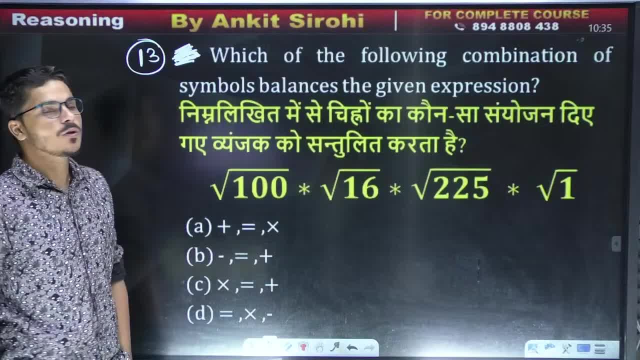 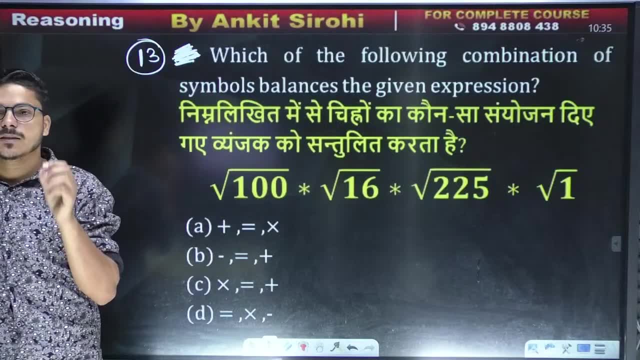 So you all will give the answer to question number 13.. Dear friends, what will be the answer to question number 13?? Brother, it is a very wonderful question. I will tell you that the logic of all of you here will seem very irresponsible. 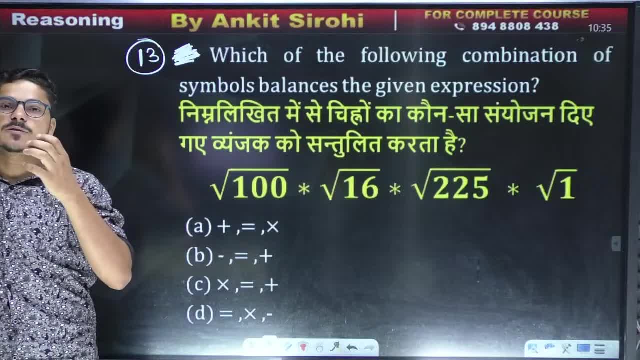 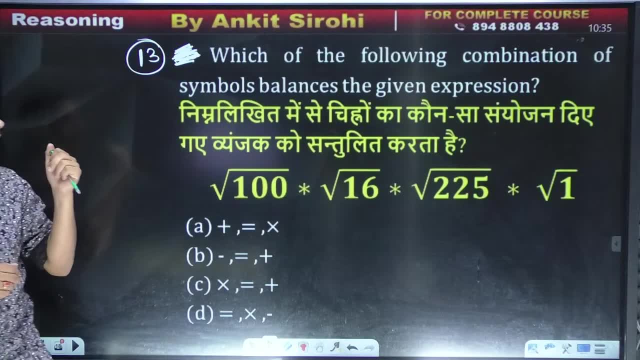 The method is good: to ask questions And let's see how much knowledge you all have about it, Dear friends. only then you can tell us about it. Brother, how much knowledge you do not have, it will all depend on your understanding. 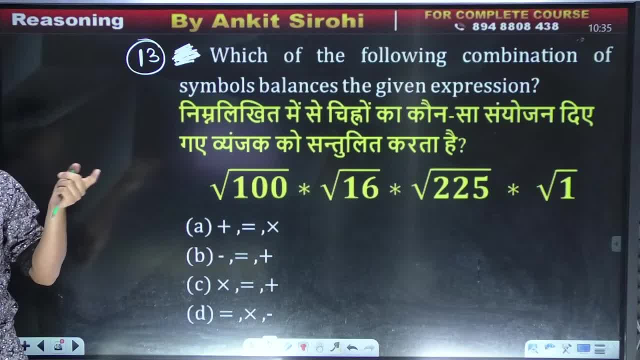 Brother? what is the right answer to this? What is going to happen in the end? What do you all have to use in the place of these stars so that it can be balanced? my dear friends, I have to tell you all quickly. 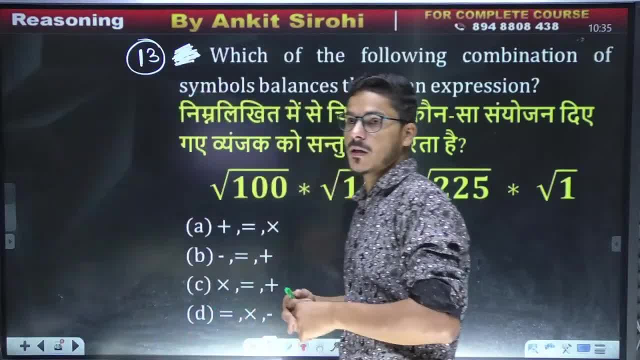 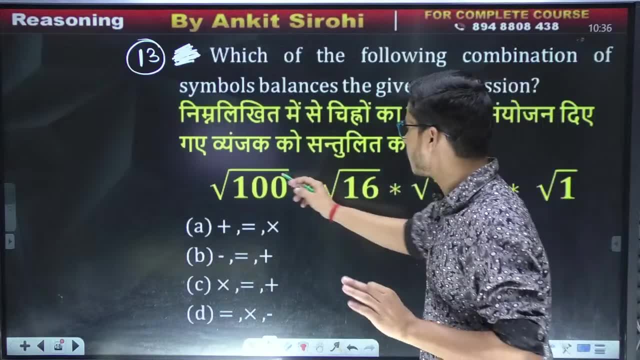 See, first of all, we will see, Okay, see, First of all, we will go to the philosophy of equal and equal. See one thing: all of you are my friends If I write this like this. see quickly, If I write this as 10, you will understand what I mean. 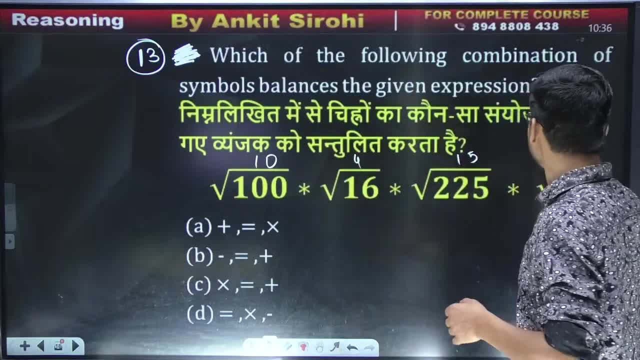 If I write this as 4,, if I write this as 15, and if I write this as 1,, there will be a problem. Say it: If you keep doing it quickly here, then 10 and 4, 14 are equal. 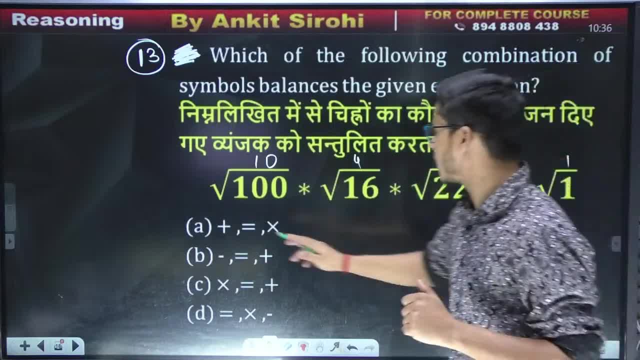 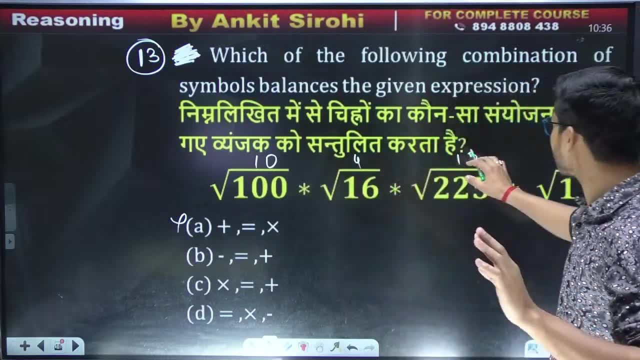 And if there is a number of multiples, then 15 minus 15, 14 and 15 cannot be equal. It cannot be. It is over Second minus equal and plus. To say: if 4 out of 10 is equal to 6,, then say 15 and 1 is 16, then 6 is equal to 16, it cannot be. 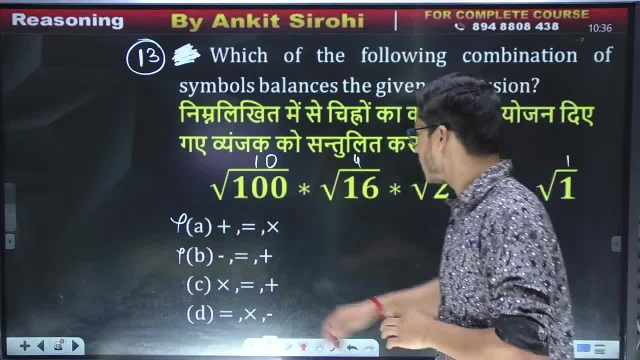 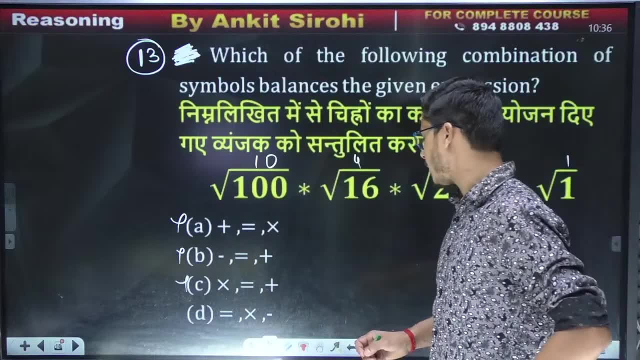 In this way. try to do it quickly. Option D: Multiples Brother 10 to the power of 40 has become multiples and equal to plus has become. then also, it will not come What will be right. See Here, my dear friends, equal, equal and minus. 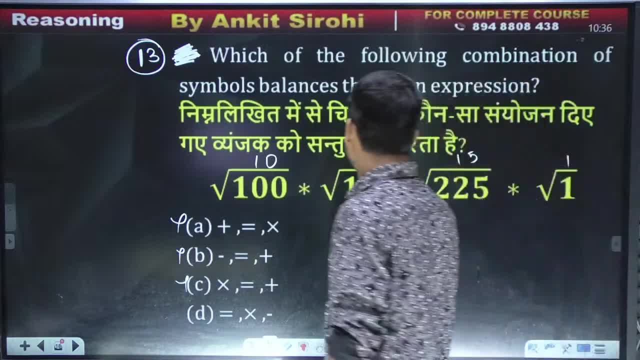 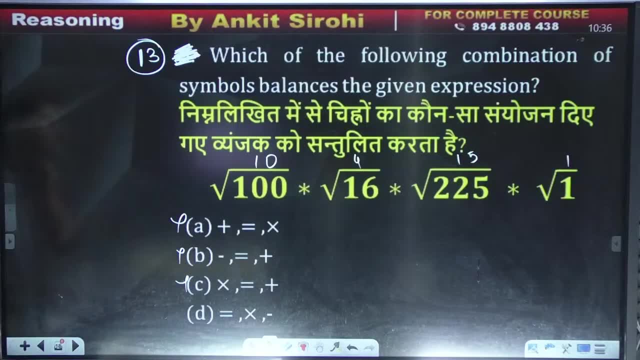 Meaning That equal, equal and minus, Equal, equal and minus. Hey brother, equal, equal and minus Here. if I make it equal Here, if I make it equal, my dear friends, then what will be the right answer? 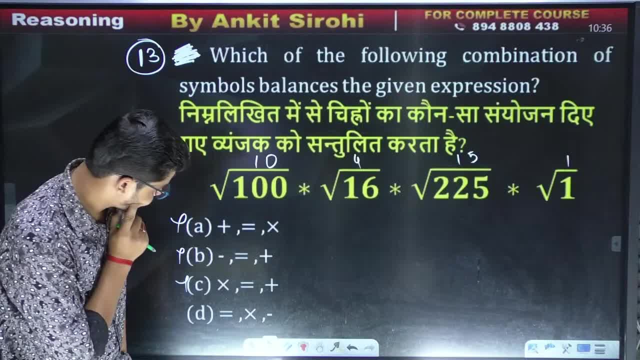 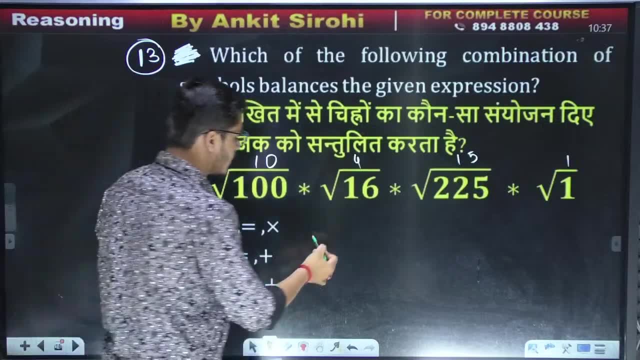 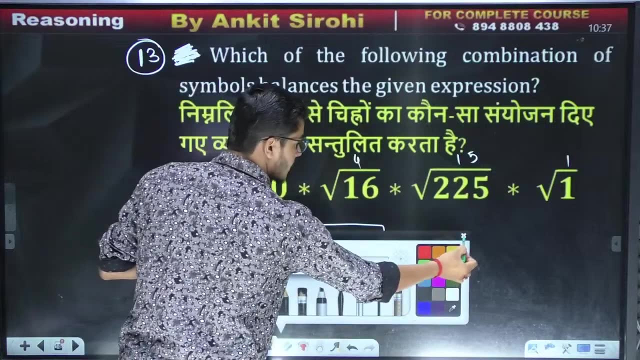 What will be the right answer Here? write an option: Plus, equal and minus. This option will be yours. Remember Here we can see that our answer is going to come from this: What is done here, my dear friends? 10.. 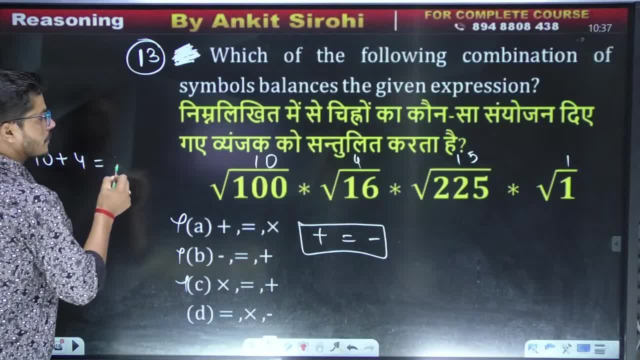 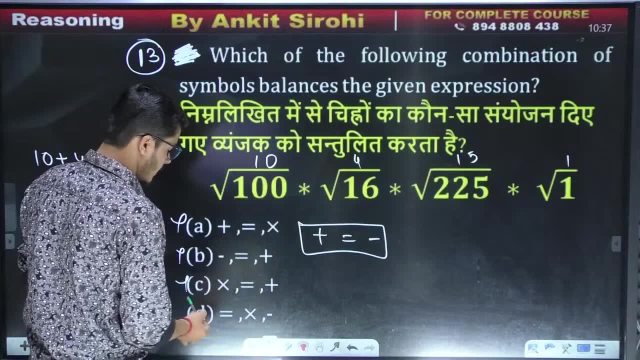 Okay Now, plus 4, equal 15,, minus 14, equal 14.. If it is given, then say a new one which was not given in this. My friends, this is also not there. 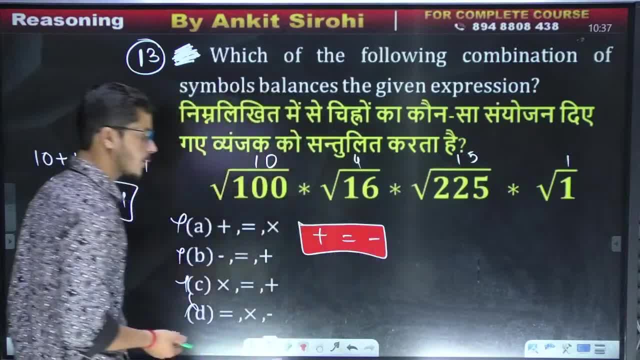 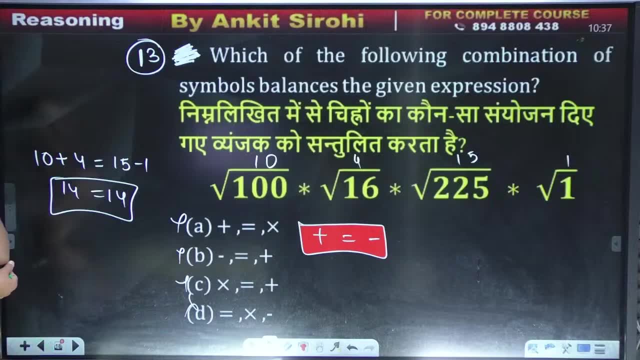 So option number, you can get it in the form of option number E. Here, my dear friends, which will be D, will not be my dear friends. So it will be plus, equal and minus. It will be plus equal, minus. 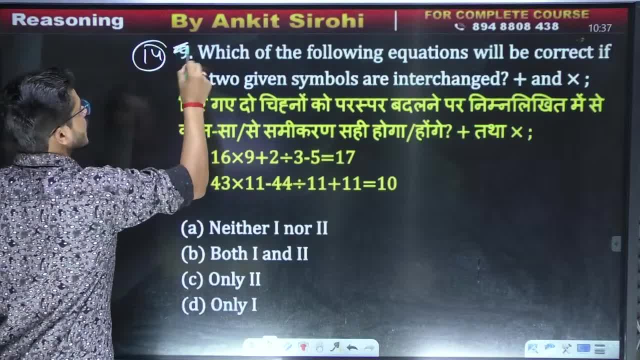 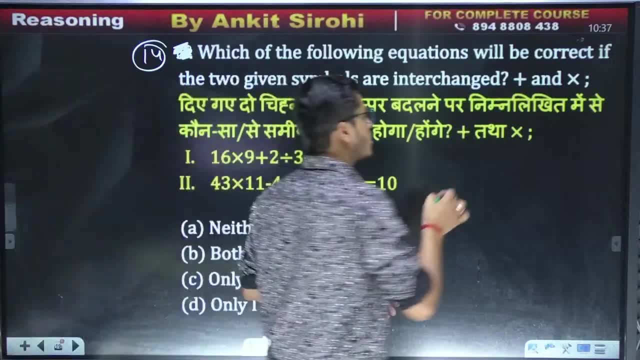 Let's go In the meantime. 14 number's percentage is in front of you all. What is said in this Once? look carefully at everyone's percentage. It says that the given signs, my dear friends, now you have to understand what I am saying to you, plus and minus. 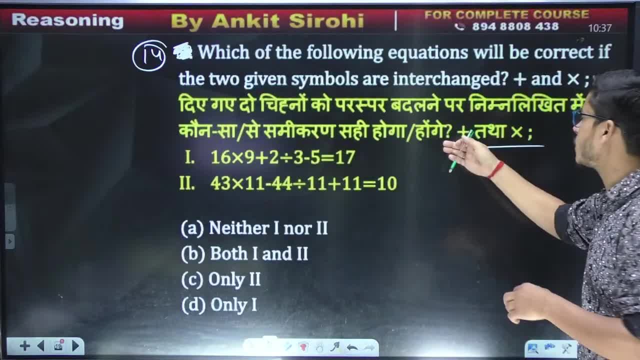 What does it mean to say? Look at both the semigrants in the form of 100,, my dear friends, And tell me that which of the two signs given will be correct, out of the two signs that have been given to change the percentage? 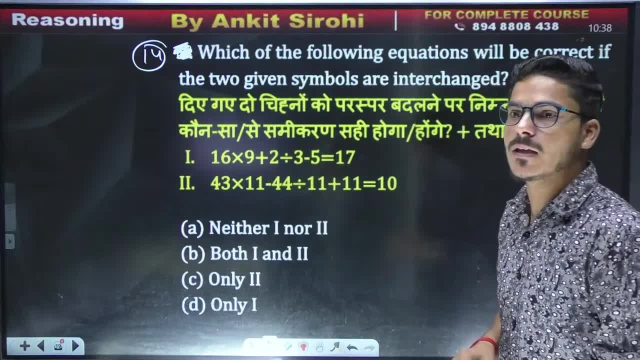 So first of all, we have to check. my dear friends, The answer has not been given. Okay, no problem, Come on, You will see here there is a mistake, My dear friends, you also know it. First check the first semigrant. 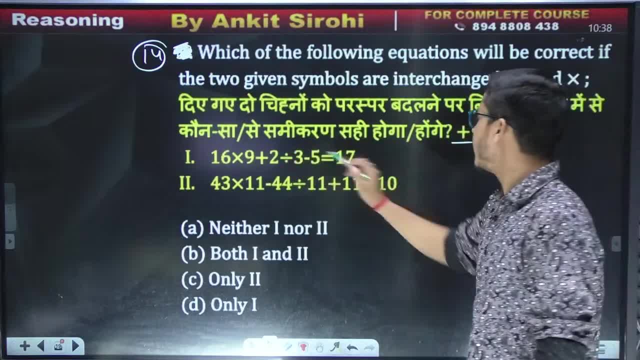 Because, simply, we have to do the change in plus and minus. only If we write the first semigrant, you will see that it is 16.. My dear friends, do you understand what I am saying? It is 16. Plus 9 in the place of minus. 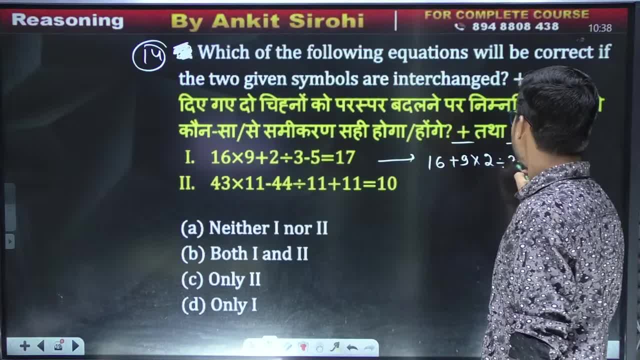 Plus 2 in the place of minus. Divide, my dear friends, 3 minus 5.. Will it be equal to 17?? So, first of all, we have to solve it once. To solve it, my dear friends, what we have to do is divide it. 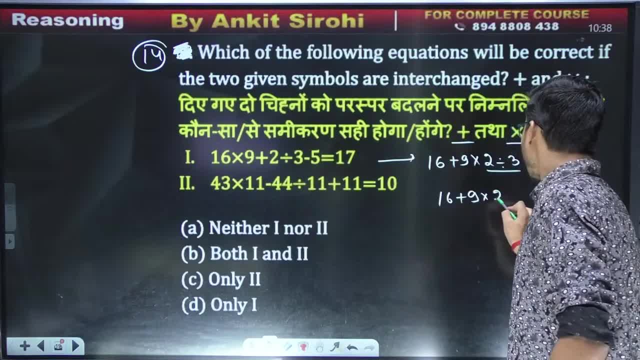 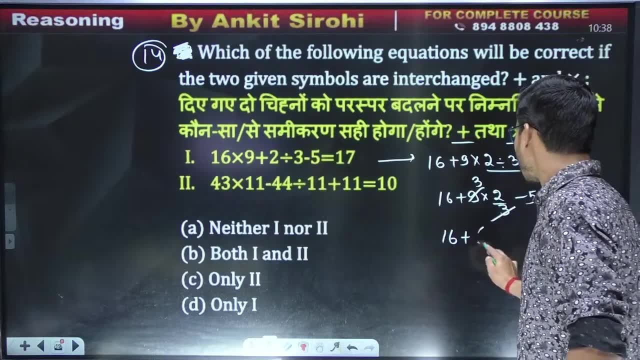 So, my dear friends, 16 plus 9 times 2, times 3 minus 5.. It was 3 times 9.. Now how much? First of all, my dear friends, 16 plus Not 3 times 2,, my dear friends, 6 minus 5.. 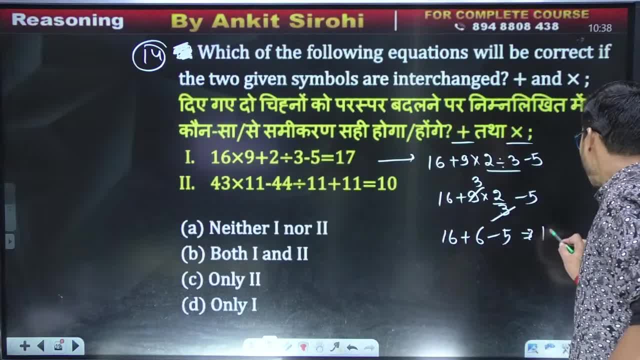 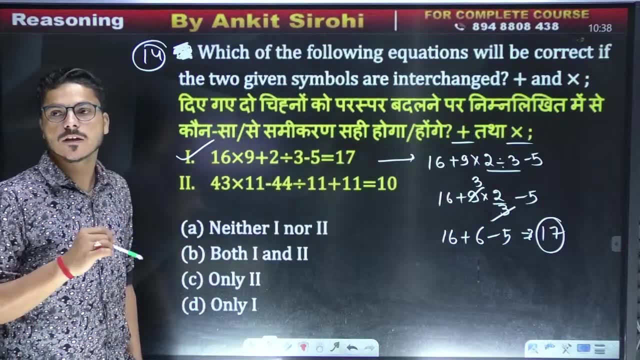 16 and 6 is 22.. 5 out of 22 is equal to 17.. So this means that our semigrant has been solved by changing both the signs. So it means that the semigrant is correct. We will use these two and change them. 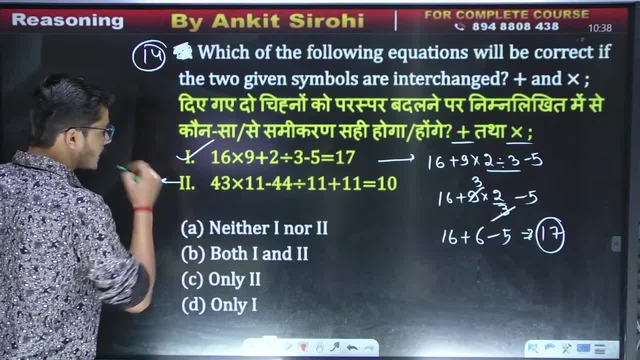 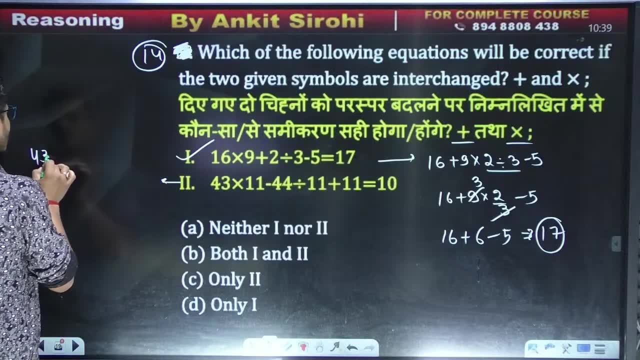 In the meantime, check the second code once. So see, we will write the second code here. What is the second 43.. What will be the place of 43 times, My dear friends? plus 43, plus 43, plus. 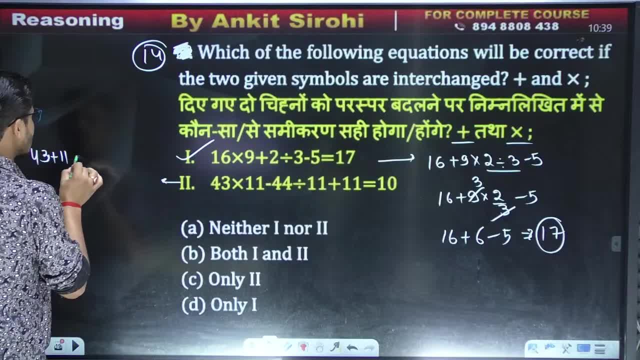 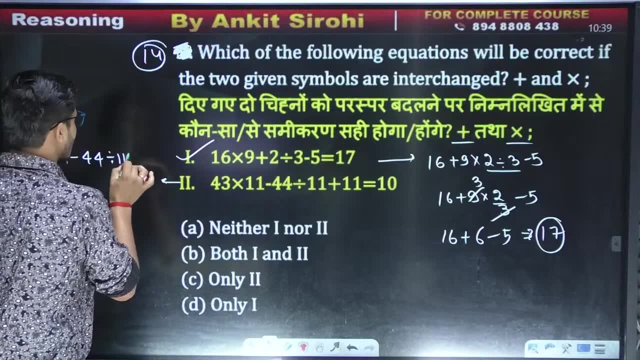 What will it be? 11.. Okay, my dear friends, Minus 44.. Minus 44. And the part, my dear friends, part 11. Part 11. The place of plus is 11.. Will our 10 come out? 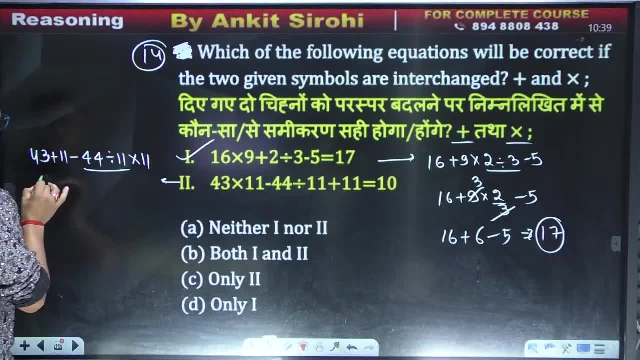 So first of all use the board mask. If we use the board mask then the first friend will see. Here will come 43 plus 11 minus 11 square 44. And the value is 4.. So first of all you have to see: 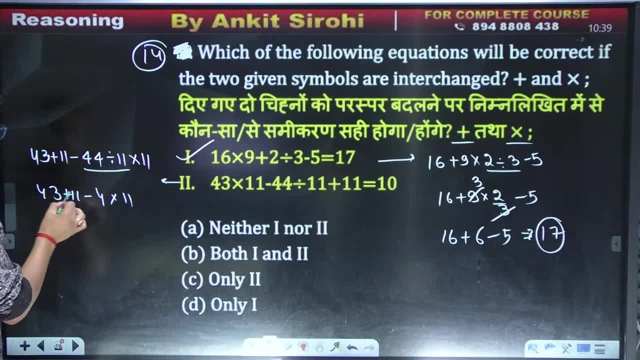 The value will be 11.. So see 43 and 11.. So how much did we get? We got 54.. How much did we get? First brother, 54.. And here, what is it? When we did 44,, we reduced it. 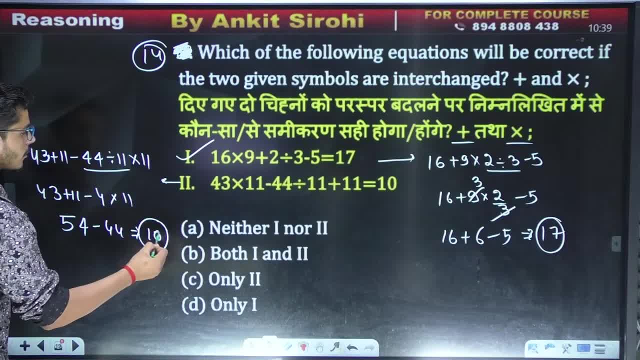 So when we went from 54 to 44, we said we have 10 left. So what does this mean? Even if we change both, the second one is also correct. So remember right, Both first and second. its correct answer will be which: 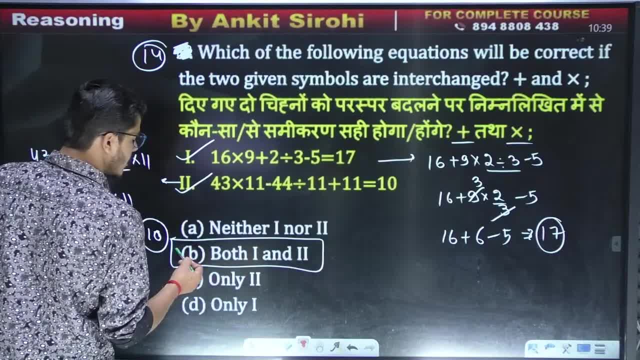 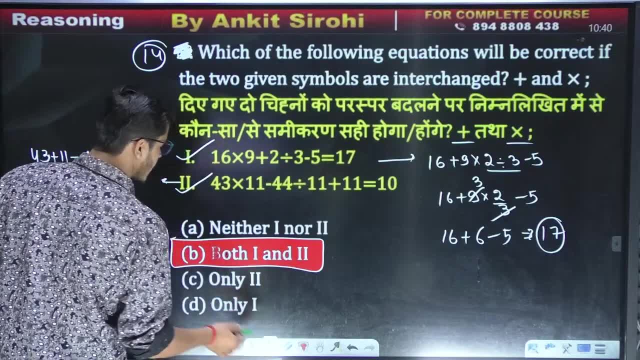 One and two. both of them sit correctly, According to which the option that was given, in which option B will be first friend, it will be the correct way to keep it here. Now you will say, dear friend, that the symbols that were given when we changed them, our two symbols, have been balanced. 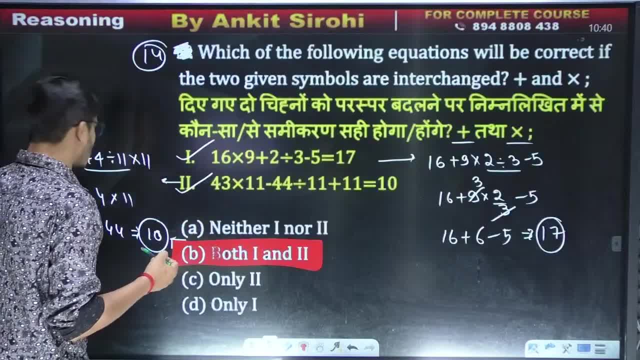 So, dear friend, why, Why don't we? dear friend, what will we do with the correct answer of this brother, Which will be the correct answer of this? Both are correct. Come on, guys. the 15th question in between is in front of you all, the question of number 15.. 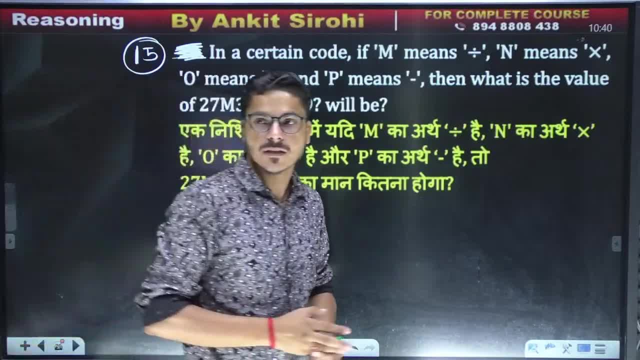 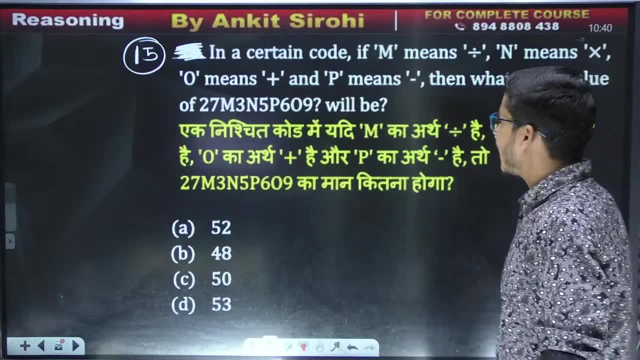 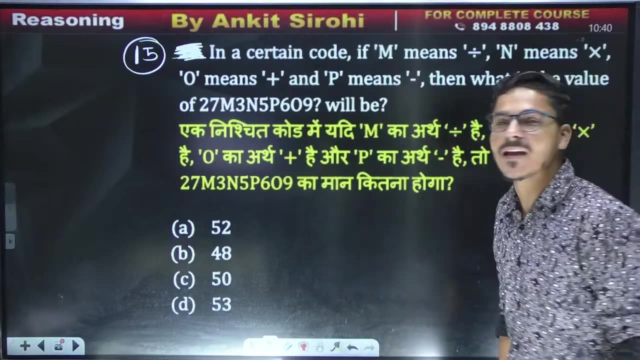 What does the question of number 15 say? Tell me quickly: 10, absolutely. Question number, dear friends, is in front of you all: 15.. Both first and second will be right, dear friends, In a definite code. if the meaning of M is a part, the meaning of N is a quantity, the meaning of O is plus and the meaning of P is minus, then, dear brother, what will be the answer to this? 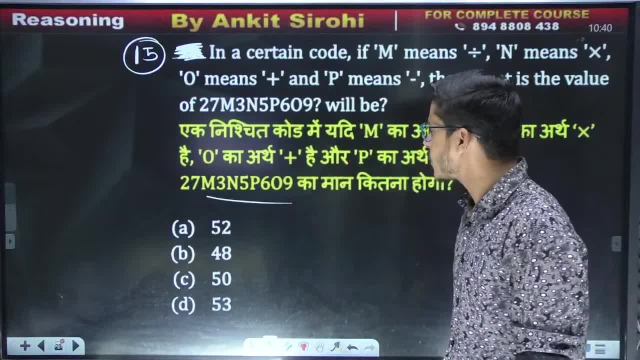 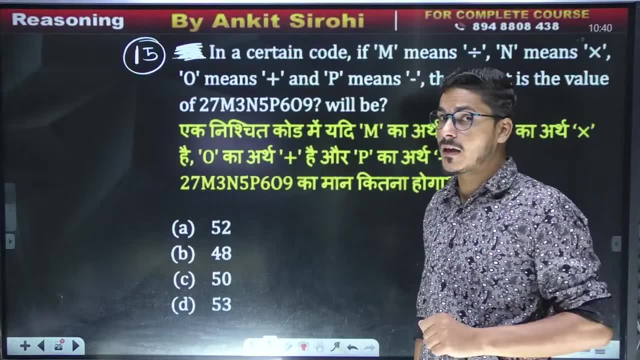 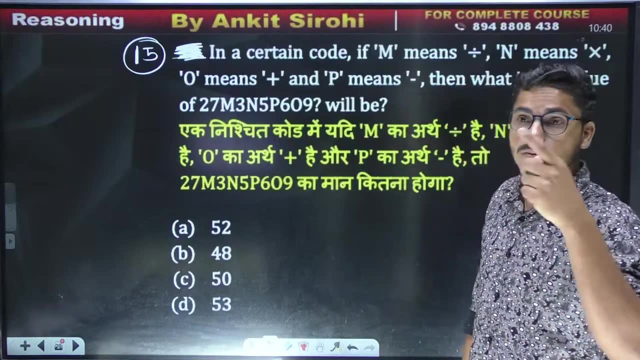 Like this, You will get it. show me If the point that the problem can be solved is saved, which is our pattern. when we say correct answer, then correct answer is chose, because So God says. Scott, You can ask him. I longer have to see. 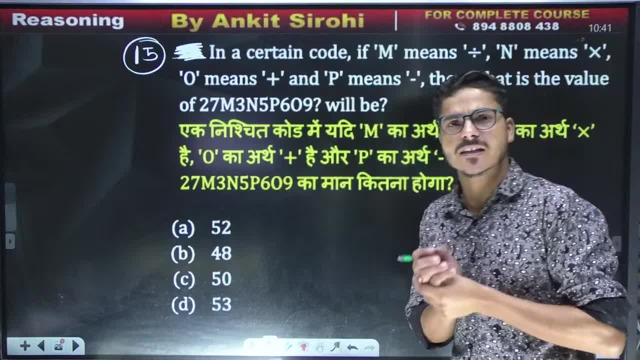 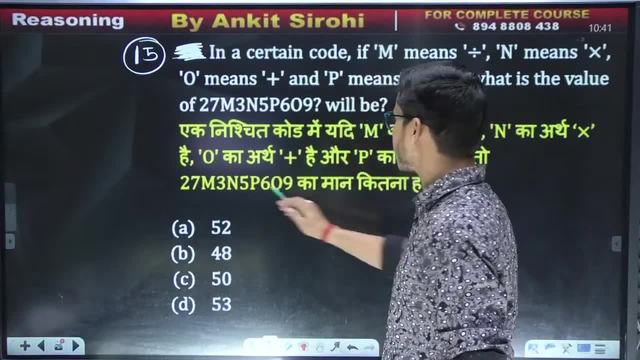 Look, the problem is obvious. If this problem was solved, then it would have been supposed to happen in the way you told. If edea was not right, It was supposed to be acceptable in the way we are told Is not What to keep on the place of m: Make all columns 27.. 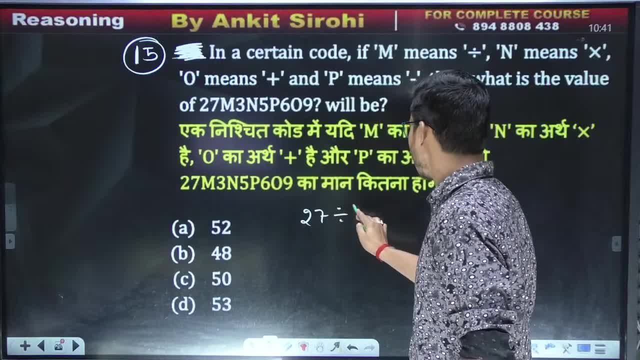 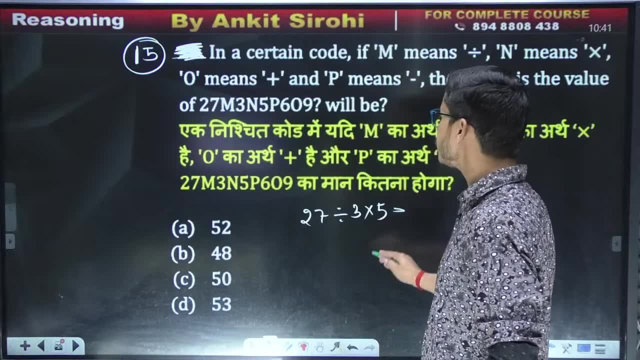 Keep on the place of m, First brother, 3.. On the place of m, we will put times. 5.. Friends, what will be the meaning of p Minus 6.? What will be the meaning of o Plus 9.. 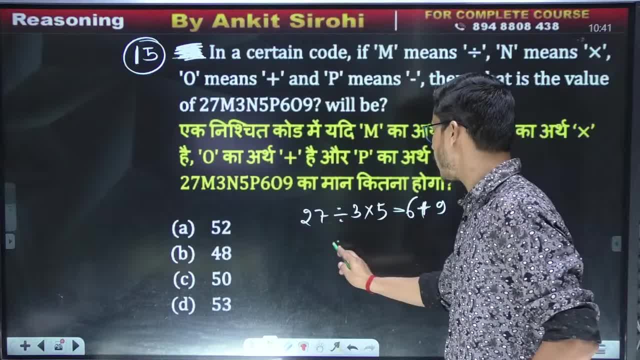 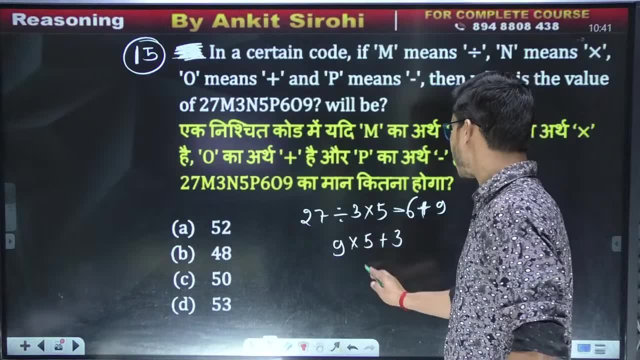 Now solve it. First of all, if we run, then you will see 9 times times 5 minus 6, and this will be the 3 of plus. So 9 times 5 is 45.. 3 equals to what 48.. 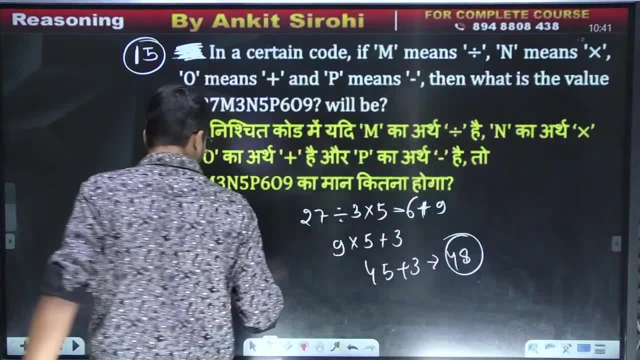 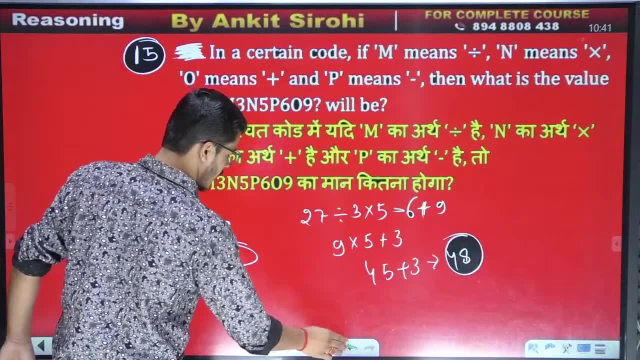 What is 48?, My dear friends? how much will it be? 48 is the correct answer, See: 48 is the correct answer. My dear friends, our math is good, but we do the calculation a little fast. Dear friends, we do the calculation a little fast. 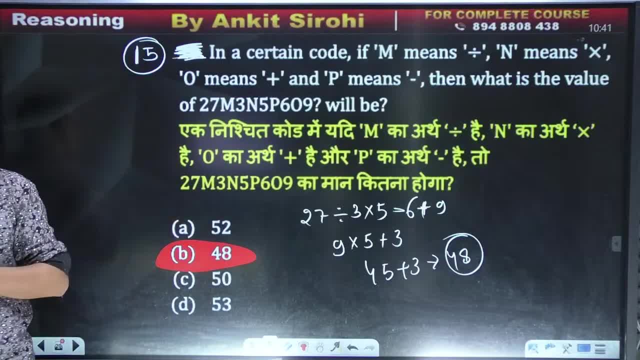 48 will be the correct answer: 48,, 48,, 48.. Excellent, my dear friends. 9 times 5 is 45 and 3, my dear friends will be 48.. Very good brother, How much is 48?? 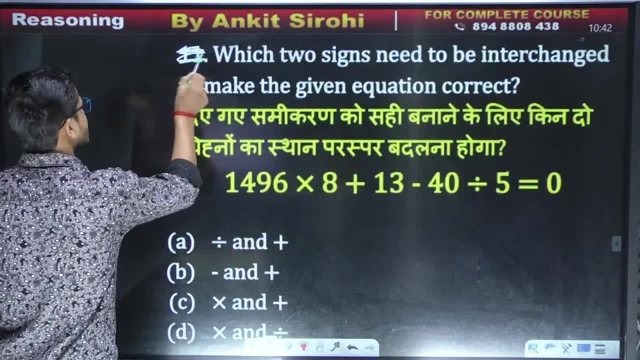 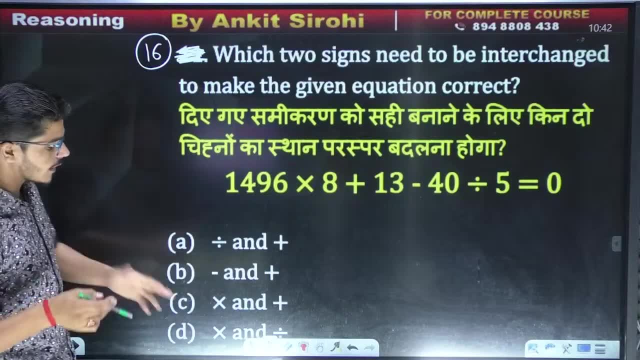 48. Let's go in between. in front of us. What is the question of number, Brother? we have come in front of us. Which person is 16?? We will give the answer of 16.. What will be the correct answer of this? 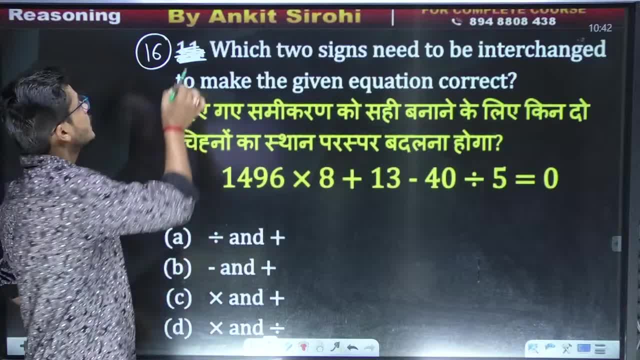 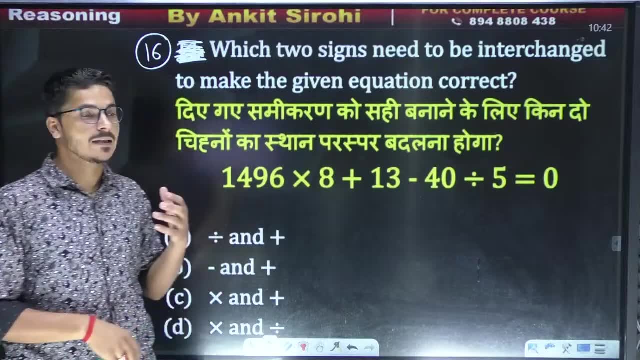 Means what to do in the question. Nothing to do, my dear friends. What to do in the question? Here you have been asked which two signs need to be interchange to make the given equation correct. That is, to make the given equation correct. 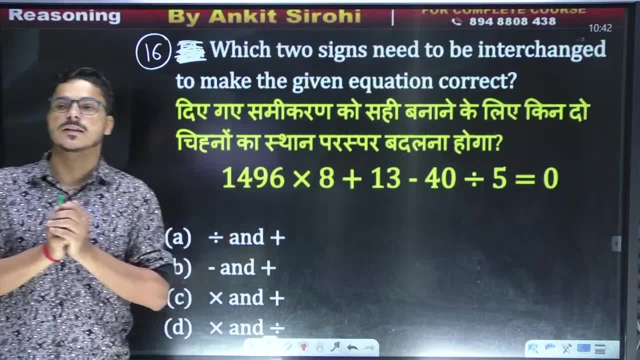 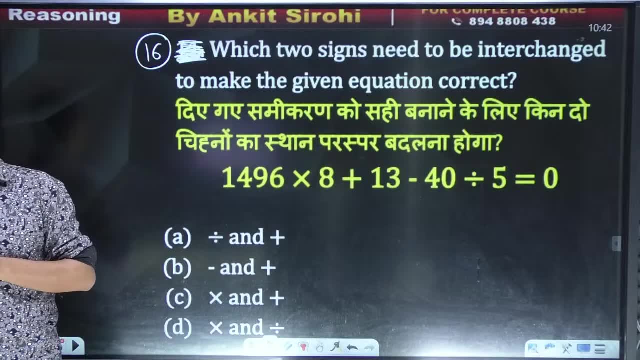 after changing the place of the two signs. here the equation can be balanced. This has to be told. It can be corrected. You have to give the correct answer. So let's see who gives the correct answer. Who, my dear friend? 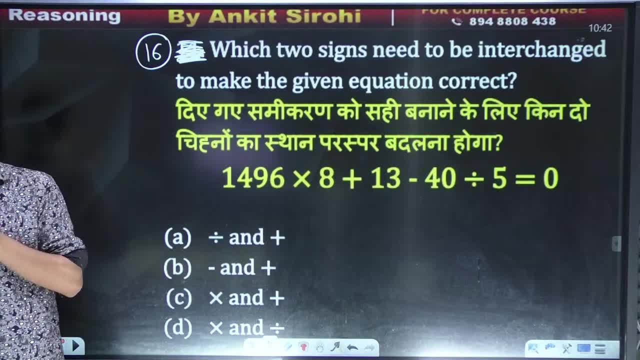 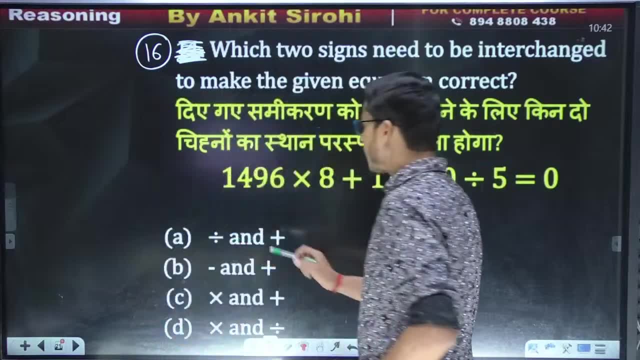 is giving the correct answer first. You will see that the correct answer will be with me. You will see that which signs will be used to change. First of all, I will change the part and the plus, The part and the plus. Think a little. 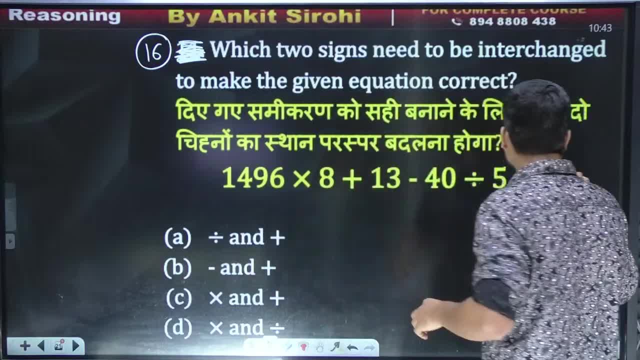 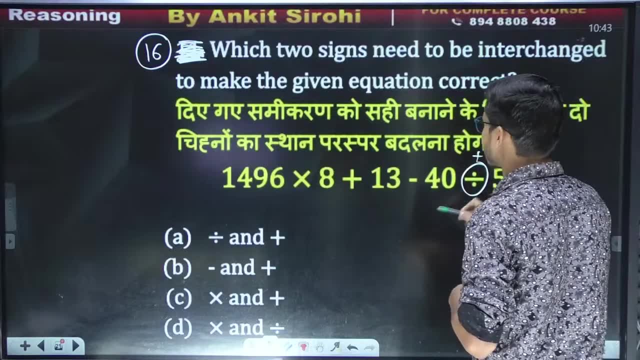 It will depend on your thinking that if you do not change the value, then how will the zero come? You have to change the two signs. If you change the part and the plus, you will see that the part means that you have done the plus here. 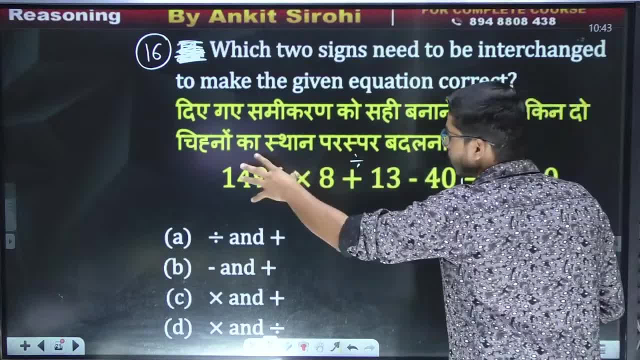 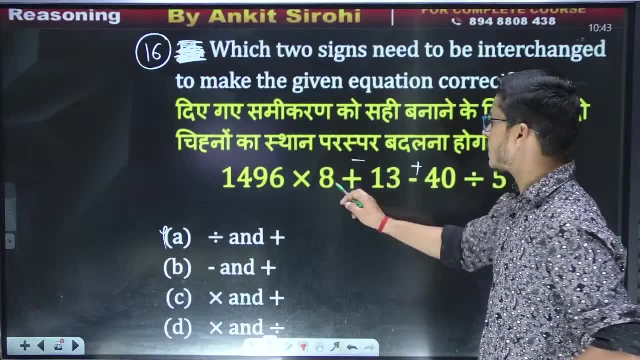 and do the part instead of the plus. Okay, tell me one thing: If you have given the part of 13 in 8, and then you will do the number, then you will not get the number zero. You are saying that you are showing. 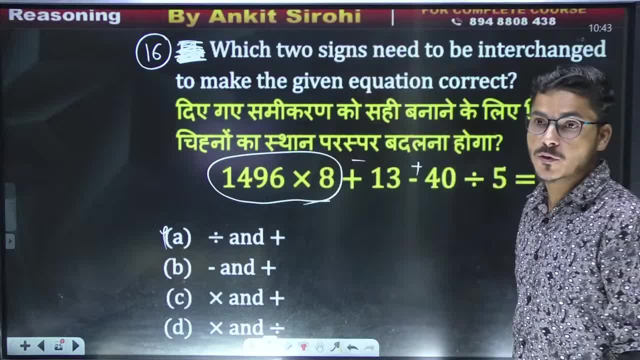 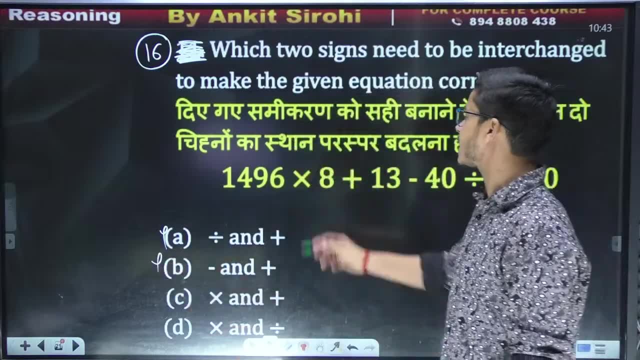 a bigger mistake. Okay, do minus and plus Here, minus here plus First of all, when its value will be, then you can change the part and the plus. You can change the part and the plus If you think a little. 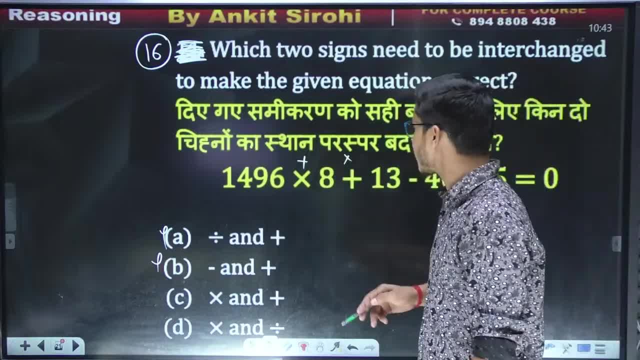 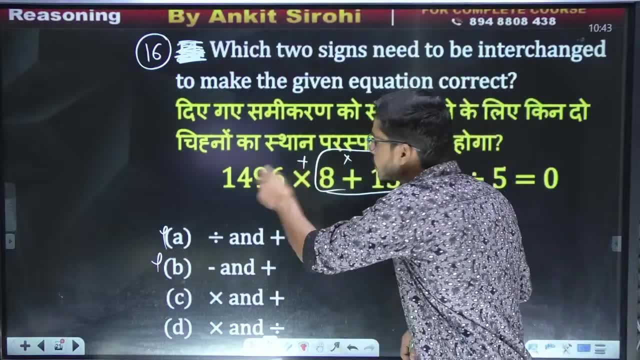 then you will say that this will not happen, and this will also not happen. Why? I have to understand this first. First of all, if I do the number here, then how much is 13 and 8? 104.. Now I have to add this in: 104.. 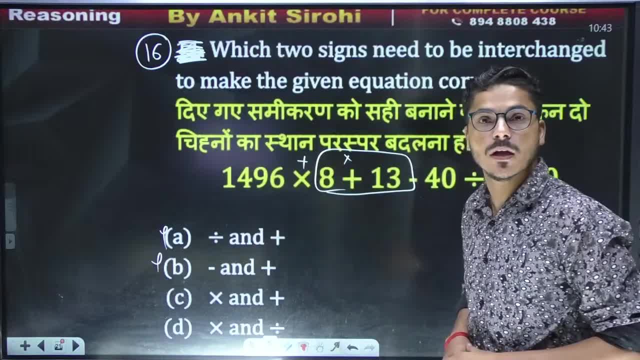 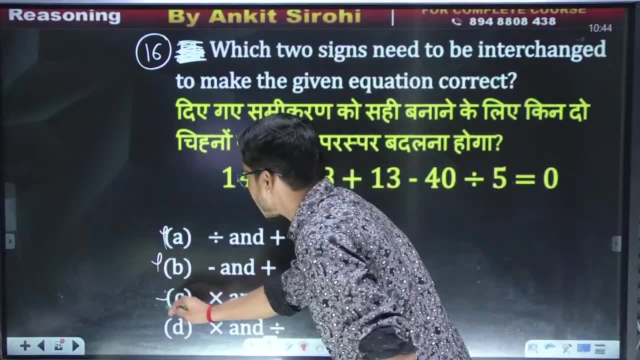 How much is it? So how much is it? It will be 1600.. Now, whatever you do, you have to listen. Now the last one is left. At the end we come to the point where you have to do the number. 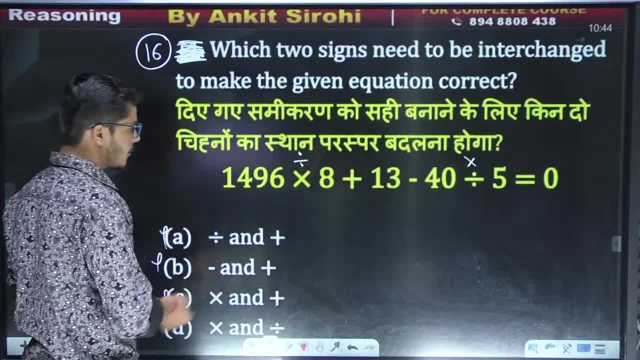 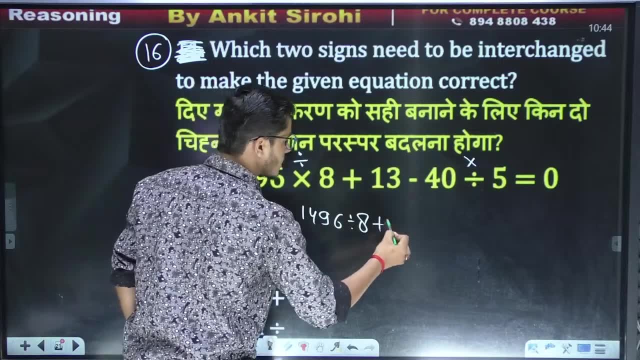 That is, you have to do the number here and then you have to do the number at the place of the number. Will it come to zero? Let's see Now what I will do here. a new way will be made that in 1496,. 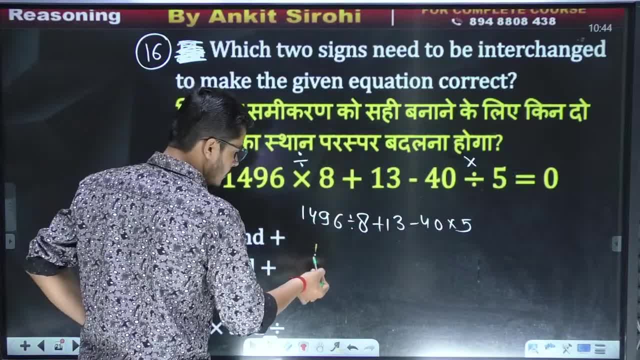 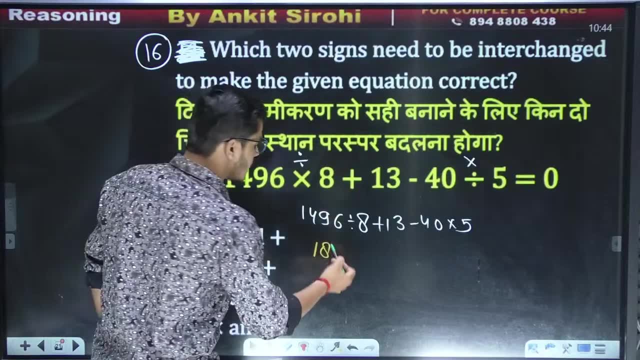 I have given the number of 8.. And, dear brothers, I have added 13 and minus 40 and multiply it by 5.. So the board master says that you all will see the answer very quickly, Dear brothers, plus 13, minus. 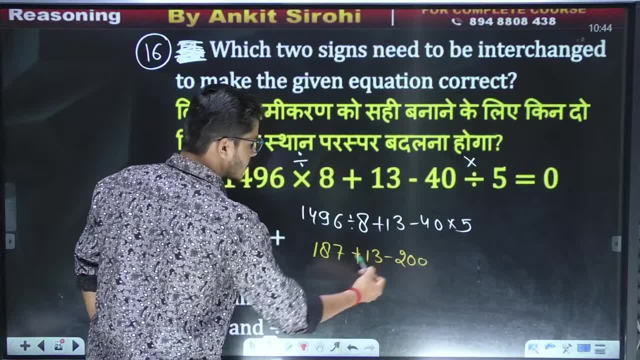 40 plus 5,, how much is it 200.. Okay, one thing was there: 187 plus 13,, how much is it 200.. And dear brothers who will have 200 minus 200, equal to You, all know that it is 0.. 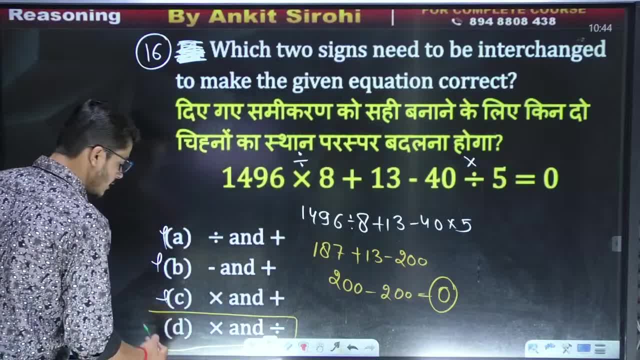 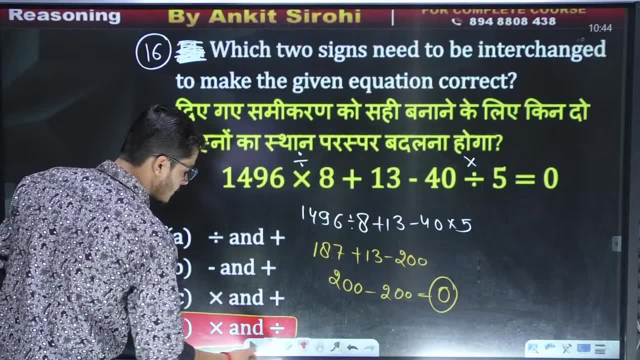 So see, if 0 is obtained, then only 0 had to be obtained. For what reason The two signs that came on option number D after changing them on the board? dear friends, we found that the answer that will be given here. 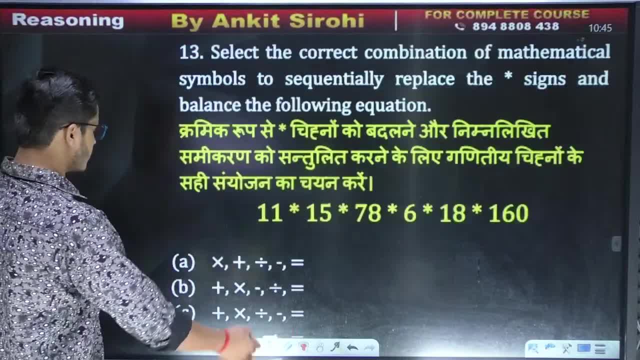 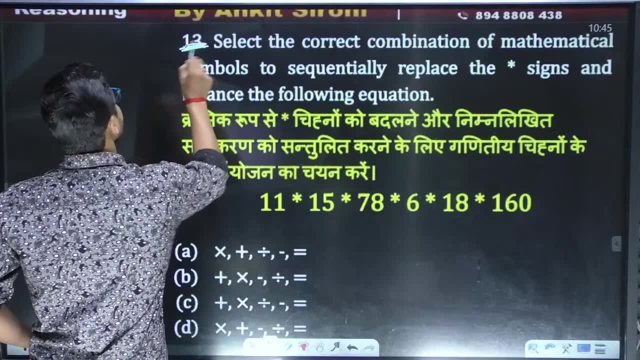 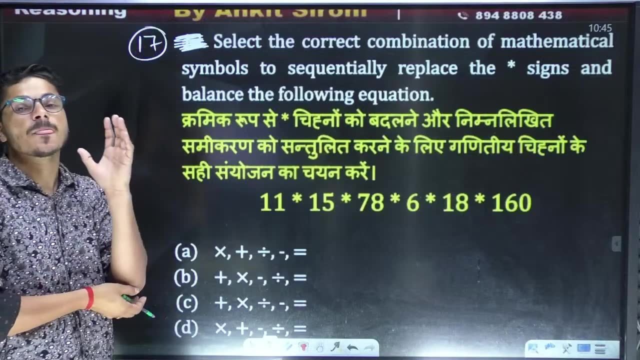 will be option D. Let's move on to option D. On which question? On question number 17.. On which question? On question number 17,. remember, On question number 17,. dear brothers, question number 17,. tell us what will be the correct answer. 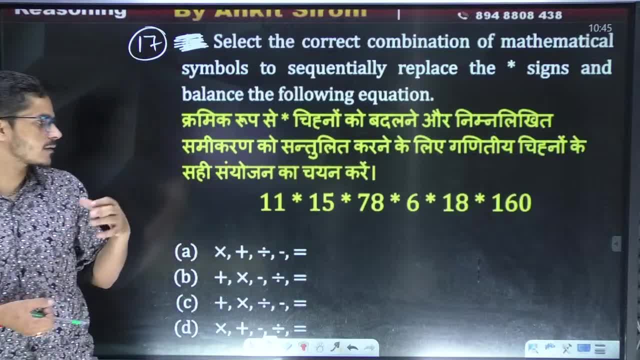 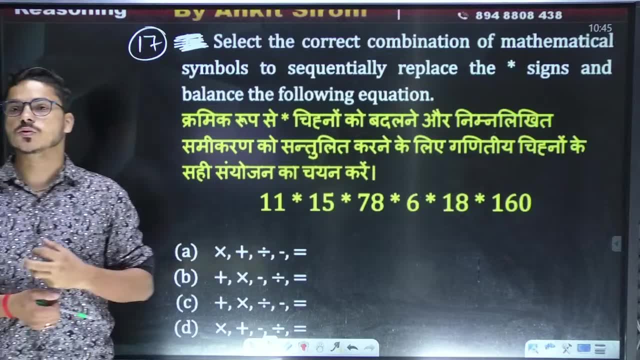 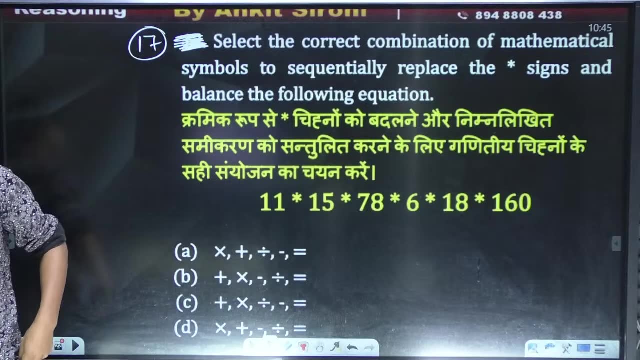 Here, instead of these stars, which one? By using the signs, we can balance the symmetry here. Here I have to tell you all which one to balance, which option will be the best for us? dear friends, What is the answer of 17,? dear friends, 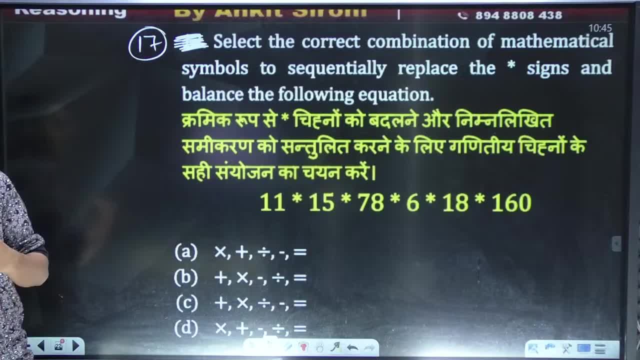 Here in front of you all, there is a wonderful line written: Dear brothers 11, star 15,, star 78,, star 6, star 18,, star 160, means what will be used here so that we get the correct answer. 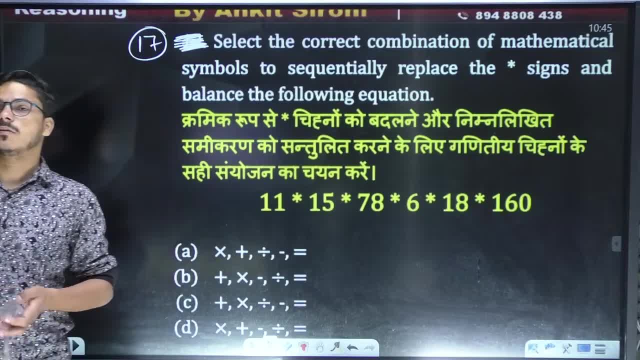 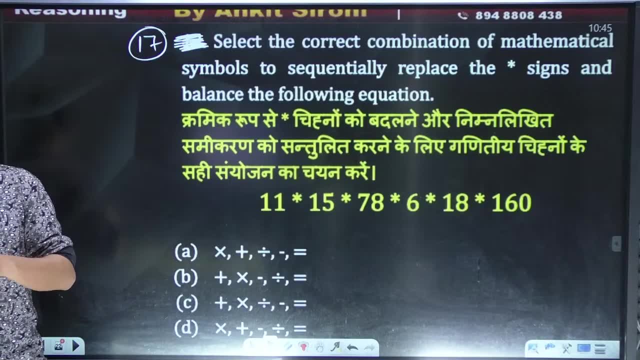 Right, Come on, tell us quickly, Let's see who will give the answer first. Yes, give it Which one will be the correct answer. Tell us quickly, dear friends, Let's see which one will be the correct answer. Yes. 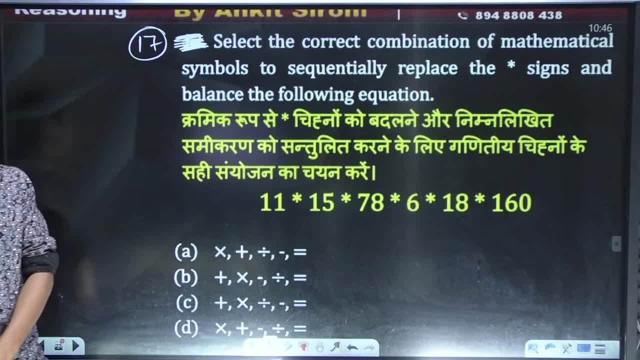 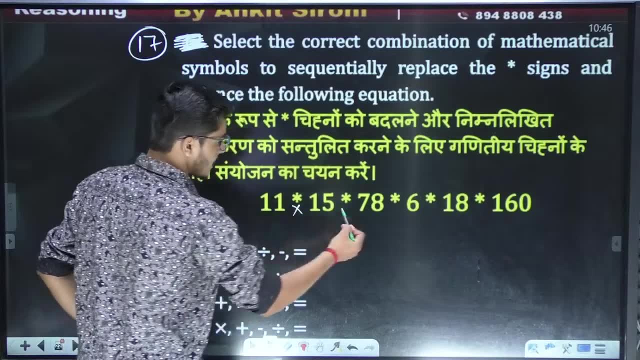 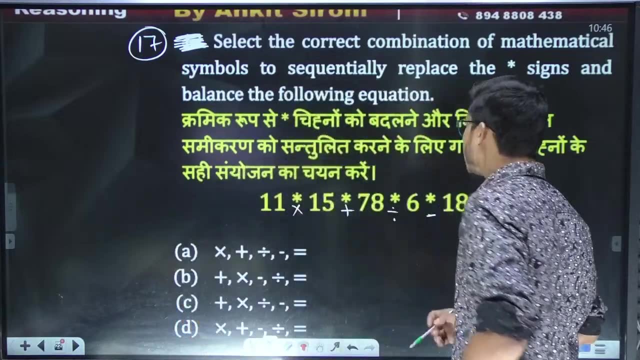 None of the friends got the answer. Brother, none of the friends got the answer. Did you see? Let's start with the first one. He said: multiply here, Okay. Then do plus, Then do minus, Then do equal, Dear friends, now we say okay. 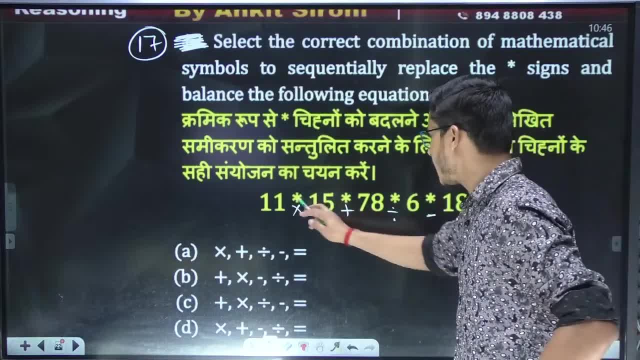 See, you have to do some calculations in your mind. If I first of all understand my thing, 11 times 15 times 165.. Here I am solving it as it is. It will come because it is coming in the middle. 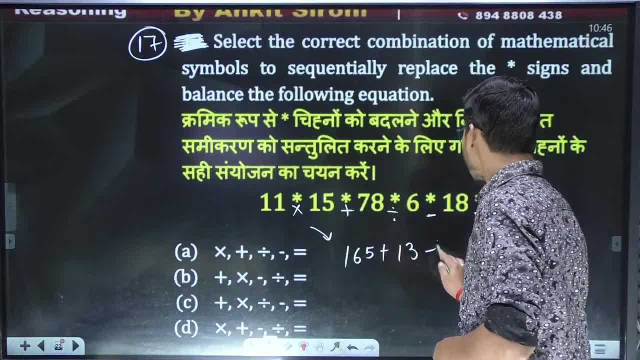 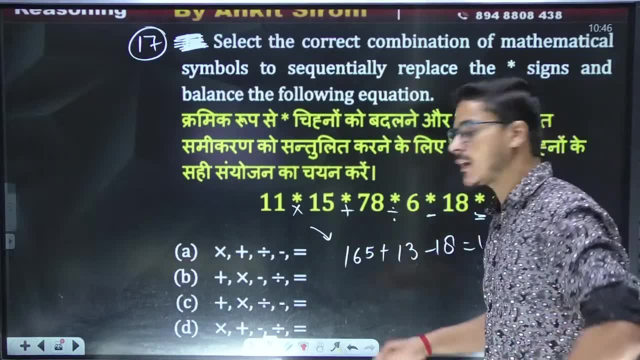 So do 165.. Now, 13 times 18, minus 18.. Will it come equal to 168 or not? Let's see Here. all of you found that, dear friends, 165 and 13 became 178.. 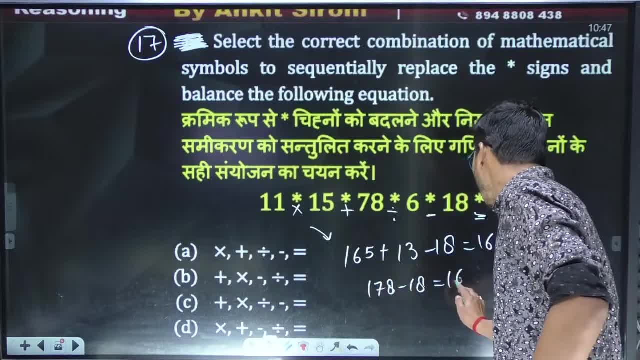 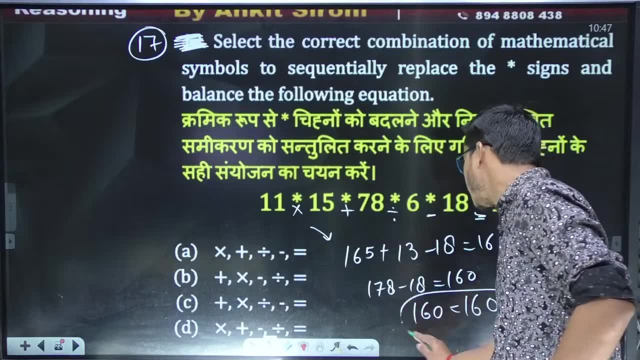 Right, dear friends, Whose 18 is equal to 168?? So you said it will go from 178 to 18.. So 160 is left. So it means 160 is equal to 160.. Through whom has it been proved? 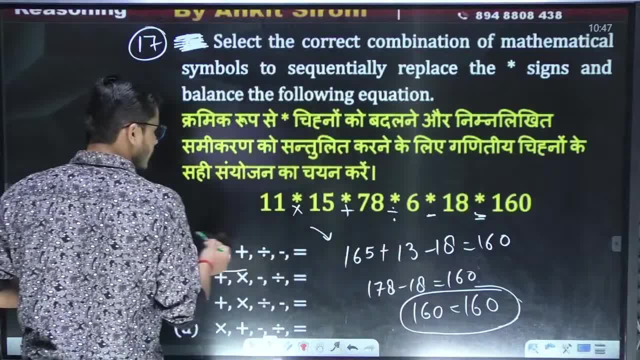 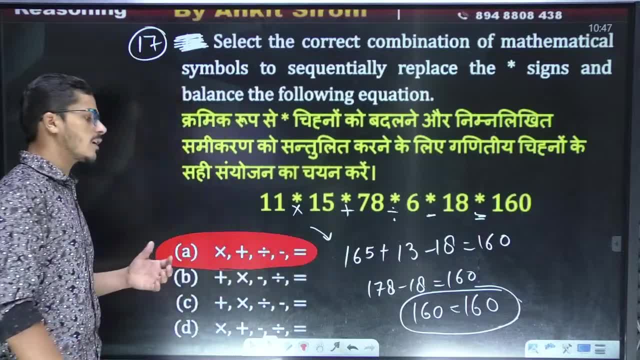 It means LHS is equal to LHS. That is the government, dear friends, who has balanced our equation. who has balanced it? through whom? Not option number A. This time we have balanced it. We have balanced it through all the signs. 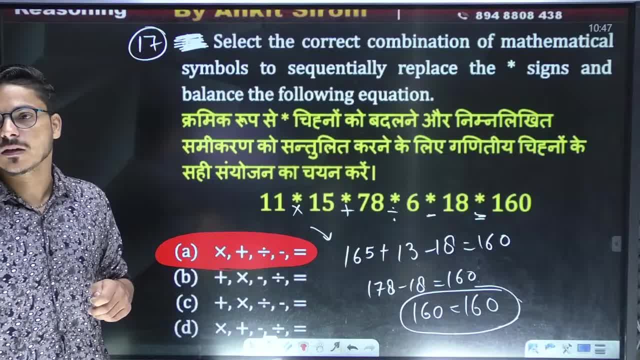 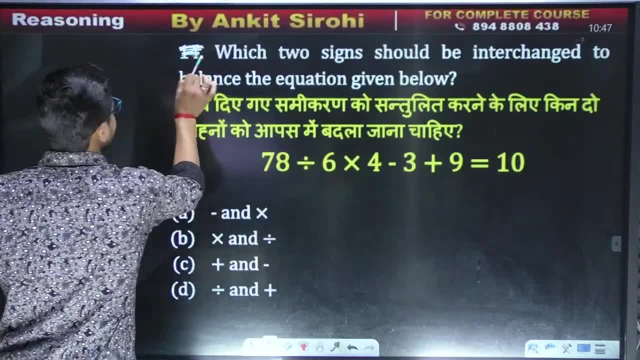 that came on option number A. Okay, dear friends Brother, the soldier girl is very good. The soldier girl also had an A. It is a very good answer. Come on, the 18th question has come in front of all of you. 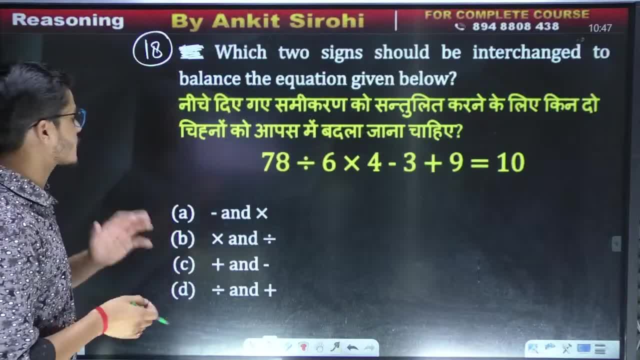 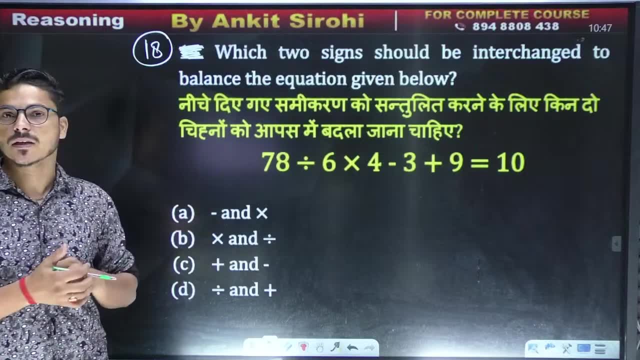 Which one? Question number 18.. What does the question number 18 of the soldier girl say? Take a look at it. Question number 18 says that it will change in each other. Who will change in each other so that our equation will be balanced? 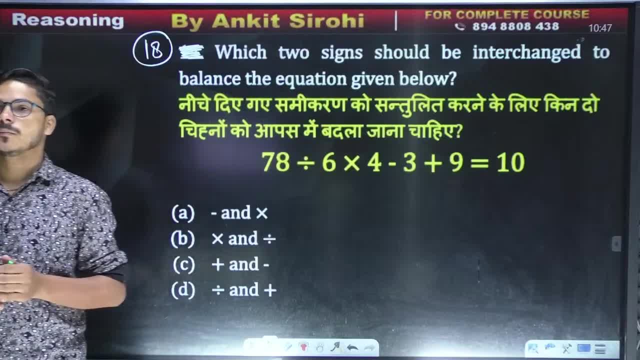 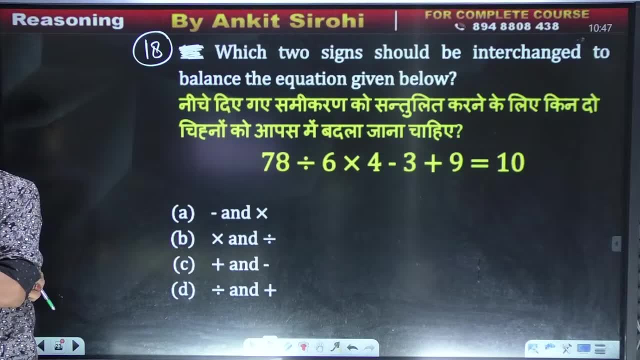 Yes, it will be absolutely 160A. Okay, It will be absolutely. A 160 is equal to 160.. Your answer is wonderful. Let's move ahead. Dear friends, all of you quickly answer what is going to happen in the 18th question. 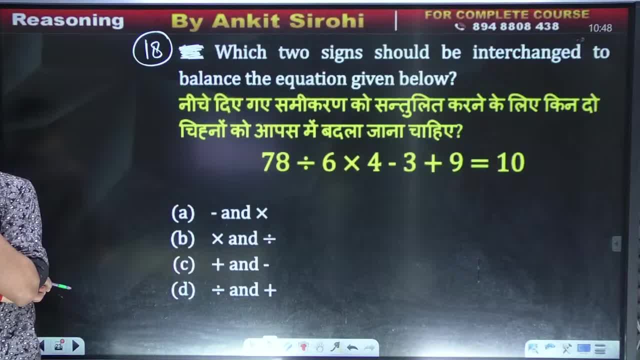 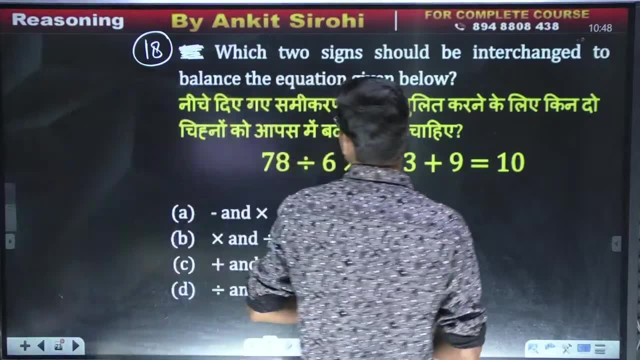 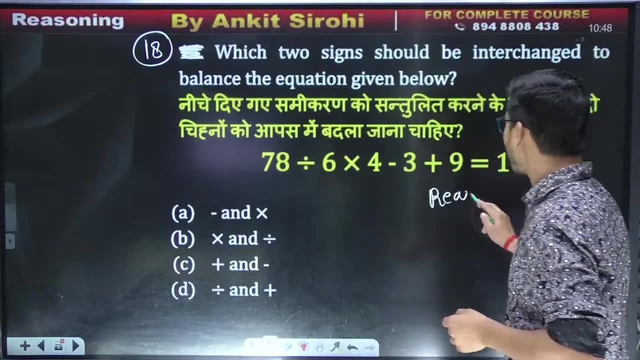 In this question which one will be changed. Which one will be changed? You all have to tell me quickly Here, all of you, dear friends, after this class, where will you get the PDF? I have already told you. I tell you that I am a soldier girl. every day, 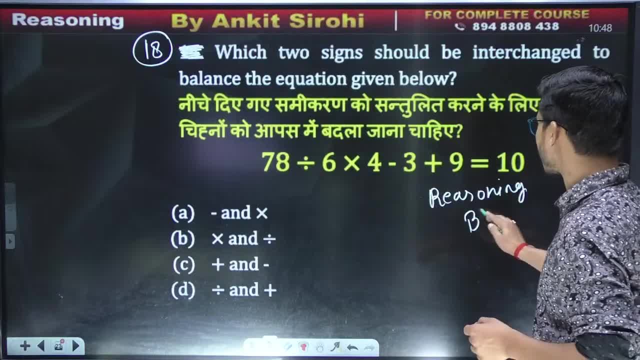 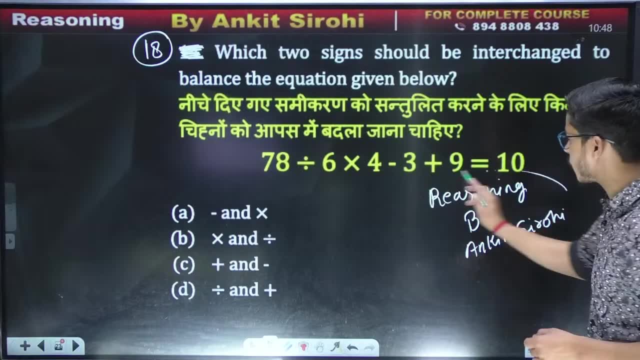 If any of my dear friends are new to the class, they will know that reasoning by M Kishore can be found on Telegram- Ankit Sarojit Telegram- And if any of you have any problem, you can ask anything in the doubt group. 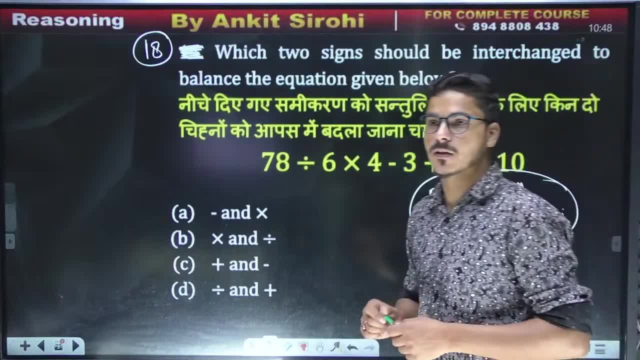 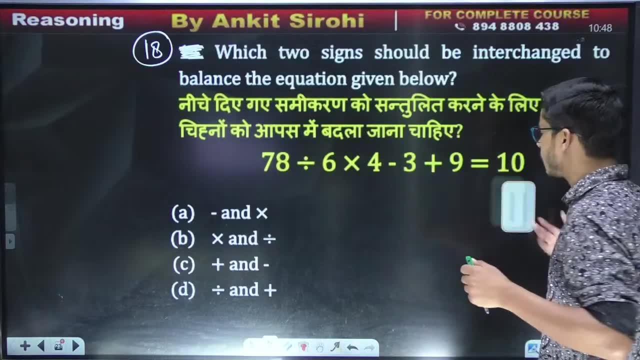 Okay, dear friends, In the end I force them to stop. Why do I stop them? Because in your P you start doing a lot of work, Dear friends. then I don't know what you start doing If you change minus and equal. 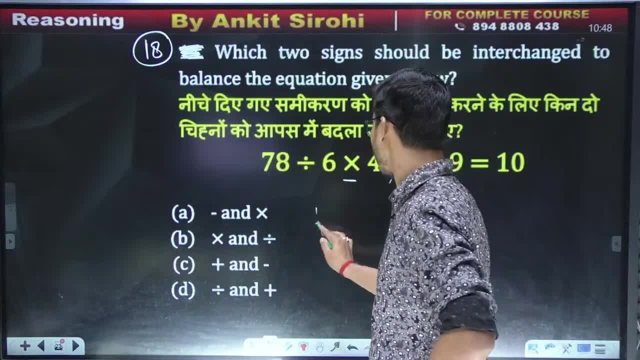 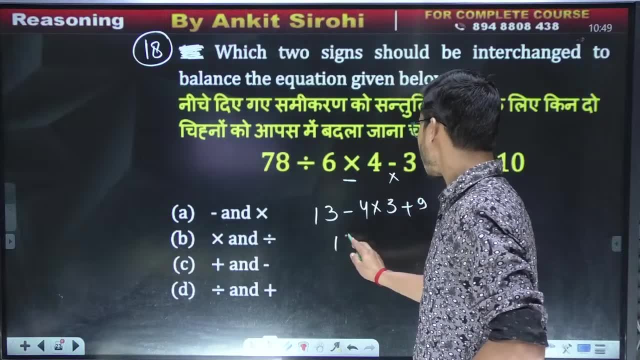 here is minus and here is equal. Let's use it In 78,. 6 ran away and said 13.. Okay, dear friends, Minus 4.. So 9.. Will we get 10?? Dear friends, 3 minus 4 is 12.. 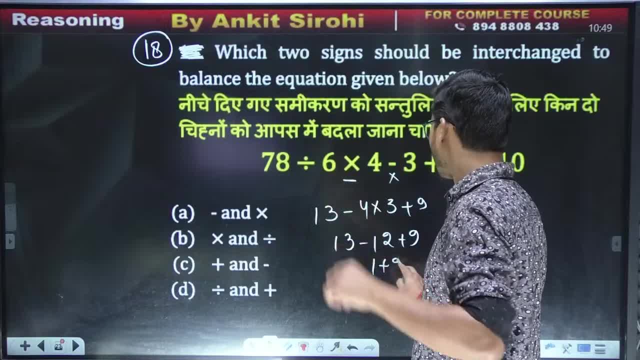 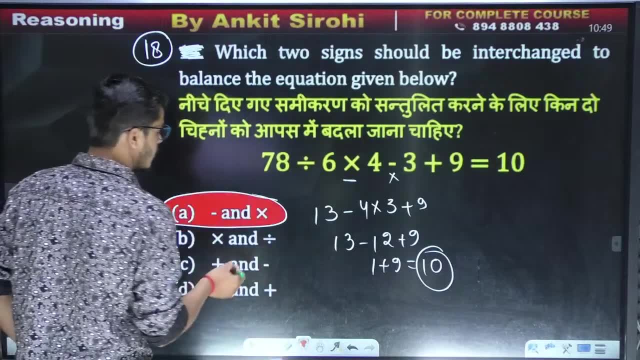 Plus 9.. So you said that out of 13,, 12 ran away. Tell me: 1 is left Plus 9 equals 10.. So this is our correct answer: 10 equals 10.. Option number A is the correct answer. 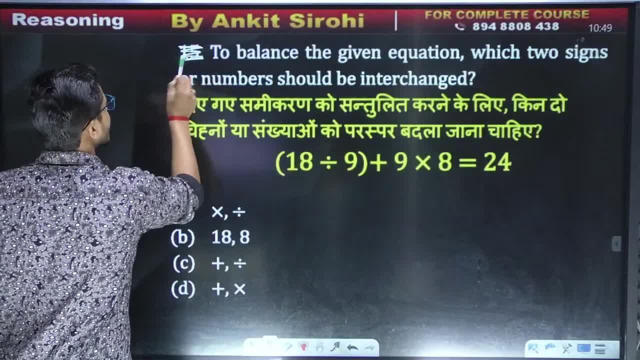 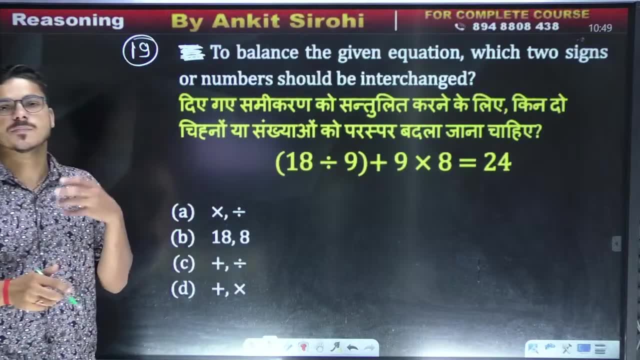 Let's go in between. We have one more question in front of us, Question number 19.. Let's see what is the answer to question number 19.. In this question you have to tell everyone that who should be changed to each other. 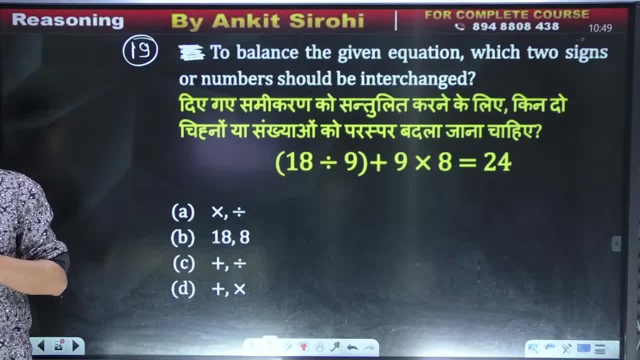 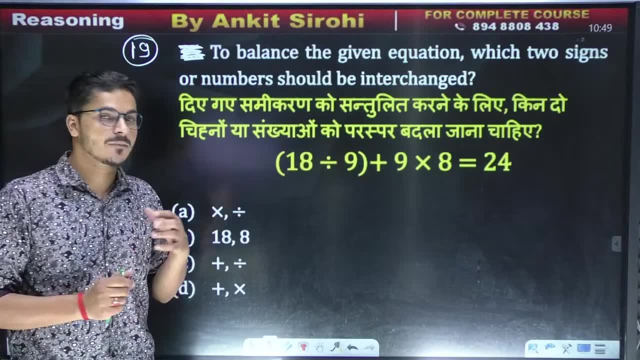 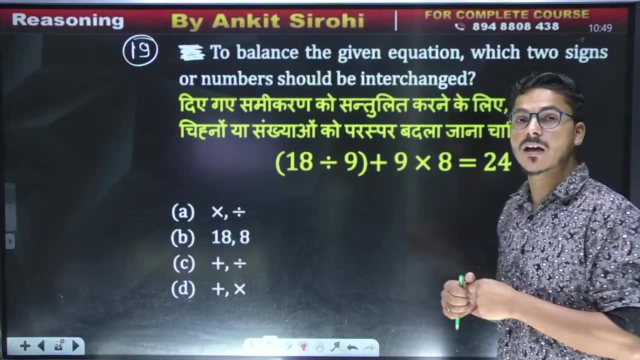 so that the balance can be made. To do balance calculation, 18 is the correct answer. Let's go in between. Now, in front of everyone, the next question has come To do balance: who should we use? Who should we change? 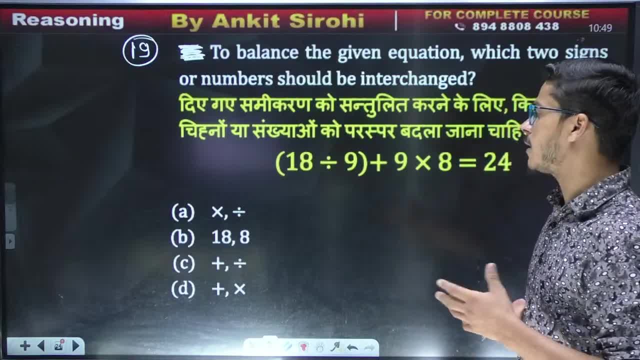 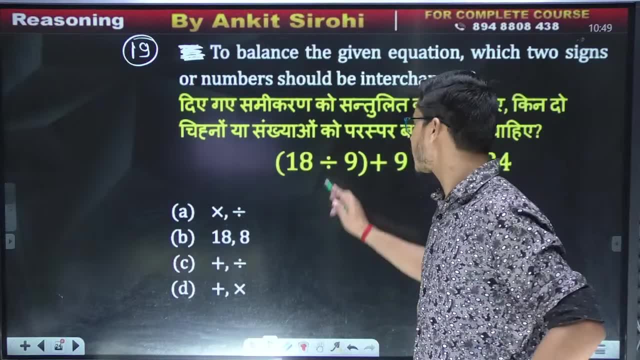 Who should we change each other? Do my friends have to do the numbers or the numbers? Look my first. friends, if you all think that, first, the value and the part means the place of the part is the value and the place of the part is the part. 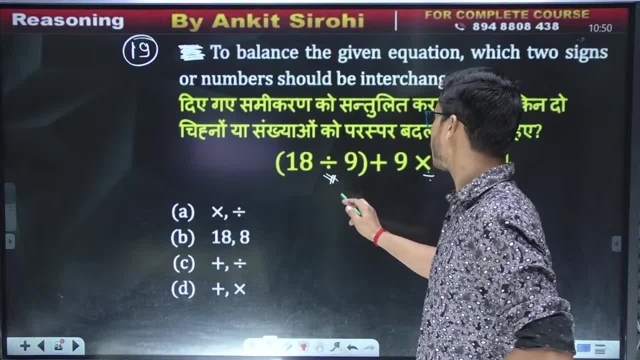 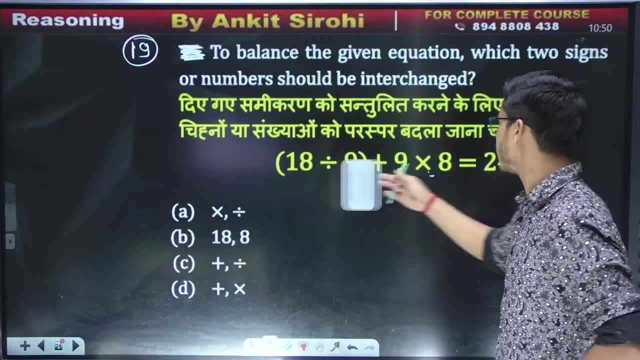 So you all know that 18 is 72.. No, not 172.. 162.. Plus 9 divided by 8. So we will not get 24.. No, So the first one is wrong If you change 18 and 8,. 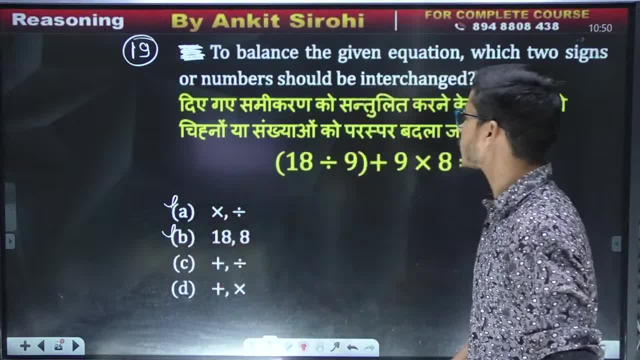 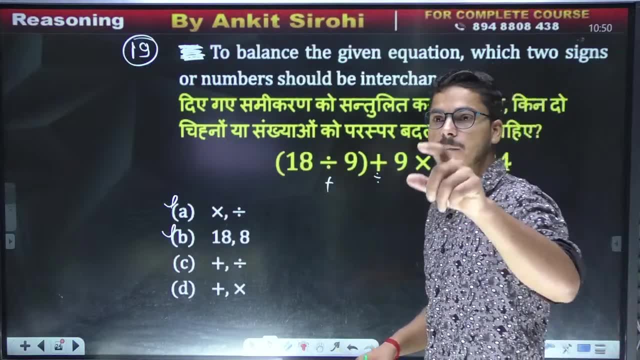 then if you do 8 here and 18 here, then 18 is sitting here more. So if you change the place of the part to the place of the part, then the first one will be 16.. So 18 and 9 will be like: 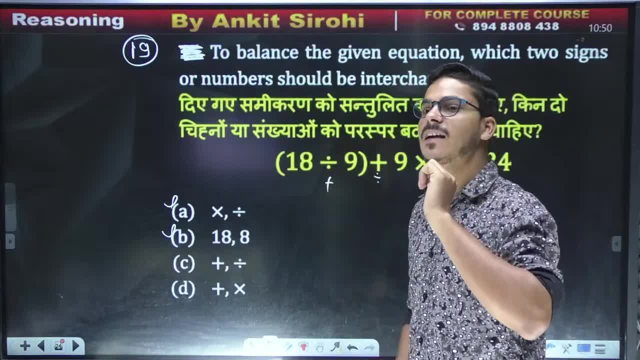 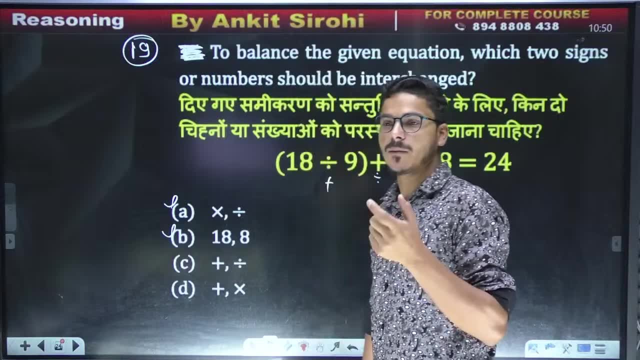 my dear friends, I saw that it is A. Don't worry, my dear friends, I saw that it is A. If you all think that you are not taking the name, then it is not like that. You all know that I will take the name again and again. 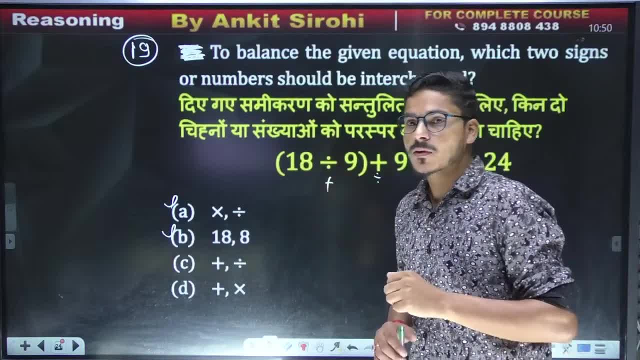 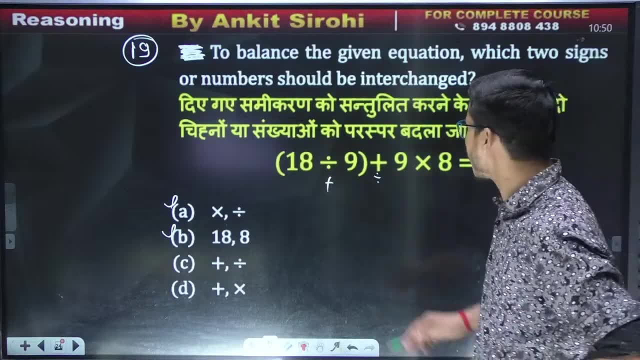 So the number of the question will be less in the numbers. So that's why I try not to take the name and ask quickly. After this there will be one more question. Now I will do it here. So 18 and 9 is 27,. my dear friends, 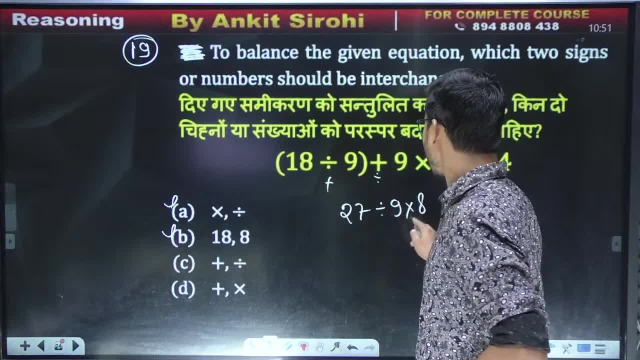 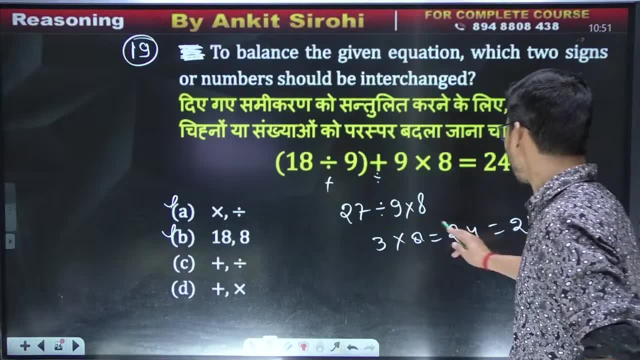 My 9 will be a part: 9 divided by 9, multiplied by 8.. Now let's do it. 9 is 27 multiplied by 8, equal to 24.. So 24 is equal to 24.. It has been proved by this. 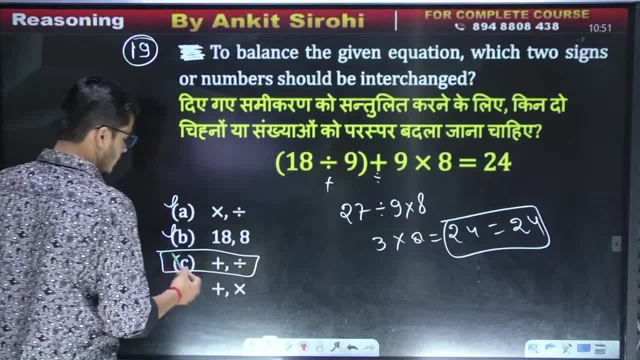 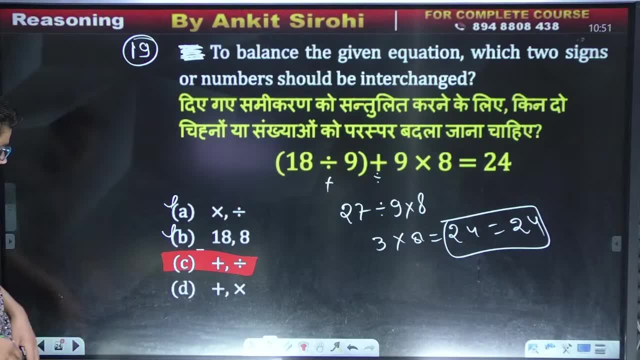 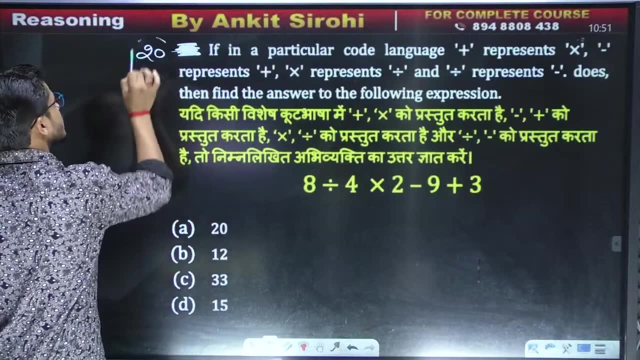 Option number 3 was to change the part and the plus together. Let's change it. Change the part and the plus together. Now it is the last question, My dear friends. it is the last question, 20.. It is the last question. 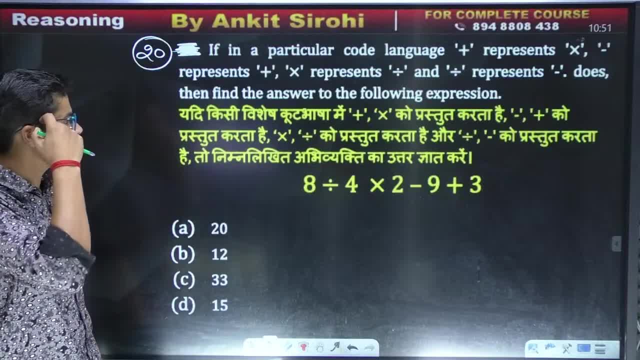 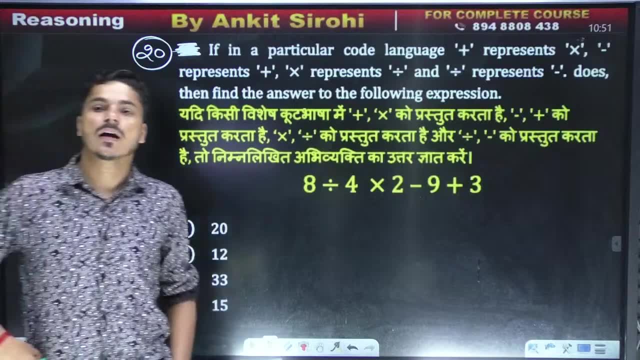 Please answer it. well. What is the answer? There is nothing. What can be an easier question than this? Ali Rashaad was very good. Arsad Ali was also very good. What is the better question than this? It is a simple question. 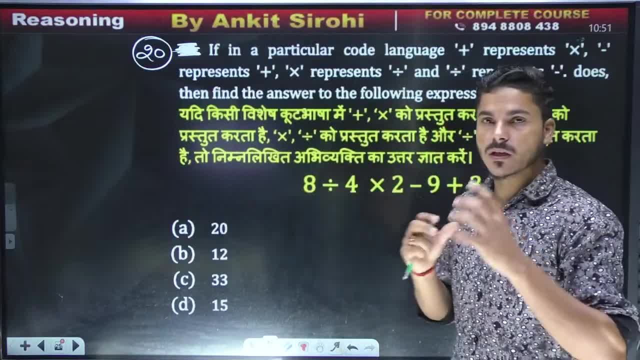 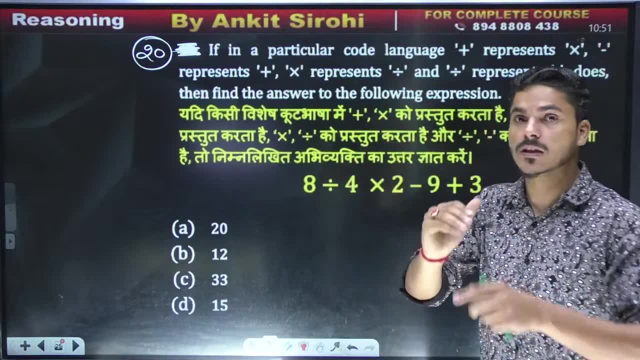 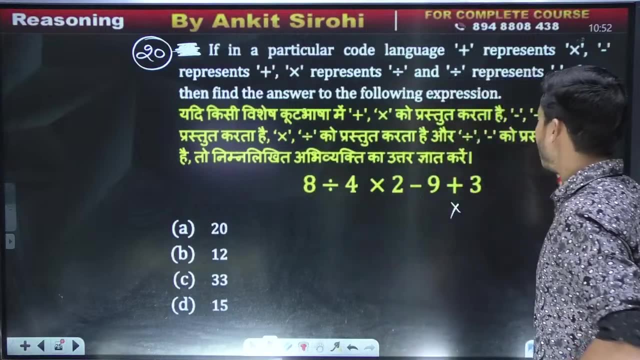 The equation that we have seen in front of us should not be used. Why not? Because, my dear friends, some conditions have been given here. Every sign means another. The plus represents the quantity. So what will it mean? It will be multiplied. 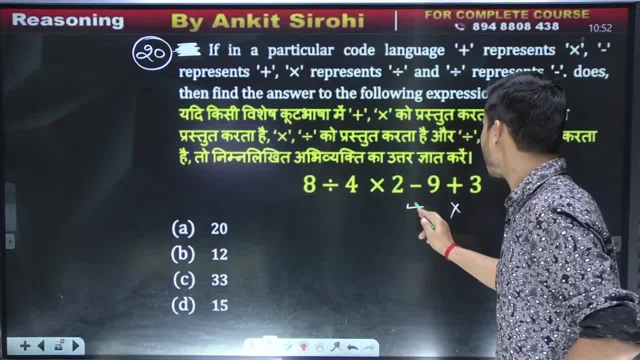 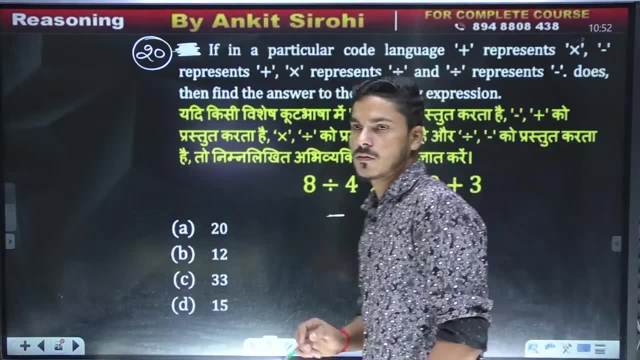 And the minus will be added to the plus. What will happen? It will be added And the multiplied will be divided, And the divided will be minus. Here is your answer. So, dear friends, what is the answer of Mr Kambia? 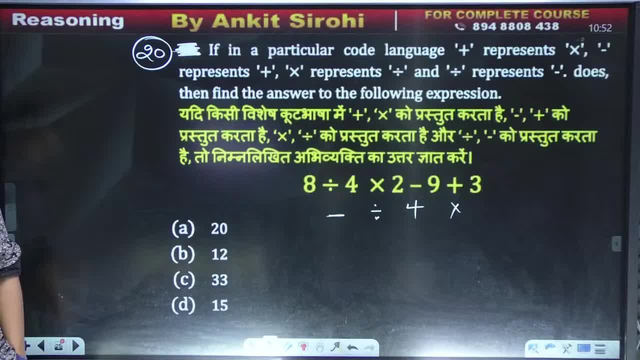 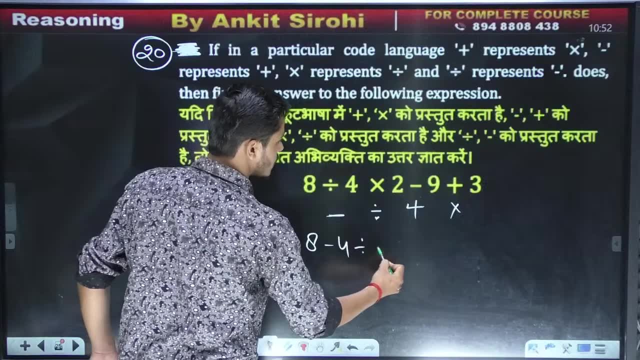 Mr Kambia's answer is 33.. The correct answer is 33.. Let's see. First of all, I have to divide 8 minus 4 by 2.. Okay, Plus 9 and multiplied by 3.. First of all.